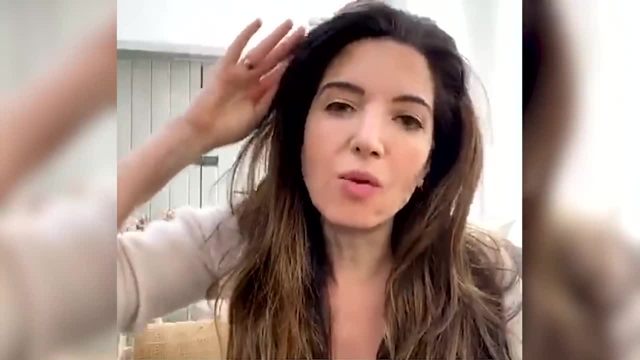 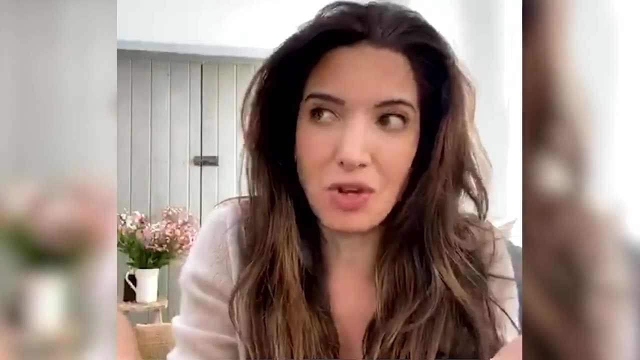 going to talk about writing. Tell me what's been happening with you, Like tell us a little bit about your history in terms of writing, Like where did your writing start? Who were you writing for, let's say, you know, 10-15 years ago? What would that look like? Yeah, well, I started my writing. 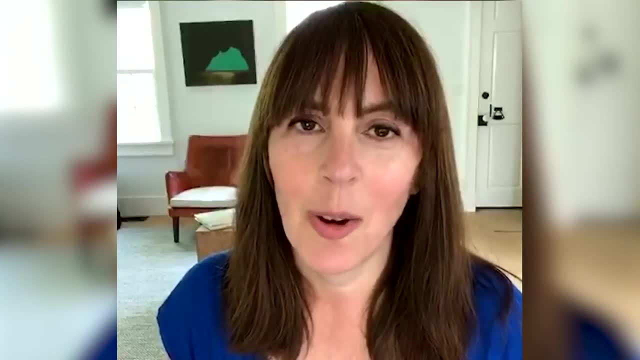 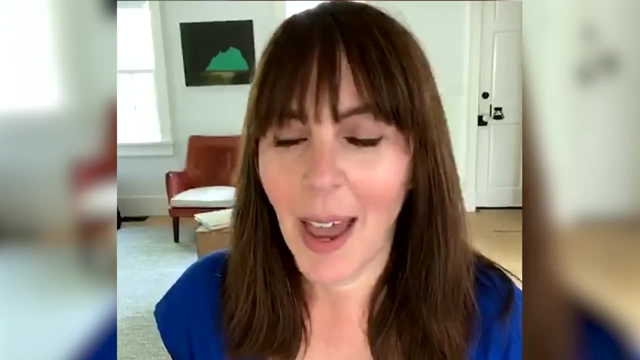 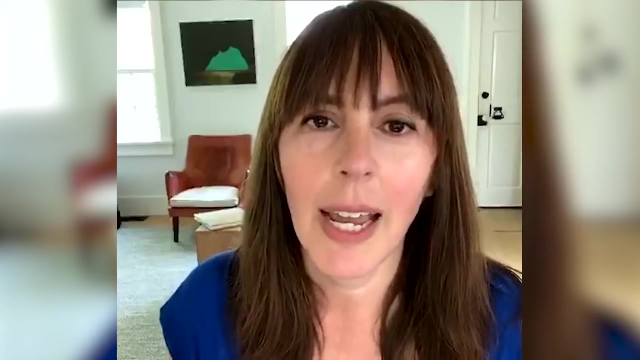 career. first of all, I always knew I wanted to do something with writing, but I didn't know what and I was scared. I was so scared coming out of like college and in my early years after college when I was sleeping till noon and eating corn flakes in front of the TV because I had no idea what I 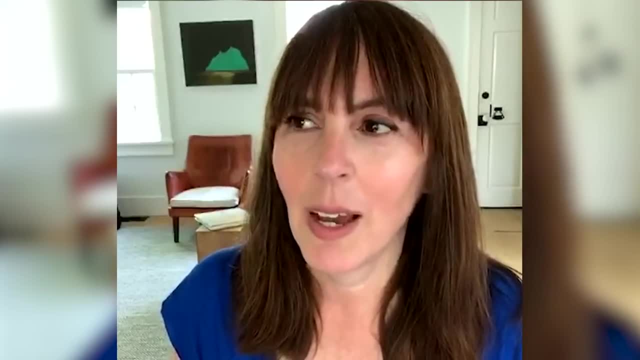 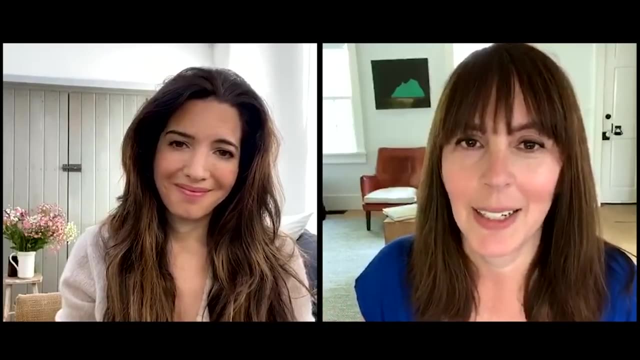 could do with my writing. that wasn't like. I was like I don't think I have a novel in me, So that was one. I was like that's, that seems like too much and I'll be sitting in an attic, you know, with a beret on weeping. and then I was like I don't, I don't want to be a journalist. that wasn't. 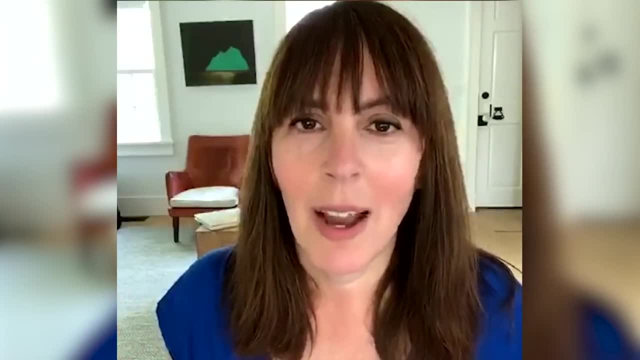 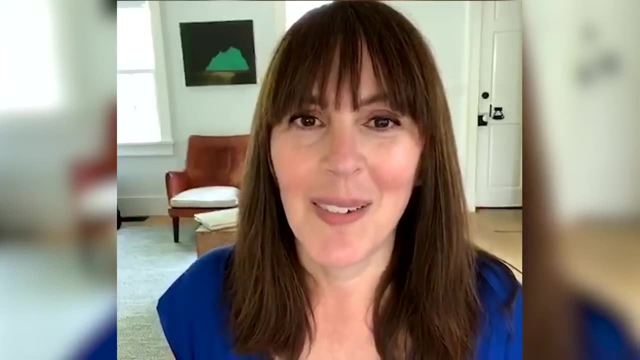 my kind of writing and like everything seemed like too much and not what I had in me, and so I was so scared that I wanted to write and I just couldn't see what I was doing. I was so scared to remember that there was this thing called TV promos, which were writing little things like: 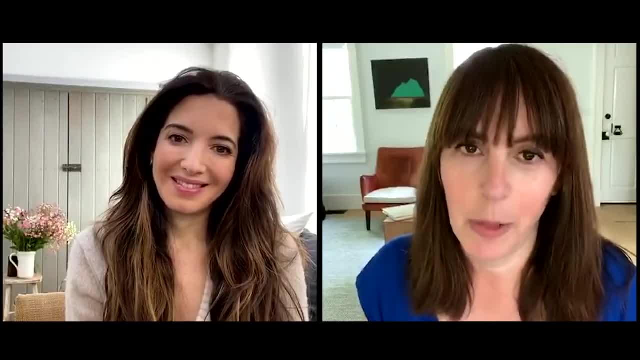 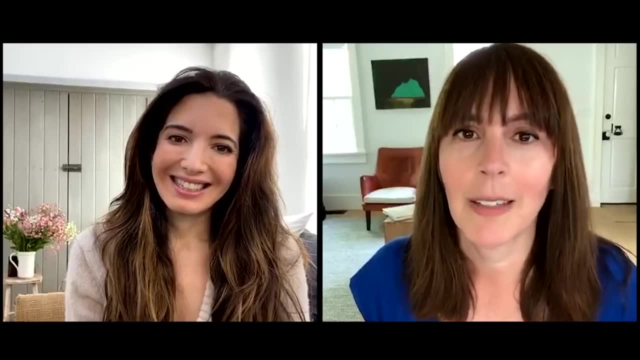 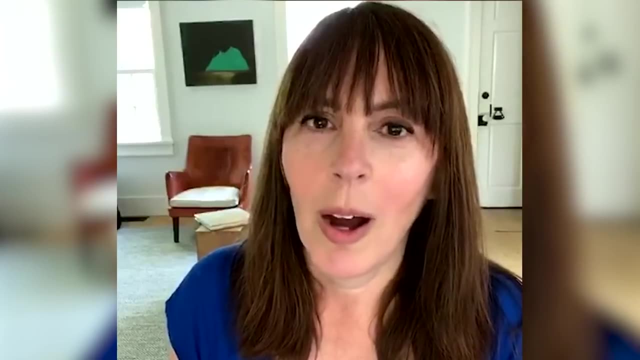 little messages from the network to advertise their own shows. because I loved watching TV and I loved writing little things, So I started off by doing that for many, many years, writing for networks like Nickelodeon, Nick at Night TV, Land, HBO, all kinds of networks- and after a while- and 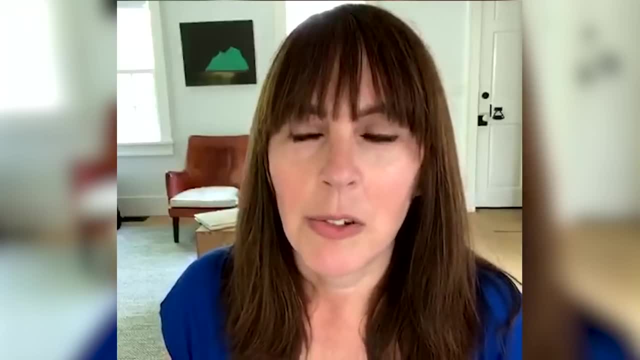 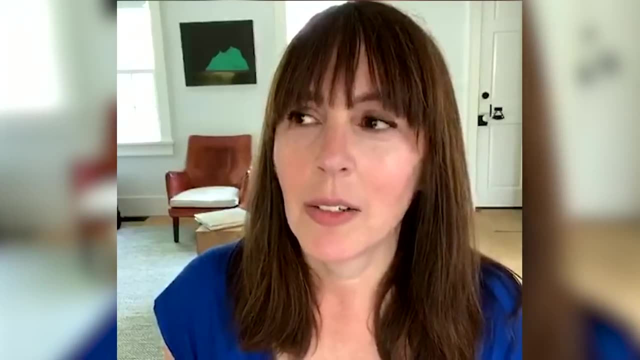 Yes, you knew me at this point. Yes, grunt, because I loved what I was doing, but it was a little bit of been there, done that, And I also I knew I had more to say And I remember sometimes, you know, often I was able to put my 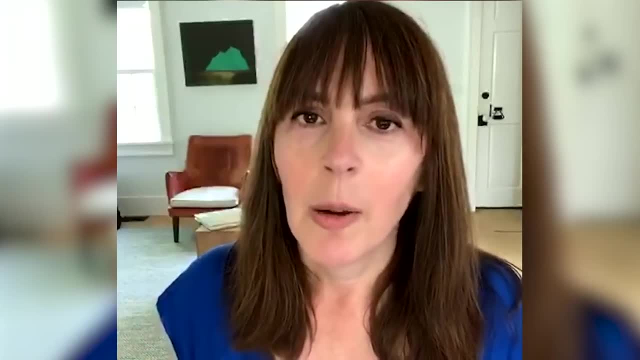 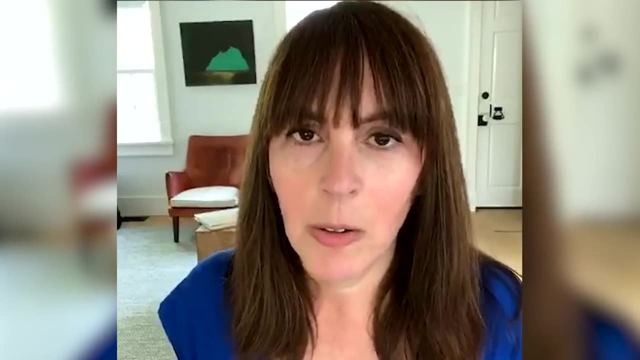 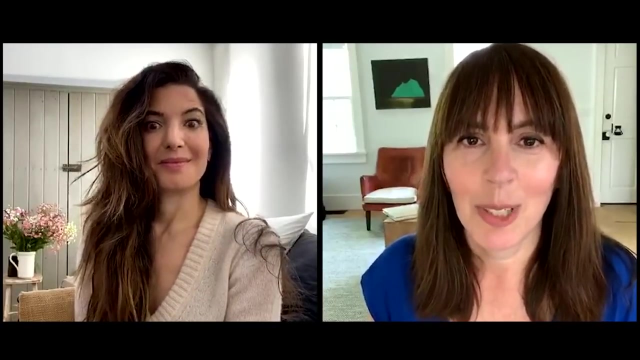 own voice into that and my own point of view. But I remember reading one script out loud at a writer's meeting and my boss said, what is this? the Laura Belgray show? And yeah, and I was like, oh, I guess I can't put so much meat into it And I felt really frustrated at that point I was. 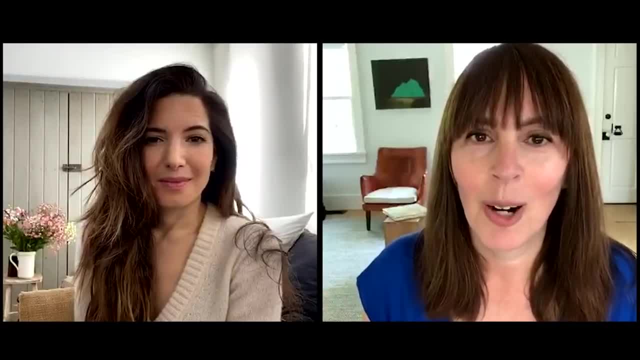 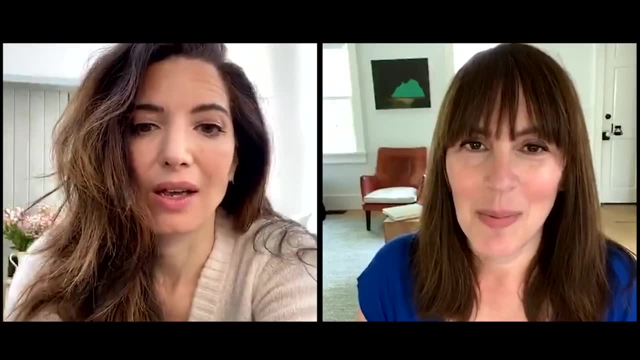 like I have more to say, but I don't know what and I don't know in what form. And so it was kind of a miracle that I was friends with you And you said to me- and I was creating a website to get- 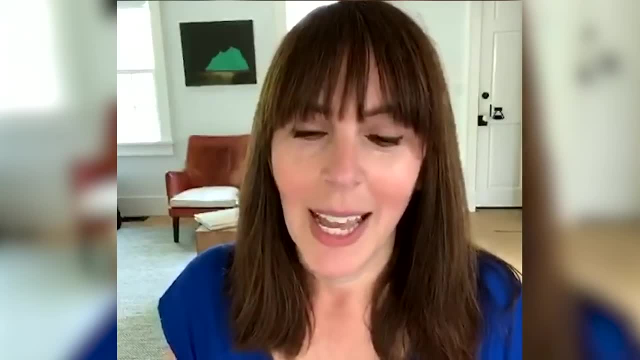 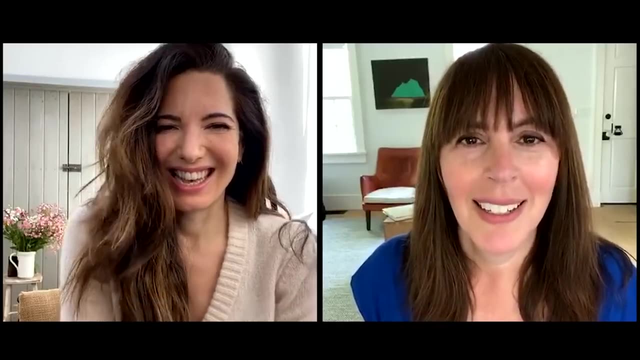 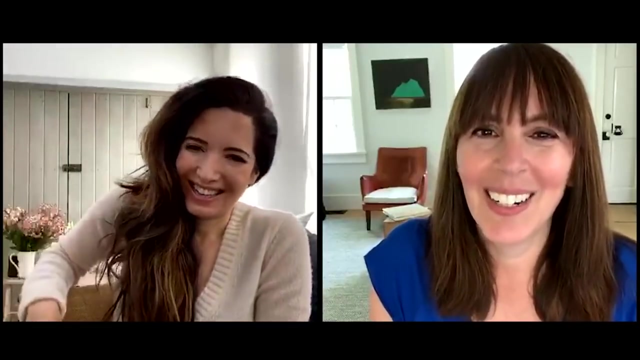 more TV clients, even though I wasn't sure that was what I wanted. And you said to me: you're going to put a blog on your website, right? And I was like, isn't it too late to have a blog? And this was in 2009.. And you were like, no, you moron. I don't think you called me a moron, But 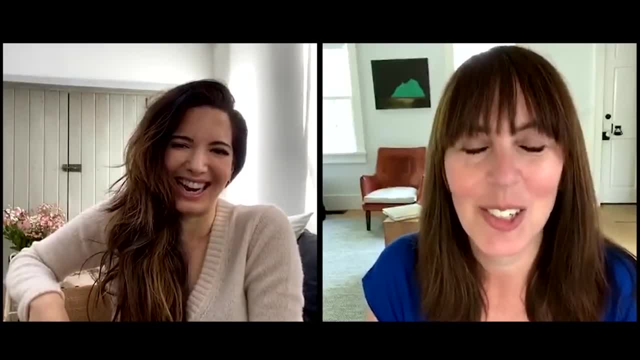 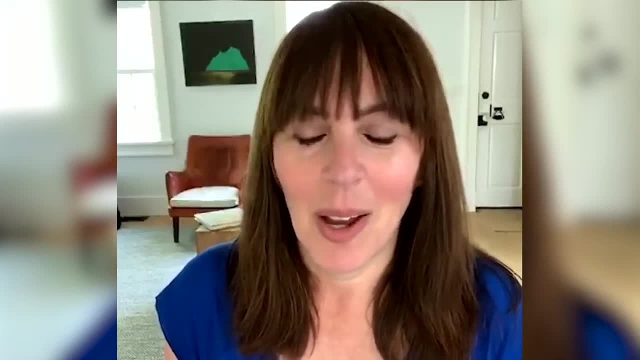 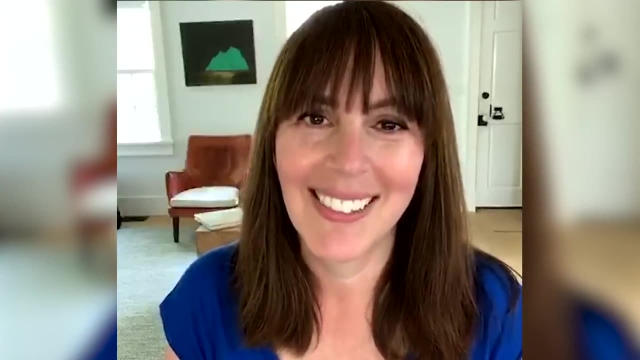 that was the gist of it And, yeah, that was the energy, And I appreciated that, And so you convinced me to start a blog, And you convinced me to also have an opt in on my site to build an audience, to build a list of people who would appreciate my blog, And that's and that's how I 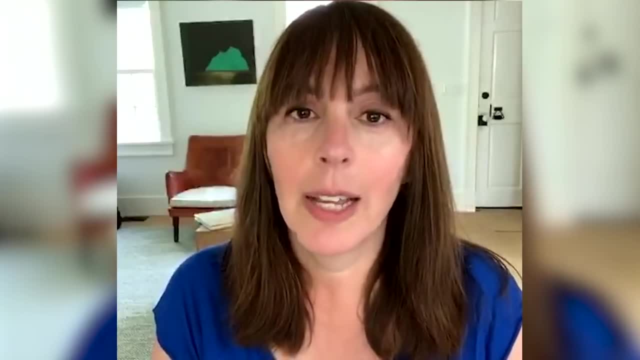 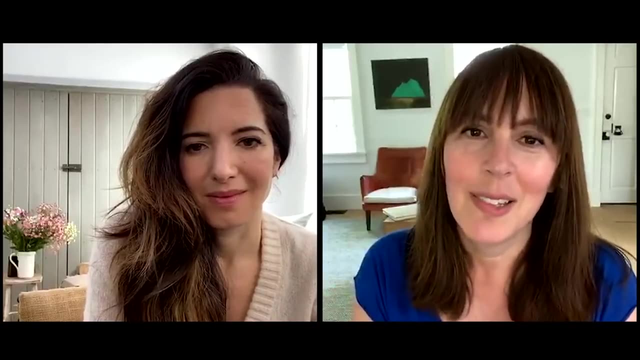 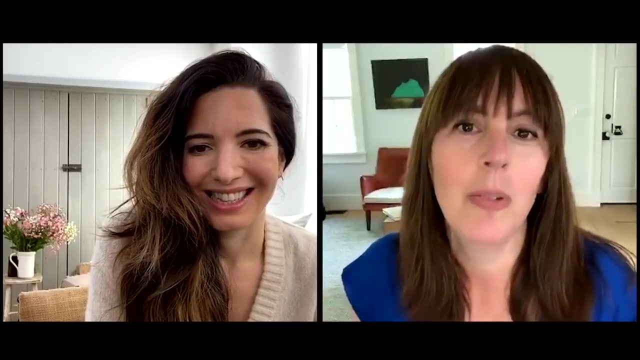 started weaving And then I started taking on private clients in the entrepreneur world and writing emails to them, And that's how I started weaving my own voice into what I do for a living, And it is like a miracle to me that I get to do that. I get to write my own stuff and get paid, So that's That's where I 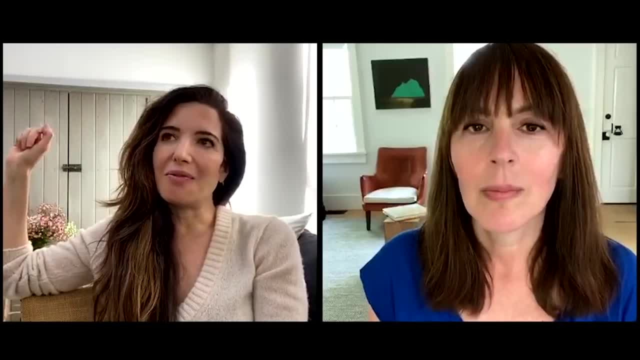 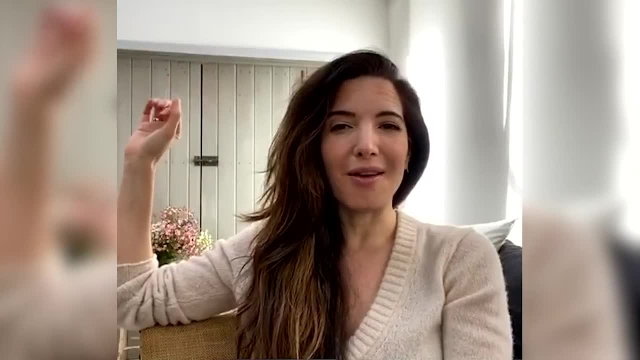 am now Amber Eichner. Yes, that is amazing. I love that story And I love the fact I don't think I ever knew that you kind of got squashed when you put a little bit of yourself. i don't think i ever heard that detail. 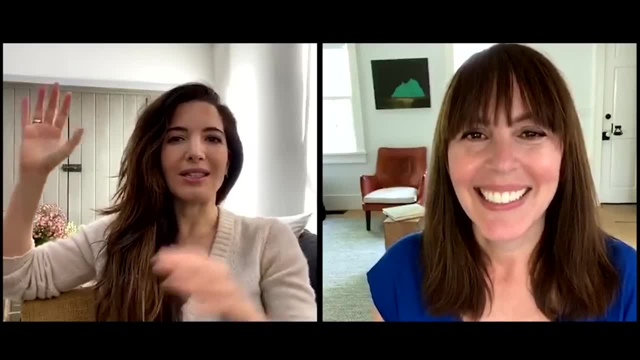 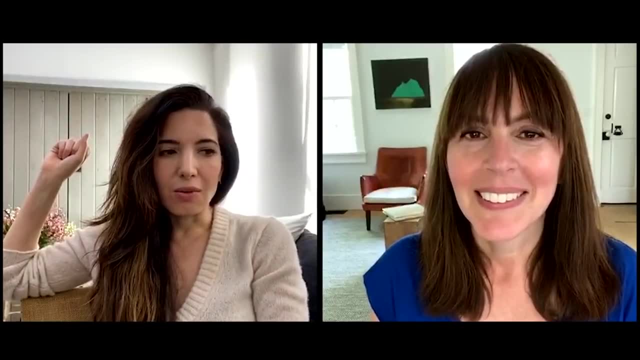 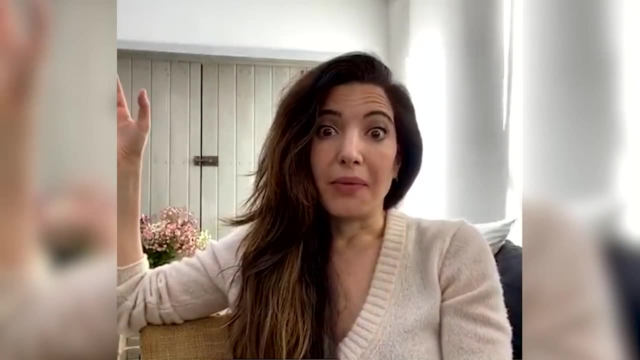 before. that's so interesting. yeah, our voices get tamped down, um by experiences and all of a sudden we get scared to express ourselves. or, you know, especially now. i think it's in the age of social media and in the age of where everybody won't get offended about something in a hot second. 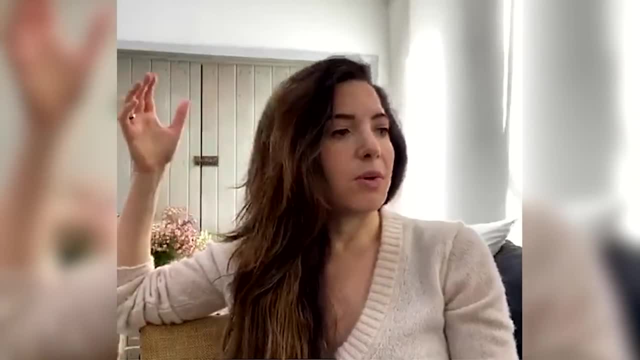 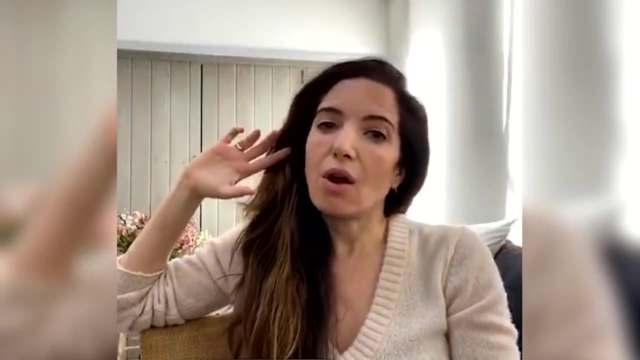 and, yes, are you a new one? it's understandable that people are like: gosh, what is my voice? how do i find my voice? how do i express myself so i don't sound like a carbon copy of everyone else? i'll tell you this. you know we're working on some new stuff in my company and in my business. 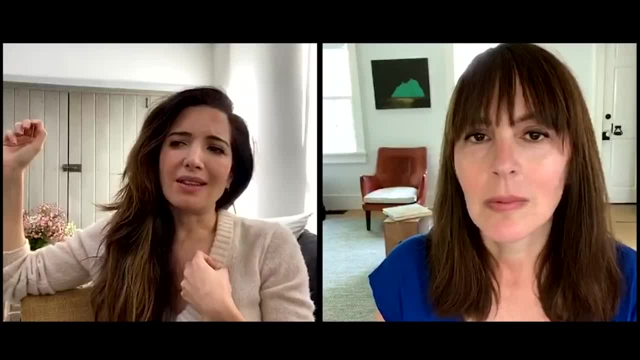 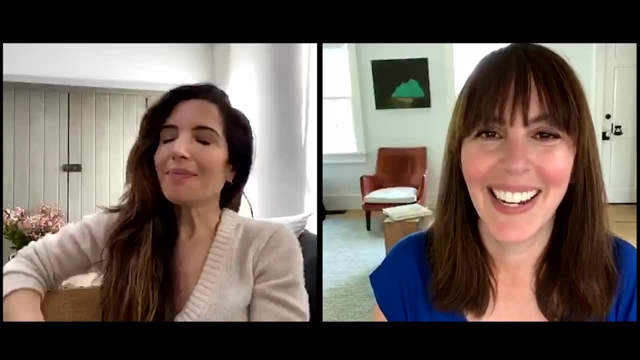 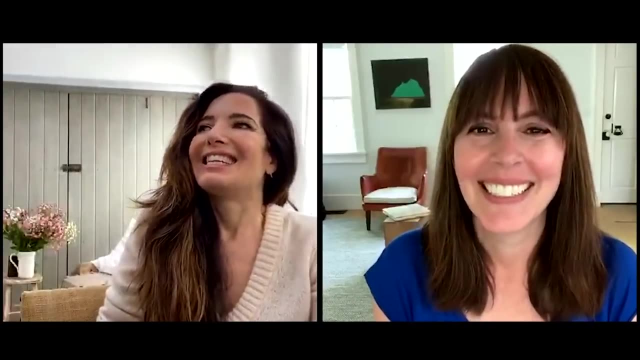 and um, you know me as a human that i'm kind of heads down right. sometimes you will ask me, you'll call me, you'll be like, oh, did you hear about so-and-so? yeah and no, i look, i don't pay attention to you, to those people. i don't pay attention to those people. no, and uh, the reason i'm telling you this: 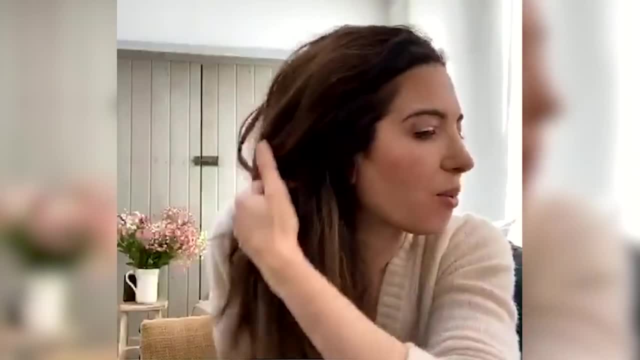 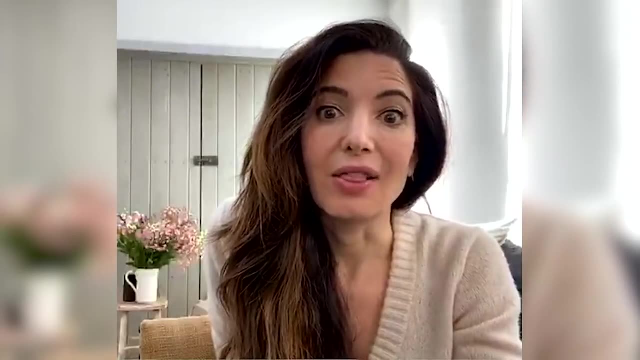 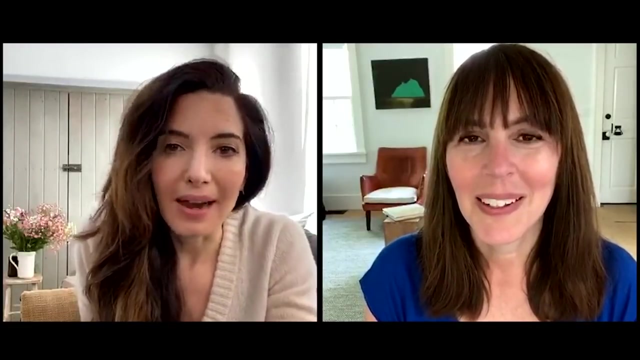 is because my team put together like a whole kind of presentation for me and they're like: oh, my god, do you want to see how many people copy? use your voice and i? it was like slides and slides of slides of all the stuff that we've been saying for years, and and i'm not mad at it, it was just 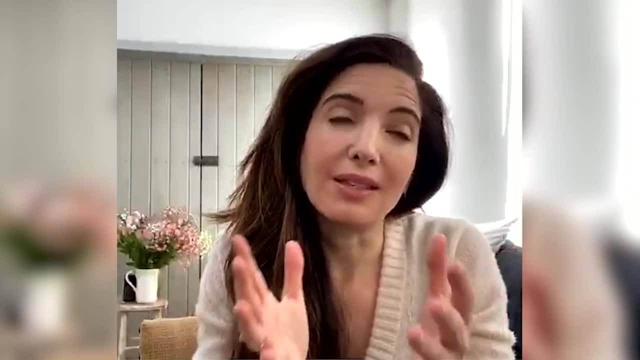 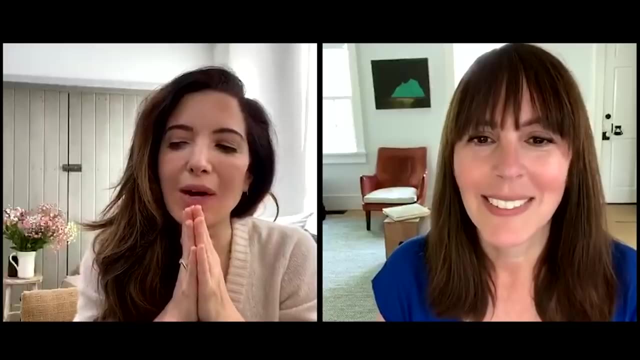 hilarious. but my point is is that i think people get scared and they try and copy someone else's voice because they don't know what their own is. so i'm curious: what's your, what is your perspective on just finding one's voice? you know what i mean if you're like, if 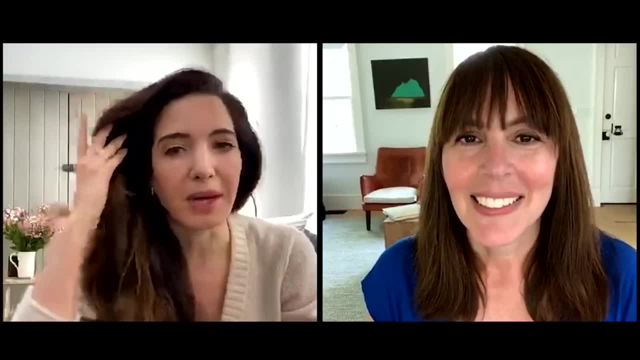 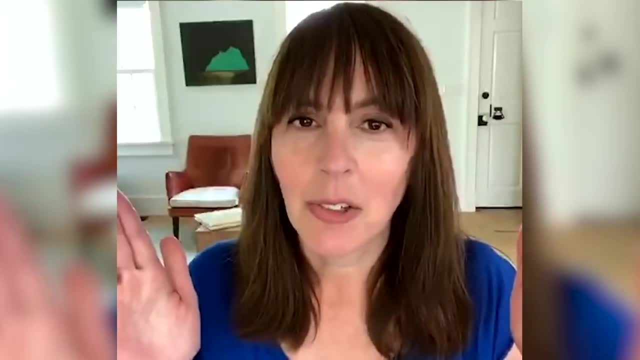 someone watching right now is insecure. how do they start to find their voice on the page? yeah, that well, you weren't saying it to relate to this, but when you were talking about keeping your blinders on not looking at what everyone else is doing. that is one way that you can. 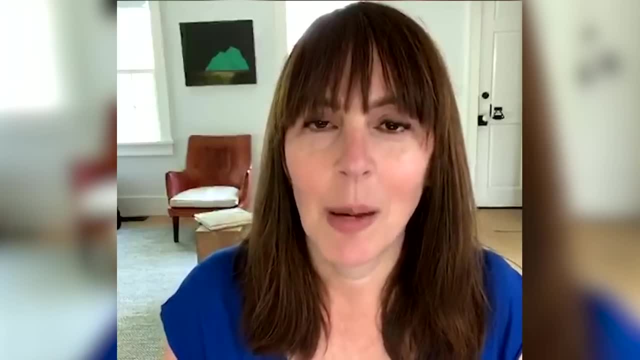 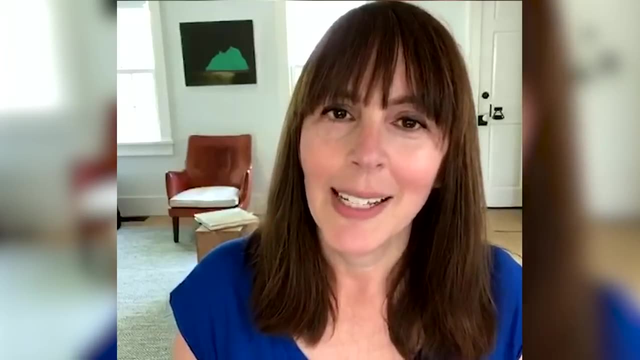 do that. um, you know, if you start to find yourself copying somebody and you're like i'm too influenced by this person, i you know their voice is the voice i want. they said everything the way i want to say it. sometimes it's time to like turn them off, and it doesn't mean you don't like them. 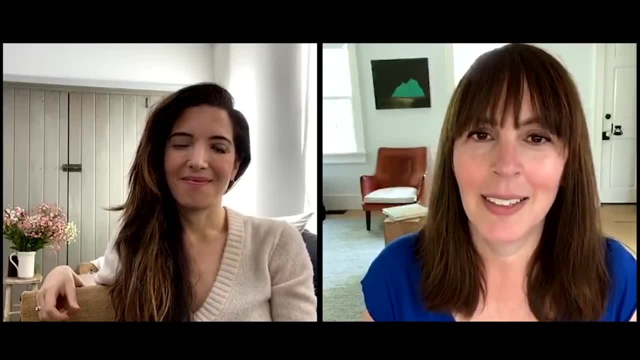 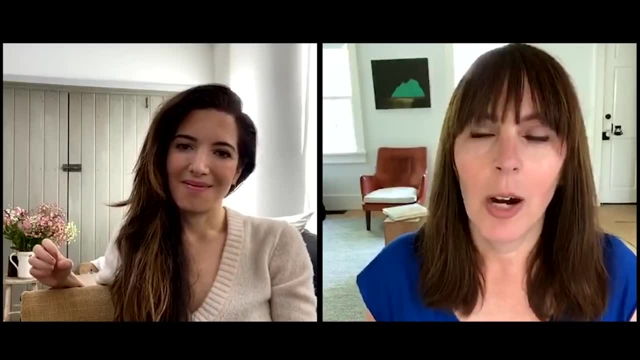 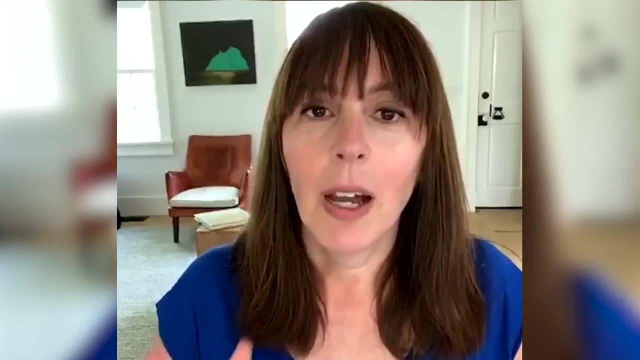 anymore. um, you might want to turn them off for a little bit and stop letting them get in your head like wonderful that you've gotten something from them and now be you. um, and we, we get this notion from watching, like from watching people like you, marie, that you know because you are so authentic. 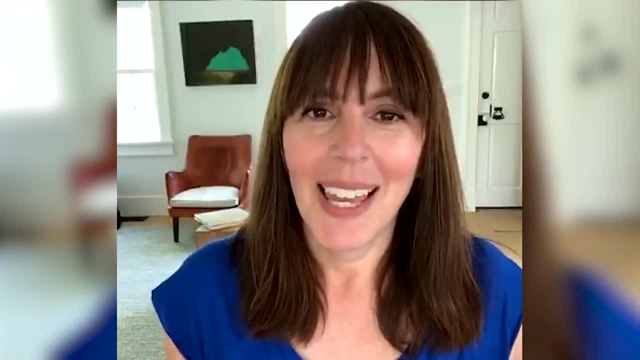 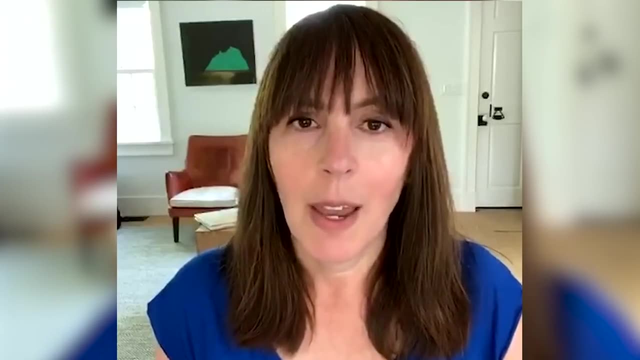 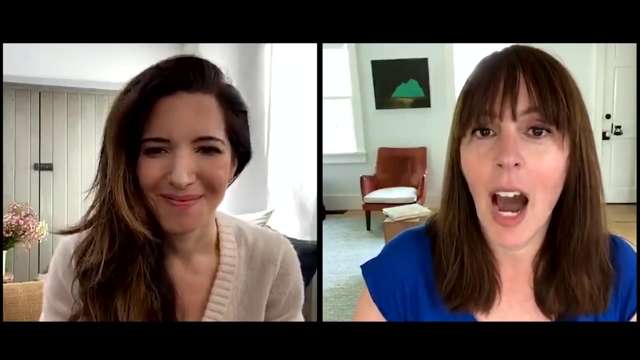 and you come across as so you um, in everything that you do, we get this notion that you are what it means to be authentic. so, therefore, we have to have your voice in order to be authentic. like, oh, we have to use, like hip hop references and we have to be sassy and say yas, and blow an air horn and and that's like that's. 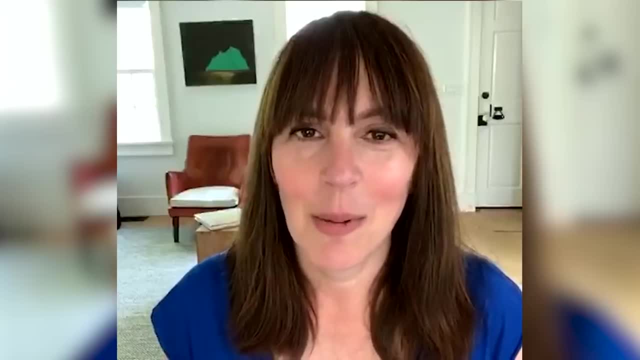 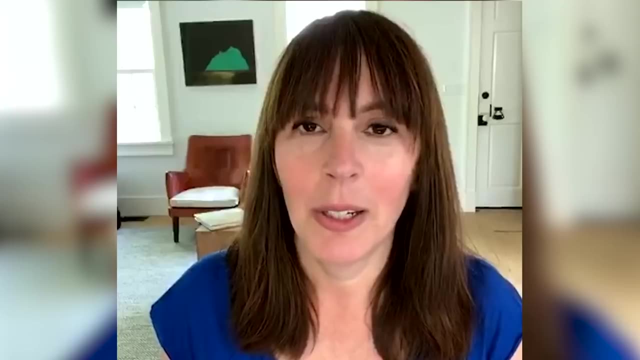 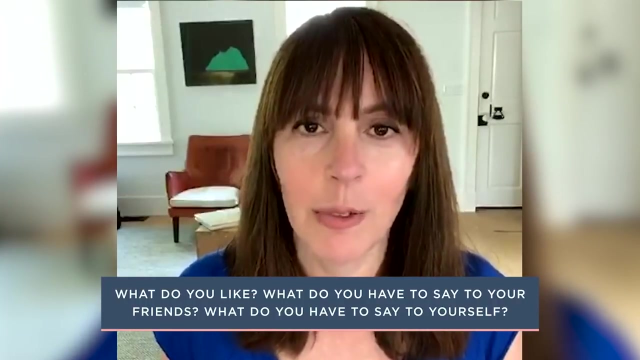 your version of authentic. that is you. that's not someone else's version of authentic. so i think um the way to find your voice and be more you is, first of all, think about what do you like? what do you have to say to your friends? what do you have to say to yourself? you know what your voice is. 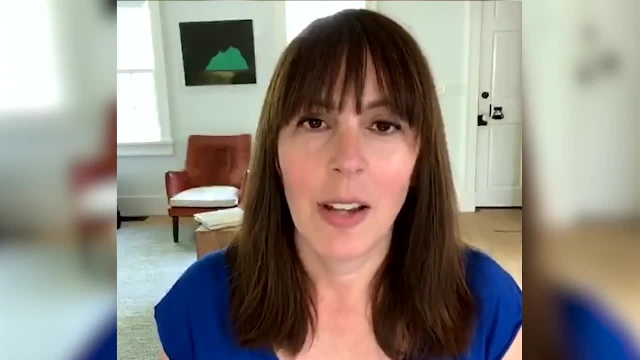 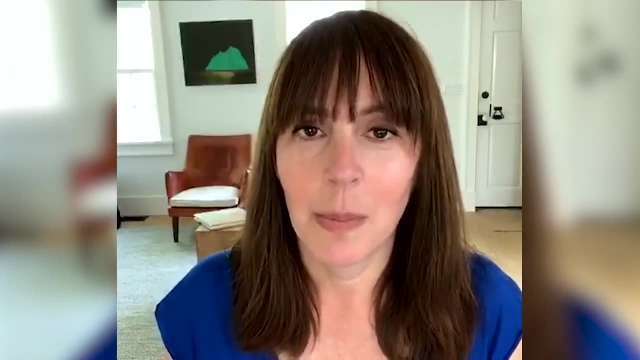 about what you have to say, not what somebody else said. so, um, you know we're talking about writing. i think writing for yourself, for starters, is a great way to find your voice, because writing without, without the intention of somebody else reading it or hearing it, or being an audience. 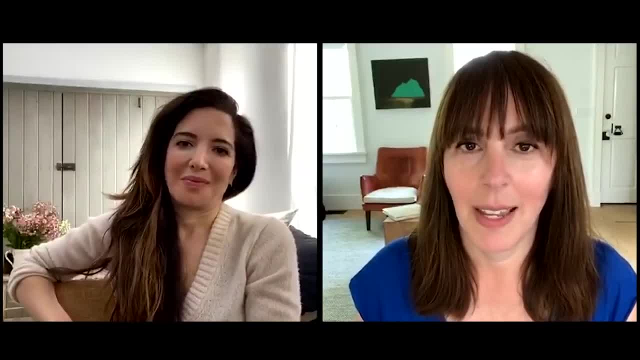 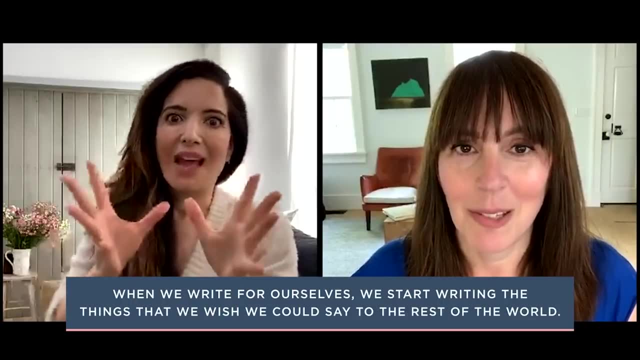 writing for yourself and seeing what comes out and what you have to say, what you want to say. often, when we write for ourselves, we start writing the things that we wish we could say to the rest of the world, and let's talk about that. let's talk about that because, um, you know. 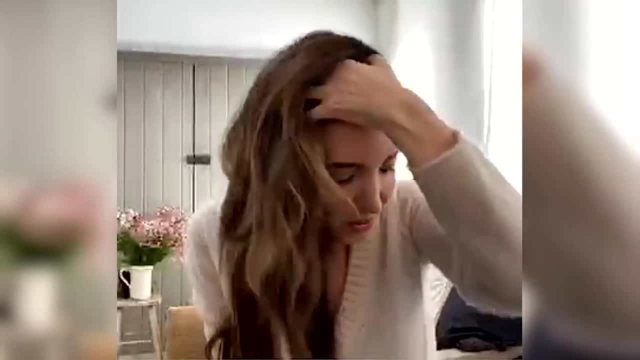 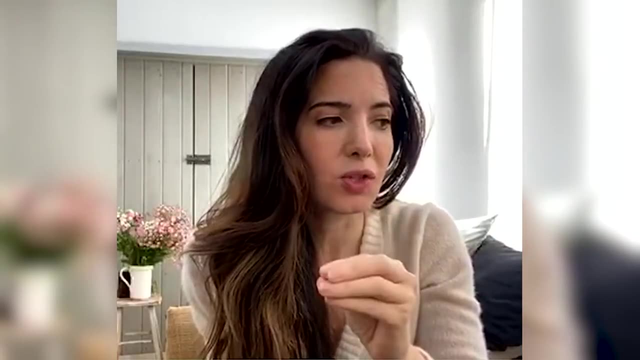 one of my favorite things that we have in the copy cure and that you and i, um like, created together, was this tip, and i think that it's so perfect for everyone listening right now if you're interested in finding your voice. one of the things that lauren 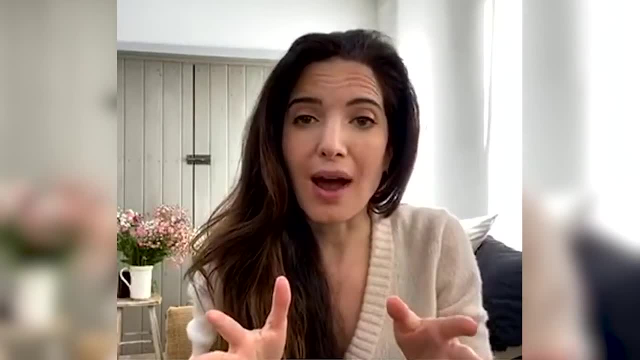 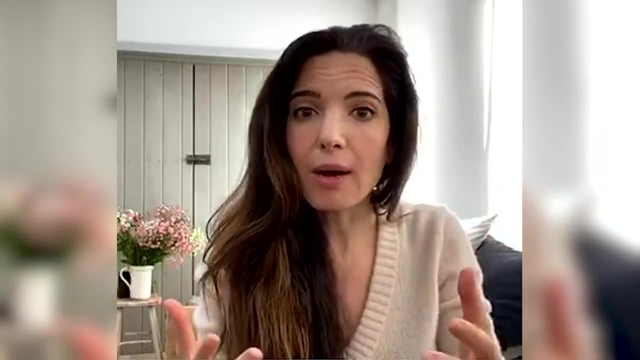 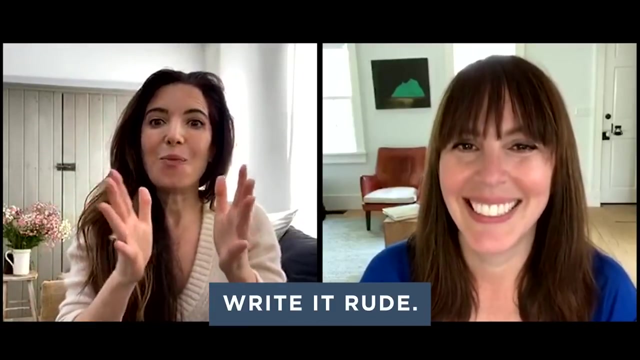 i suggest right is when you're working on your draft, whether it's just in your journal, or you've opened up a new google document and you're working on copy for your website or even a program, or maybe it's a novel or even a how-to non-fiction book- write it rude. so yes, one of my favorite. 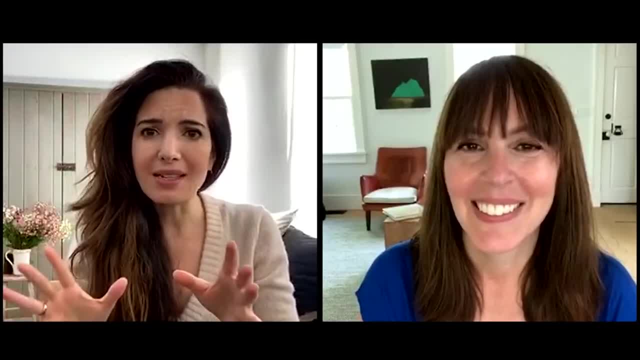 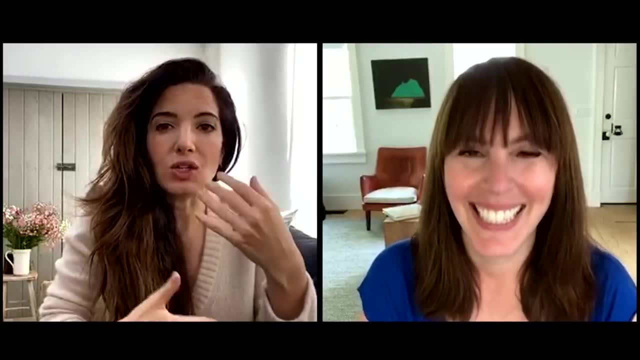 things. so when i practice writing it rude- and there's so many times that i do this and we're going to explain what this means- we're also going to explain that you don't need to leave it rude, but you need to get it right and you need to get it right and you need to get it. 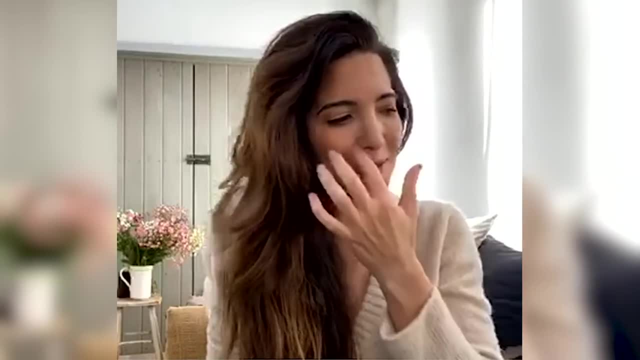 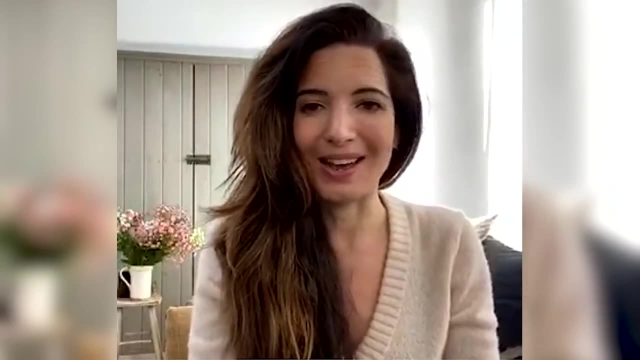 out on the page and i know because laura and i have like written together, we've like been in restaurants and i've had my computer and she's had her thing and we kind of we love playing together and it's like well okay, like laura said to me, like marine, okay, what would you say if you were? 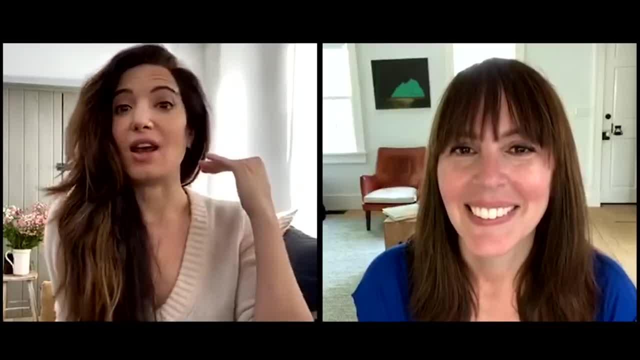 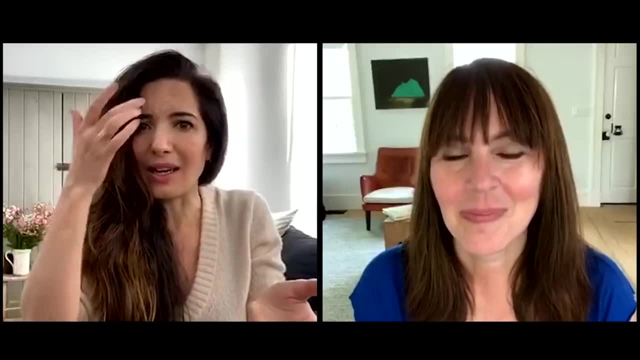 not going to publish this, like just actually say it right to me and i let it rip right, just go for it. and then we're like, okay, we're going to write that down. and then we write it and it literally almost always takes like one or two light edits. 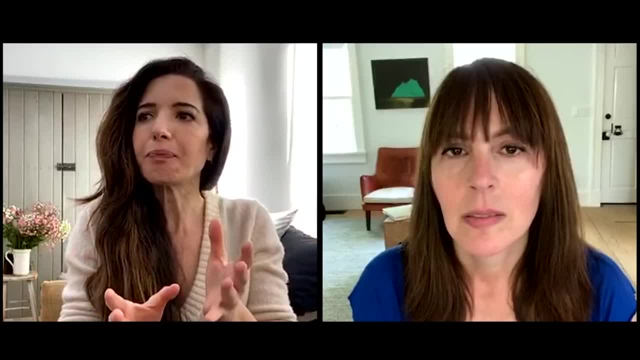 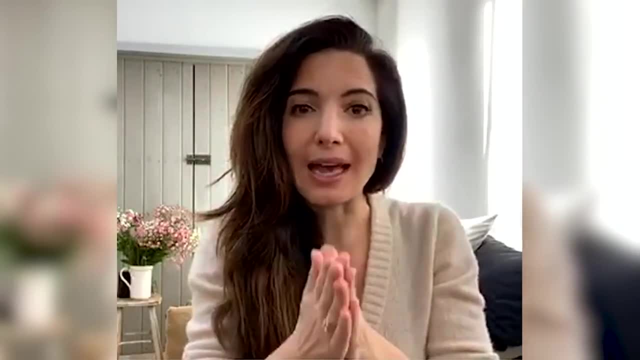 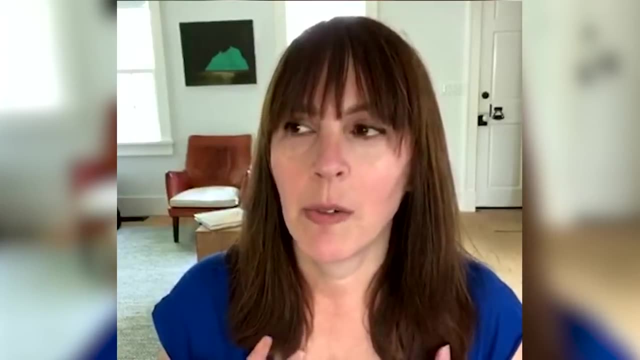 to make it. oh well, how do i reconnect that with my sense of compassion and my sense of honoring all people? but it is so effective for getting to the reality of what you want to say quickly. yeah, because often, i mean, you are first of all, i think, an empath, um, so you really feel, you, i think. 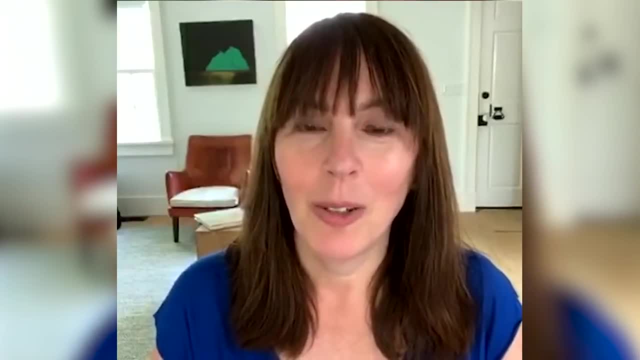 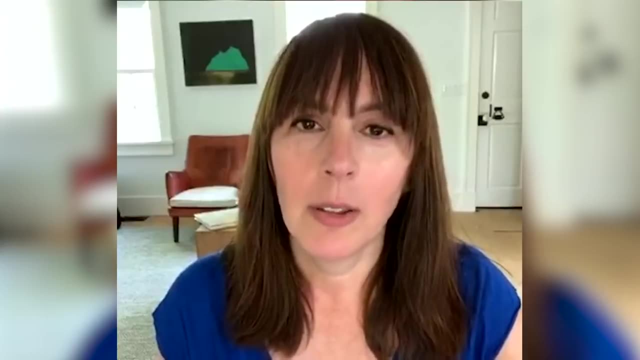 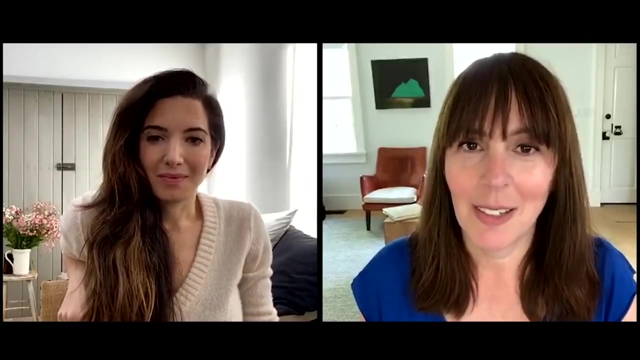 you pre-feel the things that people are thinking when you say something and you're like, i think you like there are ghosts around you that you pick up on that are saying, well, i don't like the way you said that, or well, what about me? you know, this didn't apply to me, and so you tend to get really careful when you're listening to. 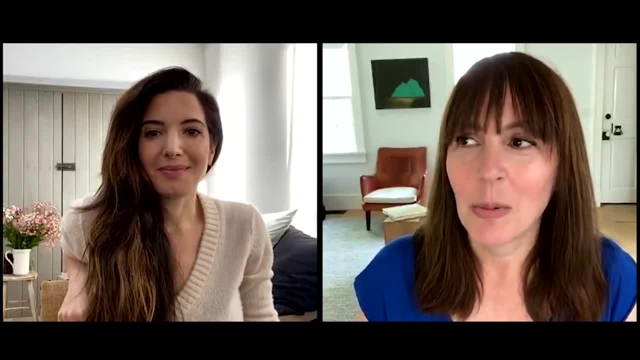 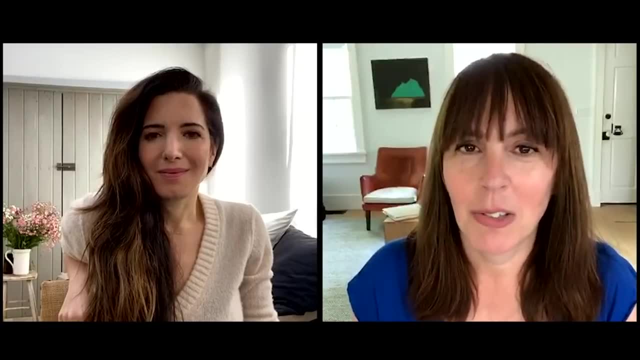 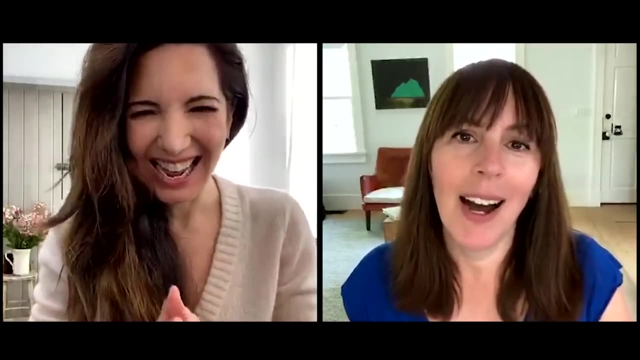 those voices and then often i'll like get you started, but just by with something i said like did you, you know, just as an aside, being distracted while writing, um, did you know so-and-so, said this thing, this route, and you're like what that mother you get when, when you. 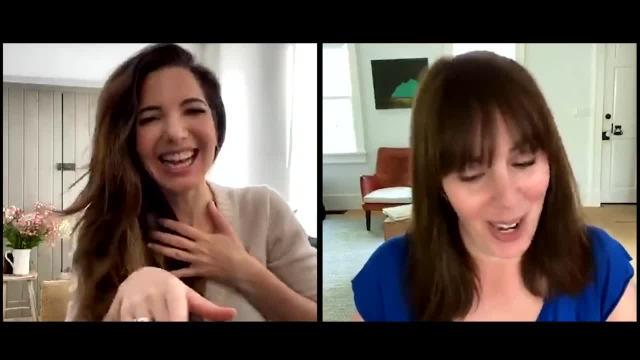 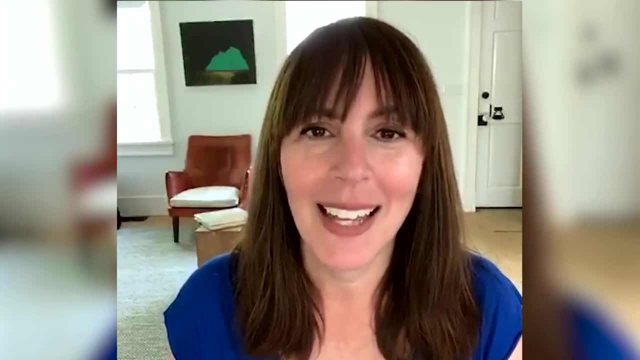 get mad. that's when the gold comes out and i'm like i'm taking out everything you're saying right now. so that's like you went. just let yourself be rude, and that is the best stuff i used to like when i was working with clients. i had a questionnaire that i'd send them in a google. 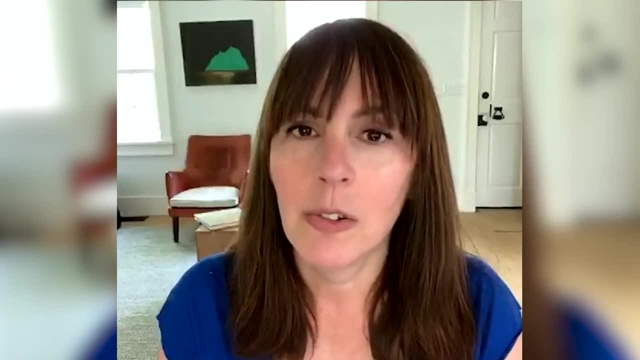 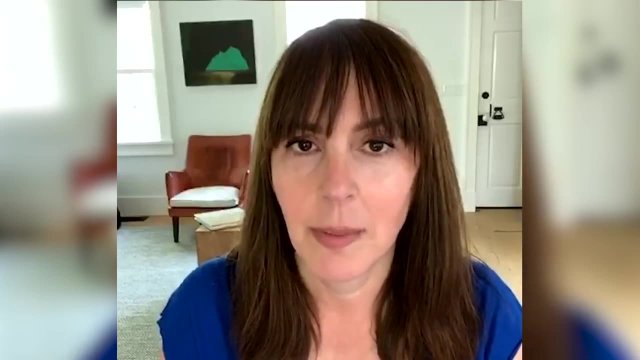 doc, and one of the top questions was: you know, it was like: what do you do? and then the next thing is: what would you say you do if, um, you didn't give a crap what anyone thinks, and that is always the best thing to do, and that's the best thing to do, and that's the best thing to do, and that's the. 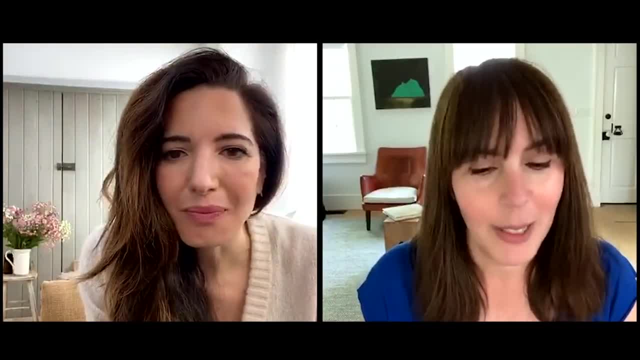 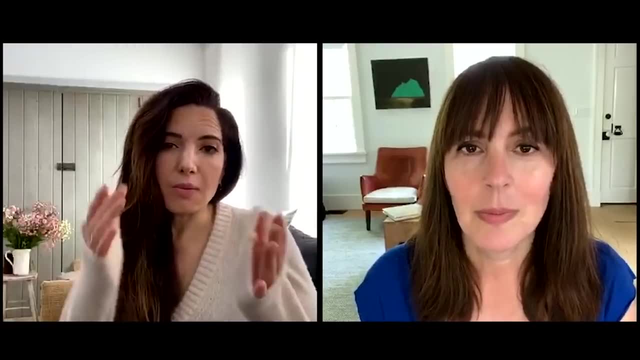 best stuff and that you know, just writing for yourself, thinking, just letting it out and not thinking about that audience. yes, so important it's. i think important too because what we're talking about are stages of writing, you know, and so many people feel a sense of writer's block, or 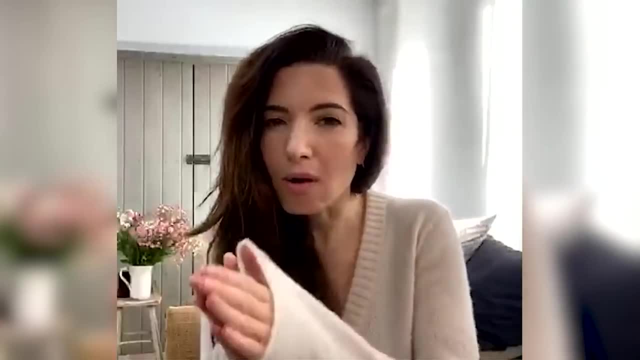 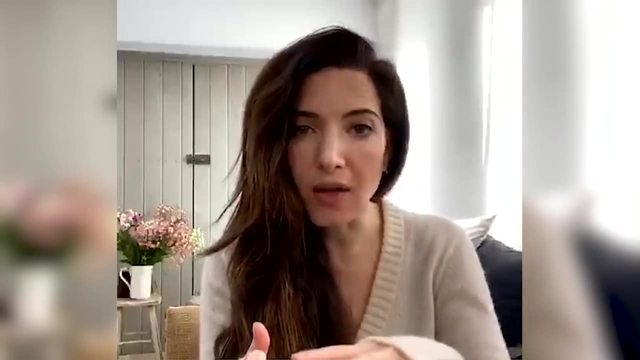 they feel like they don't know what to say, or they don't know how to say it, or they're already jumping kind of to the end product, which might be the finished manuscript, the printed book, the copy that's actually on the website, the copy that you send out in your email they're looking at. 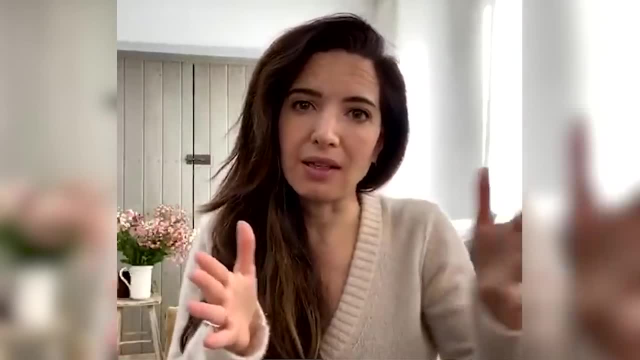 the end product and they're looking at the end product and they're looking at the end product and they're looking at the end and going like how do i get there? not realizing that there are so many steps in between. i think one of the other things that people have to realize especially. 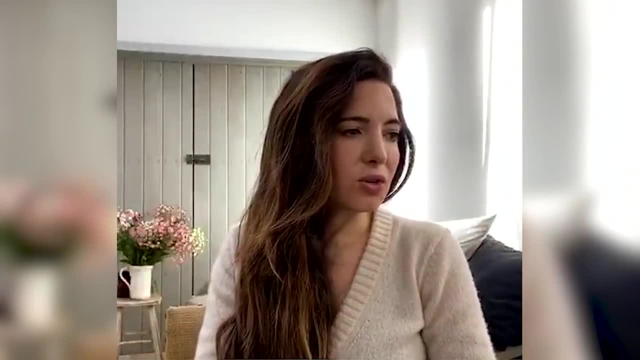 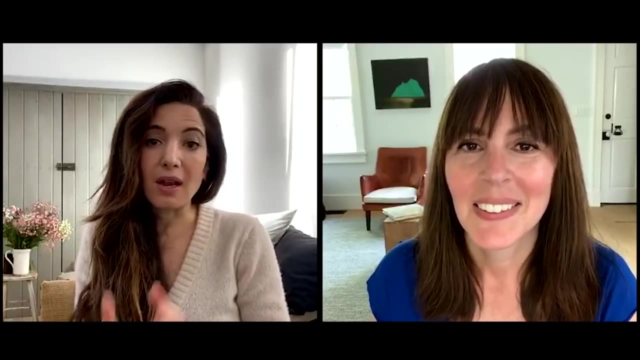 about writing and then i want to kind of shift gears and go into um kind of creative writing and the healing qualities of it and telling stories and stuff. but i think all of us have to realize i'm going through this now because i'm working- actually working on my next book. 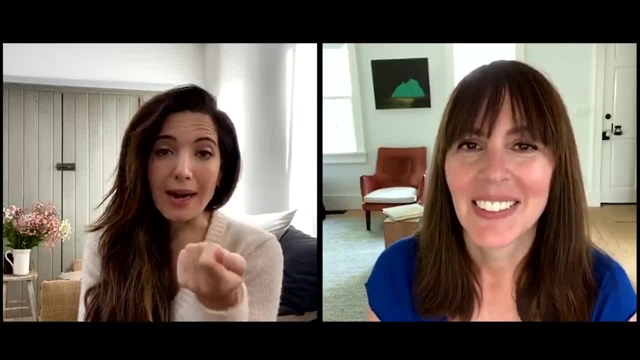 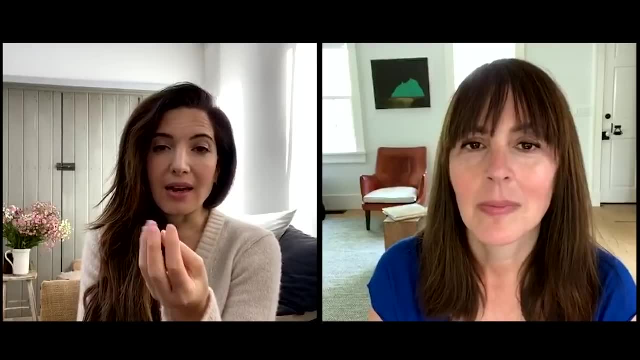 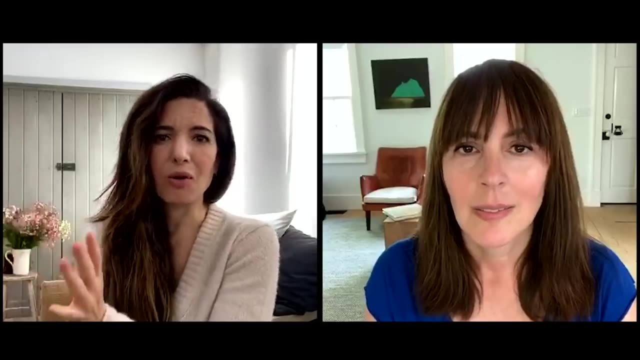 and um. you know? what's great is that i'm close enough in to everything. is figure outable that i have energetic and emotional memory. do you know how, if you get so far away from an experience, you almost either always just remember the good parts or you almost always. 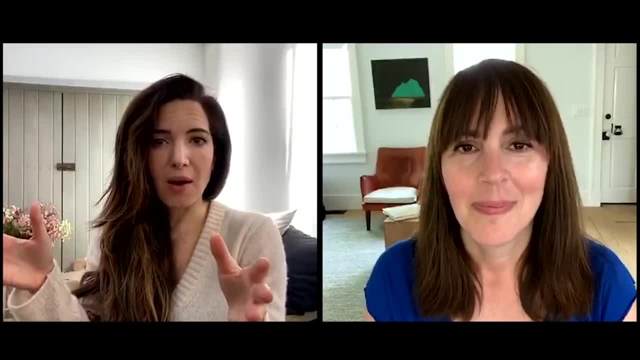 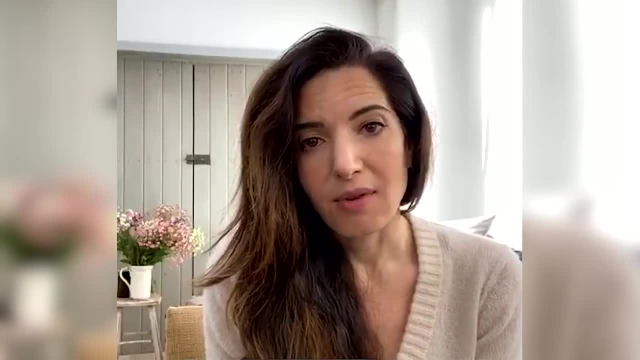 remember the bad parts, but you kind of miss some of the nuance of how it actually went down. and for me, i remember very viscerally wanting to like bang my head against the wall writing. everything is figureoutable- when i was in the messy middle. 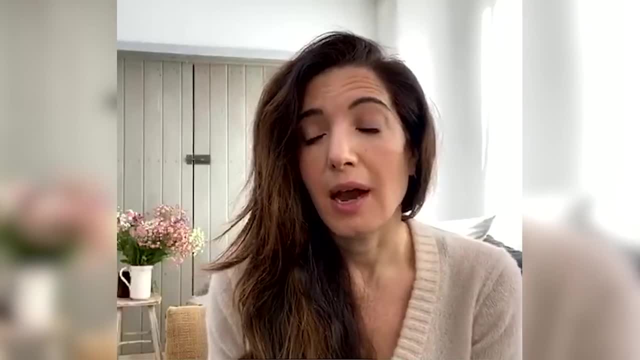 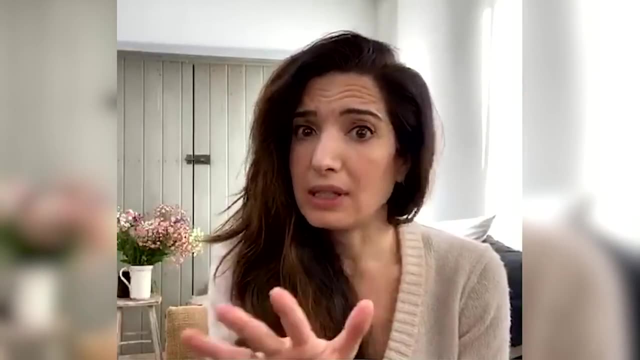 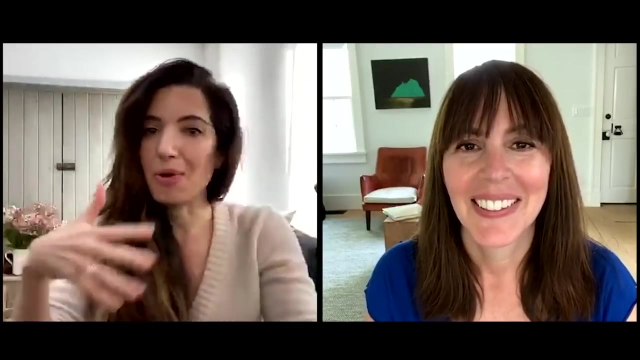 yeah, torturing myself because, and i want to say this, you know, writing marie tv for me, like when i sit down to write, that it's not always easy by any stretch, but i'm not trained to sit down and to write and to complete and to produce, and a book is a very 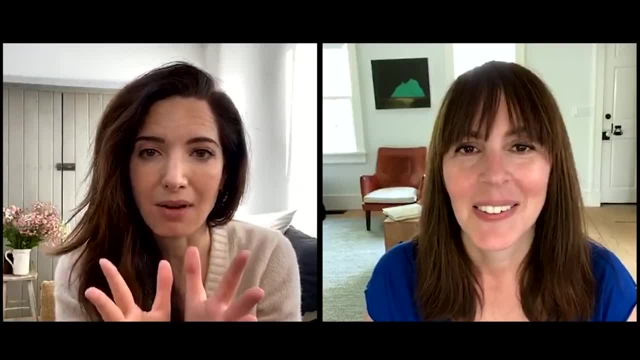 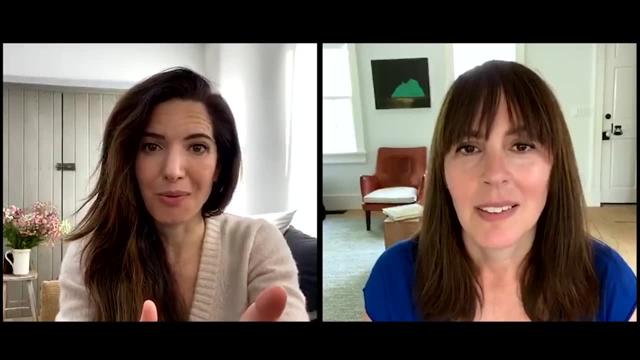 different thing and i think that remembering there is the messy middle and it is so uncomfortable to have uncertainty right when, like all of your material- and i want you to talk about your proposal like- i remember being on the phone with you with the book that you're working on right now- 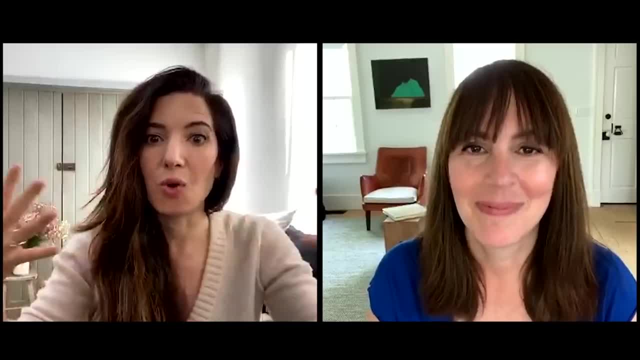 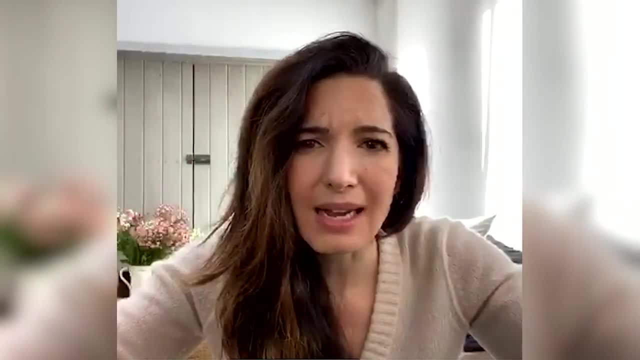 and you're like, marie, i have so much, right, i have so much, i have so much, i have so much. and you're like i don't know if it's a book. is it a book, right? it's just like that's how i felt. i was like, how did i talk about this big idea? and it's messy and it's uncomfortable, but you 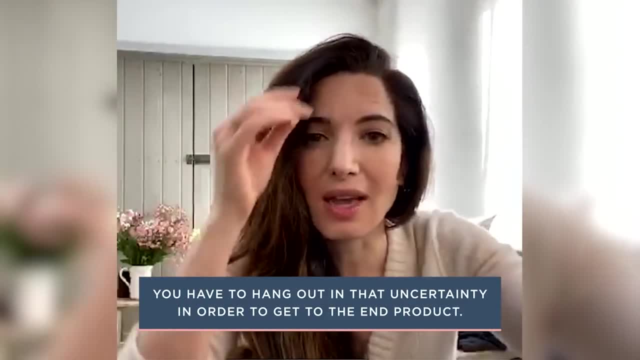 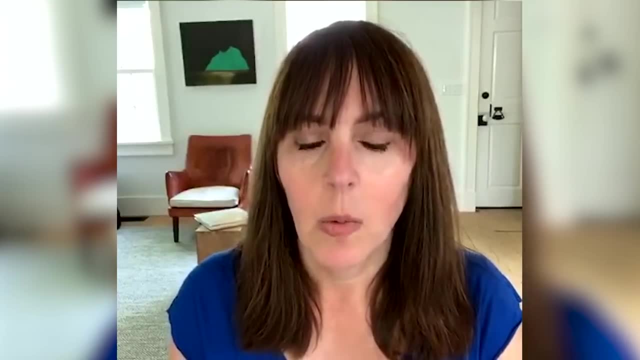 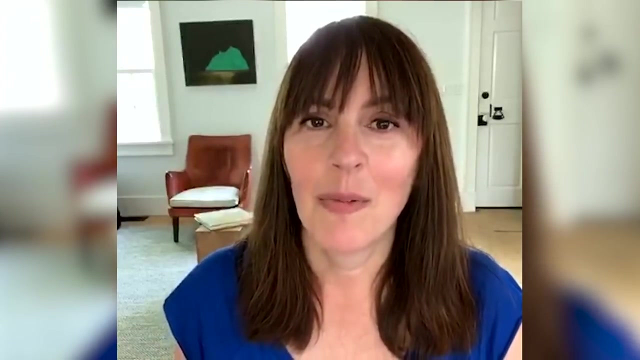 have to hang out in that uncertainty in order to get to the end product, whether it's a website, an email or a book. yes, um, a couple of things about that. one is: yes, i very much feel like i've had, or did have, first book syndrome, fbs. um, feeling like i have to put everything into this. 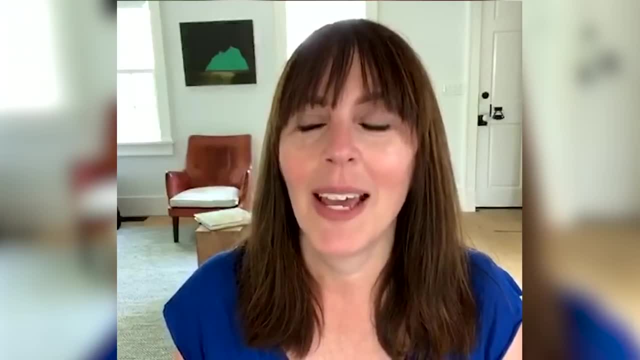 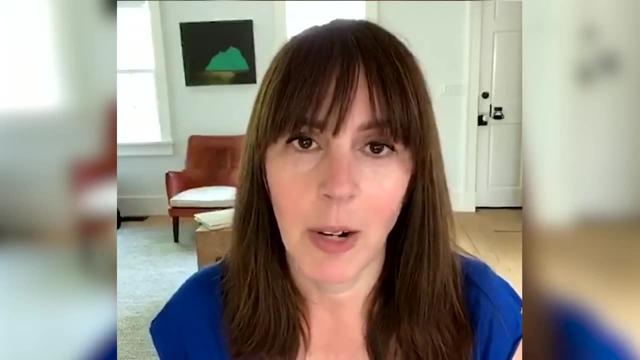 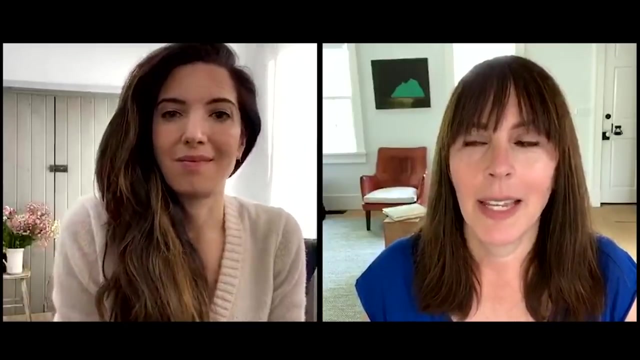 but not everything belongs in it. so what do i do, you know? and i finally trusted myself and trusted the process enough to just start writing, like, write the part that's fun right now, write the thing that that i remember right now. write every story i want to tell, and like it's kind of like 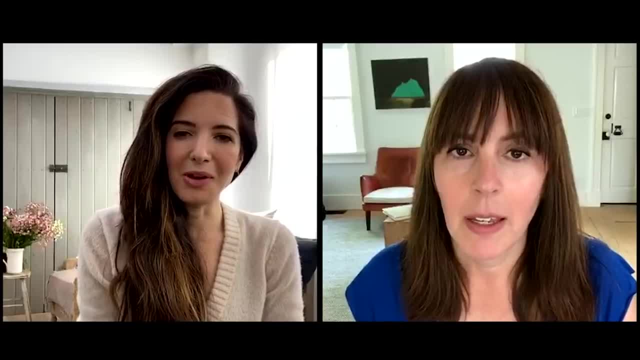 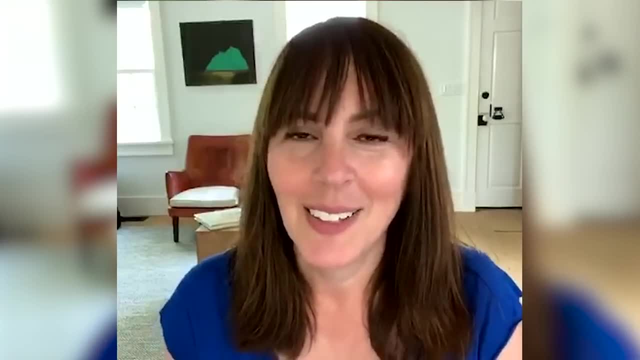 getting mad at a buffet because you can't eat everything like you don't get. you know how dare. this buffet exists. it should only be the things that i want right now. no, that's the point of a buffet. when you're writing everything like, don't start getting mad that you're writing too much and not. 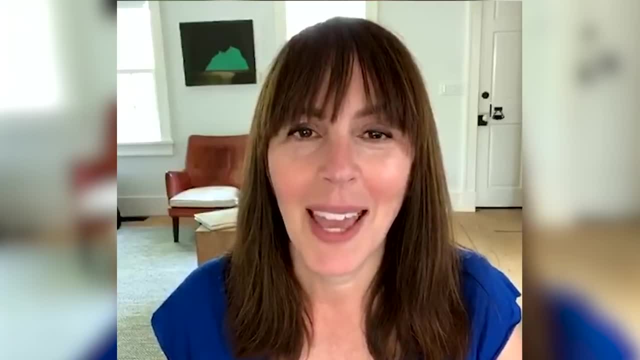 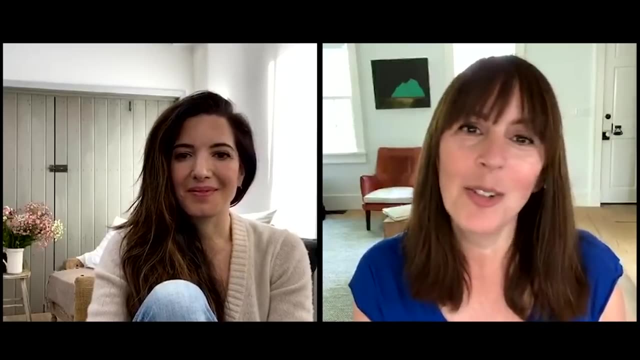 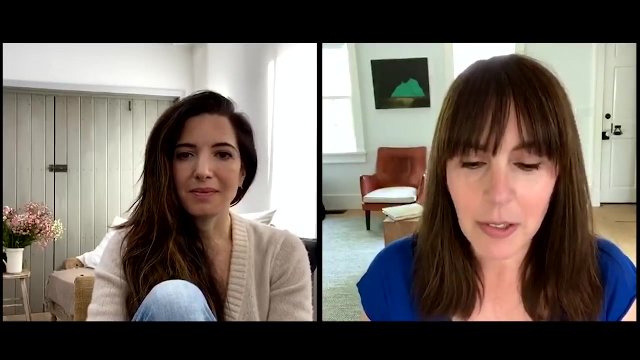 everything is going to go into it in the end. um, be okay with that, it's a buffet and later you can pick from the stuff that's really good and maybe you, you know, take a new plate and go back for seconds. but, like, stop being overwhelmed at that. um, and then also this: um, wonderful woman that i 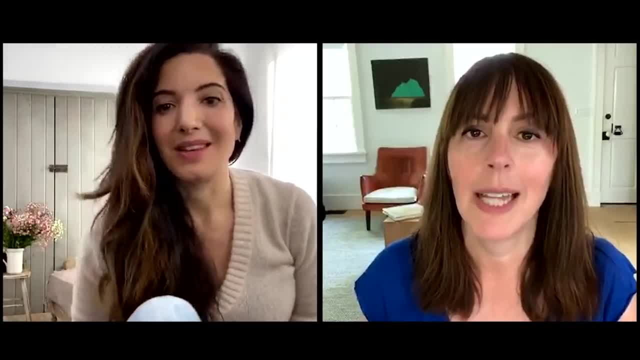 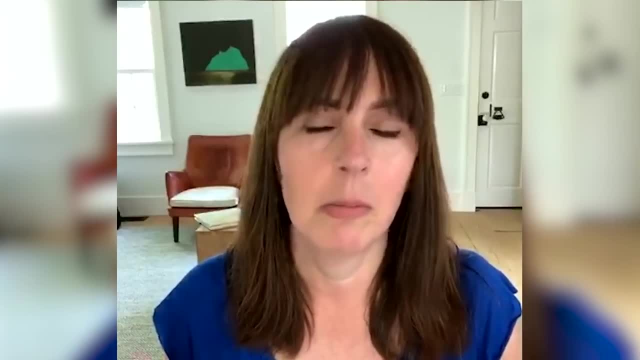 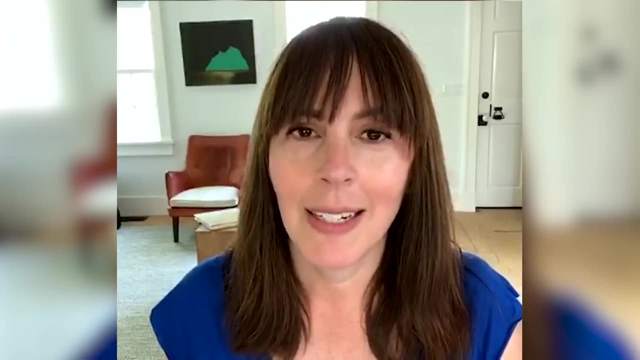 work with named suzanne kingsbury. she's been helping me with my book. she's an editor and i was on a group call and somebody on the group calls echoed everyone's feelings. basically, she's like i'm writing all this stuff, um, and i'm really worried that it's not going to come together in. 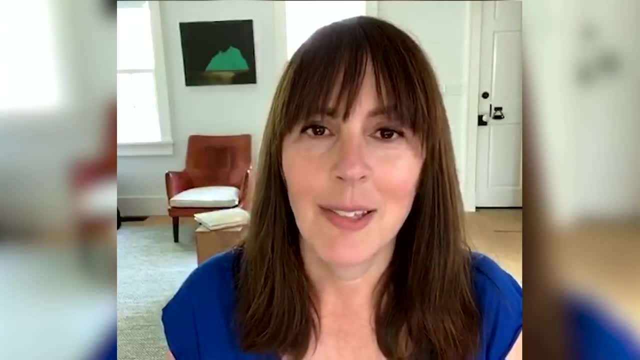 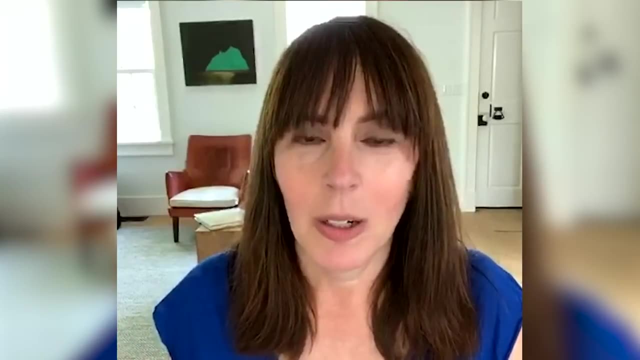 any way, that there's not going to be any theme to it all. and suzanne said: well, basically every keep writing, because everything in nature, everything in the world has a pattern. and you might not see the pattern yet. she's like: but slice a slice, open a pie. and i'm like: no, i'm not going to do that, i'm. 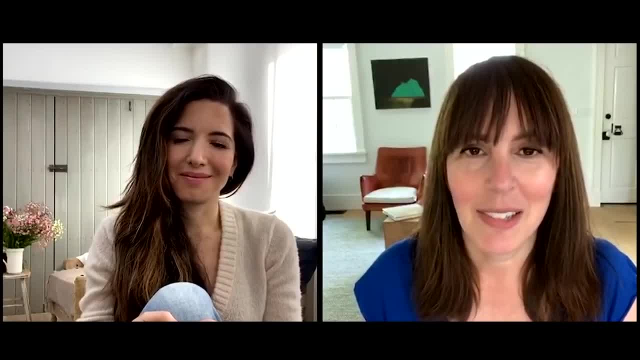 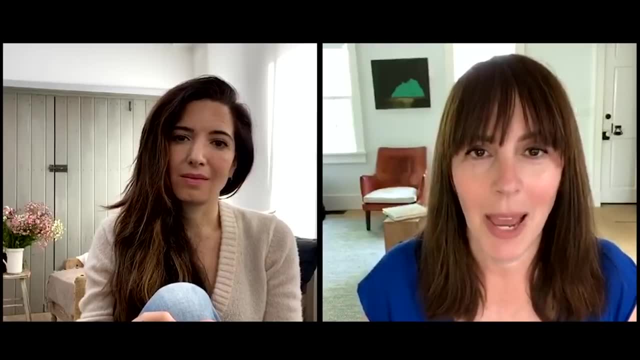 pineapple and you will see a pattern in there. and it's the same with your writing. you, you know you're not going to find it by just writing one thing: you've got to keep going, keep going, keep going and eventually the pattern will emerge. but just trust that and don't think that everything 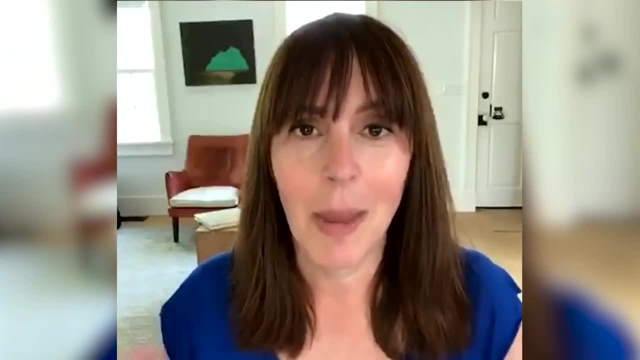 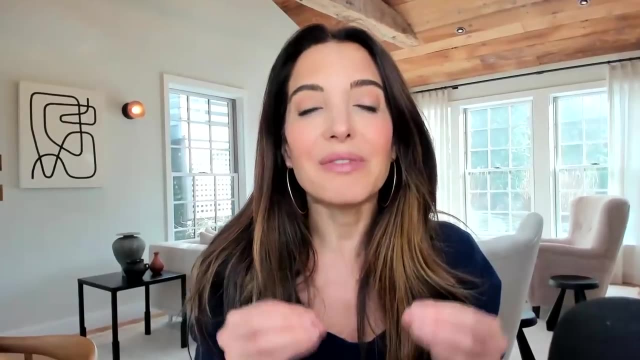 is going to come out perfectly, because it never is from the start. it's going to come out in one big mess and then you're going to find the theme later. you're going to find what's there later. if you want even more strategies to create high converting content, then you need to get your butts. 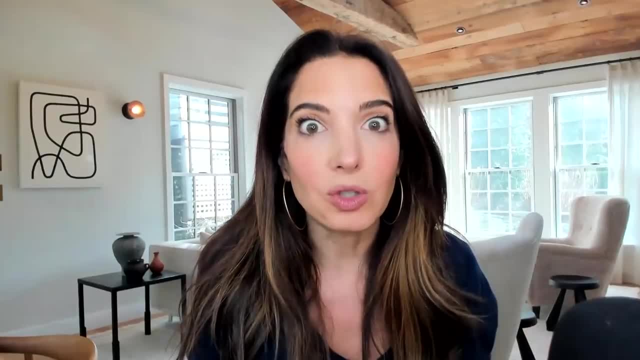 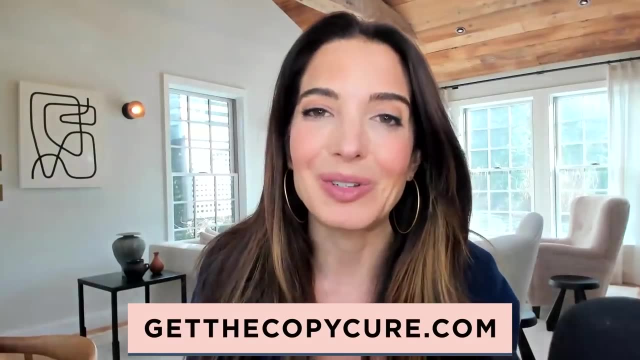 in the comments. copy cure. it's my flagship writing program. the door's just open, but only for a limited time. so to get started, go to get the copy curecom. now let's get back into it. i think it was back in maybe 2010, 2011. we were having all these conversations. i was starting to train. 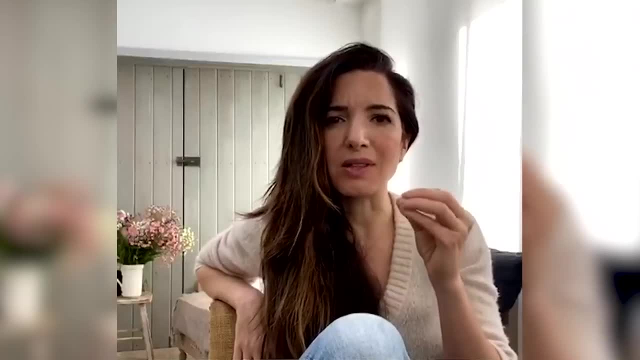 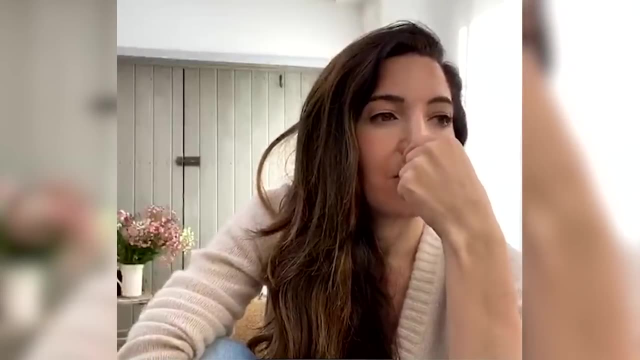 tens of thousands of entrepreneurs and i would see just smart business people who had great products and great services, yet they were falling down. i was like why? what's? what are they missing here? and it was had all to do with their messaging and their copy and the way that 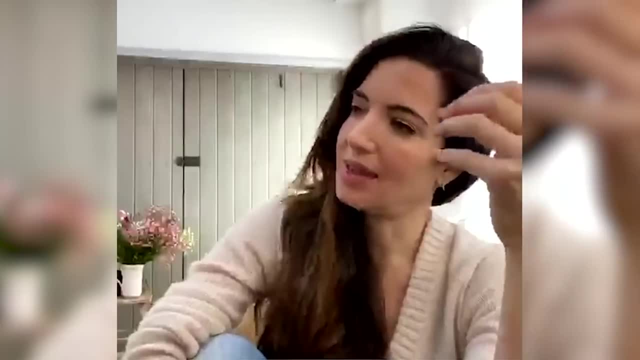 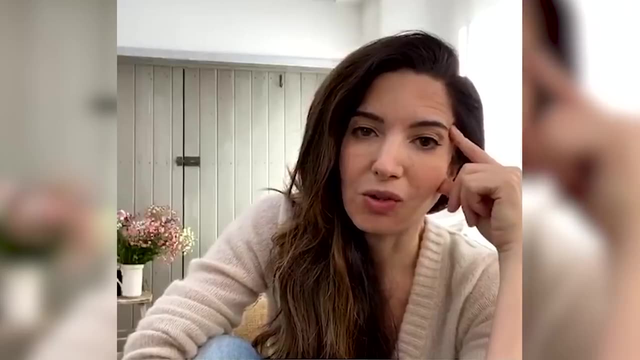 they were communicating about their incredible products or services and they weren't able to kind of bridge that gap. so laura and i um once we taught a live session together at a conference we used to do in, uh, new york city. so i used to do this conference in new york city. it was so amazing. 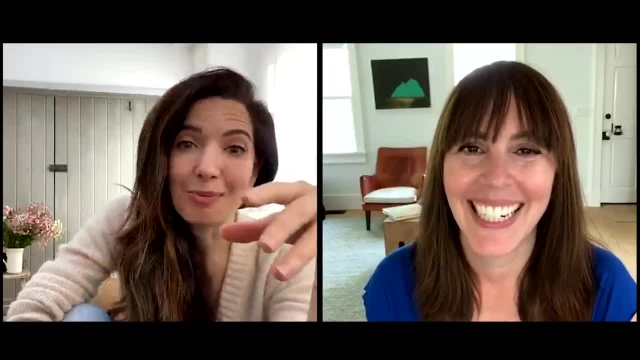 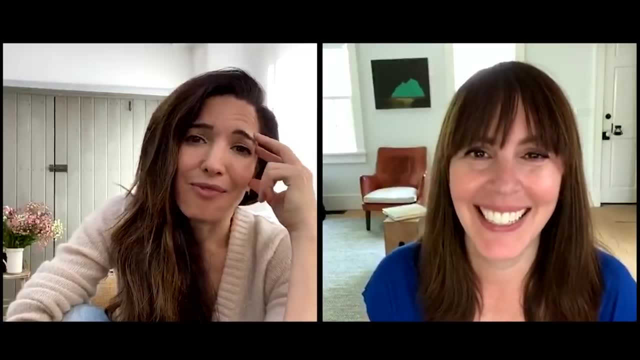 it was so good. oh my god, i had a wheel of dance. remember we would spin the wheel of dance and people would come on stage. it's just amazing. i'm feeling very nostalgic. yeah, i am feeling very nostalgic too, because i'm like you know what? we will have an event like that at some point in the 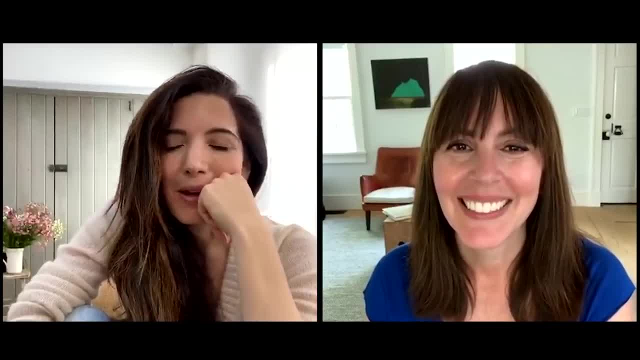 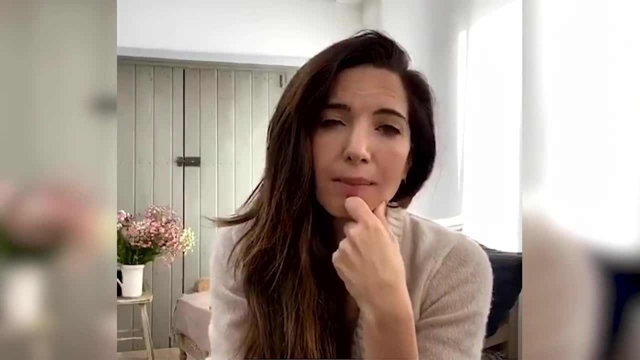 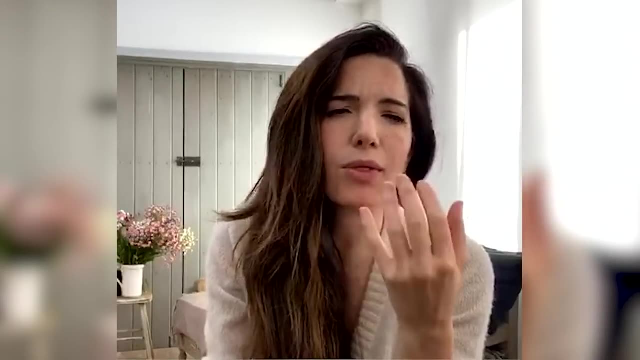 future again, yeah, when it's when it is safe for everyone to come together. i want to talk now about the power of like creative writing, and one of the things we promised folks for this self-care saturday was giving them some journal prompts, because, oh yeah, the more that you write and 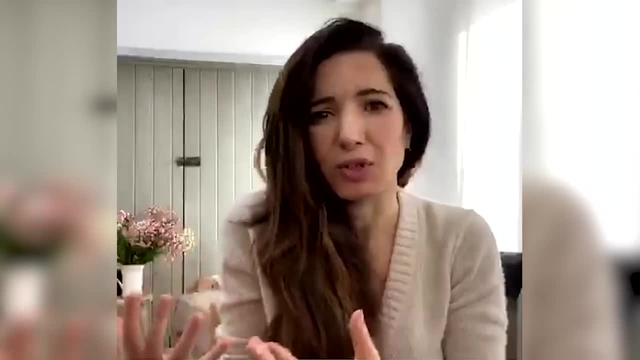 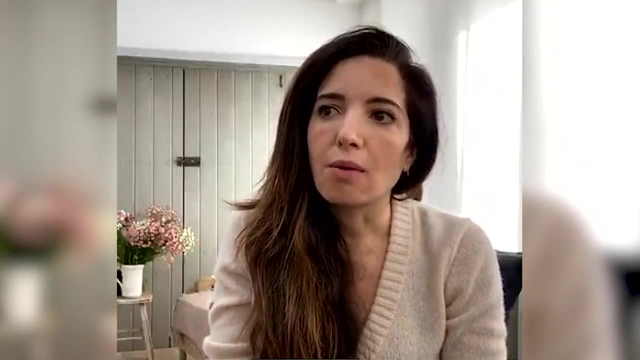 whether you write in an actual journal by hand because it just that feels good to you, or you want to take some of these prompts and use them to just get your writing flowing, um, for more professional oriented projects, and i think that's a really good idea. i think that's a really good. 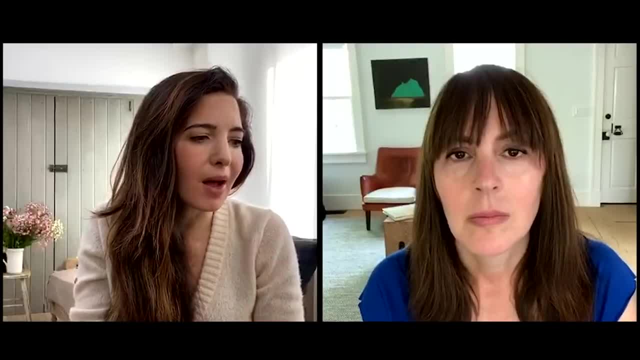 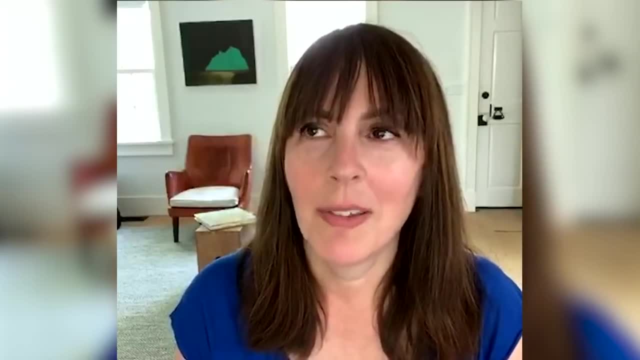 idea so you can do whatever you want with them. but, laura, let's set this up. tell me more about how you've been so passionate about creative writing these days and why. yeah, well, first of all, i always have been passionate about it, like in the abstract, like i want to do more creative writing. 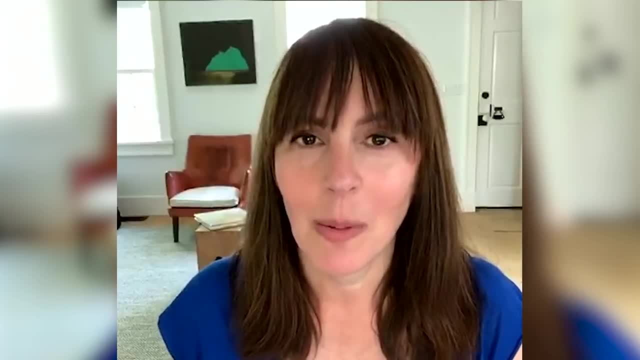 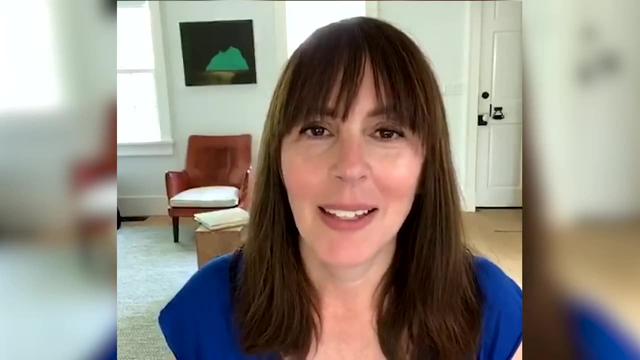 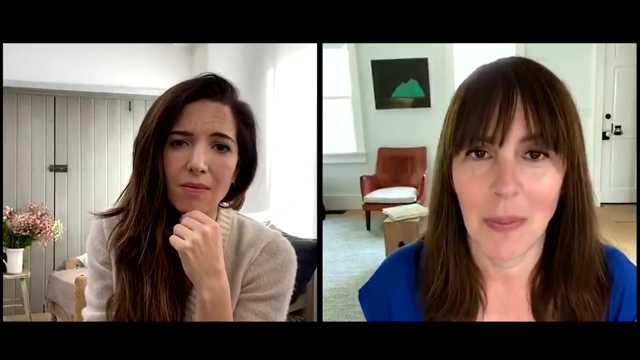 and i took classes that were great, that taught me a lot, but like where the assignment would be right just for 10 minutes every day. um, and very simple, very gentle, you know. and i couldn't even do that because i think i felt overwhelmed and like it had to be something and for some reason i don't know, 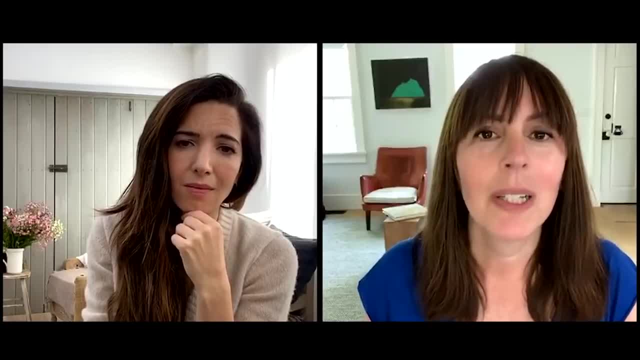 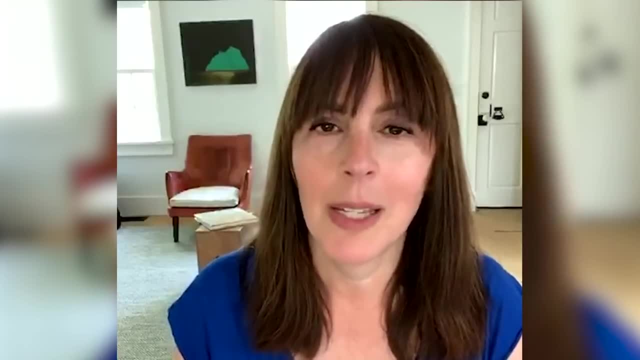 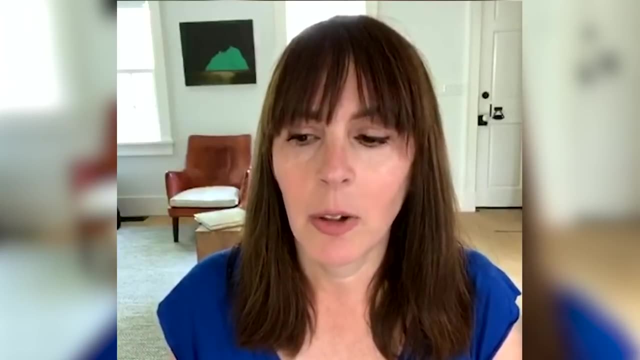 why it clicked when it did, but one day, a couple of years ago, it clicked up for me that i should write every day, just free. write every day i might. it might have been from reading the artist's way by um juliet cameron or something else, but i discovered um. i don't know how i came across it. 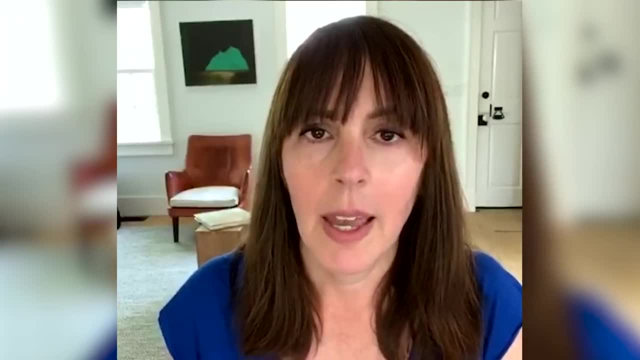 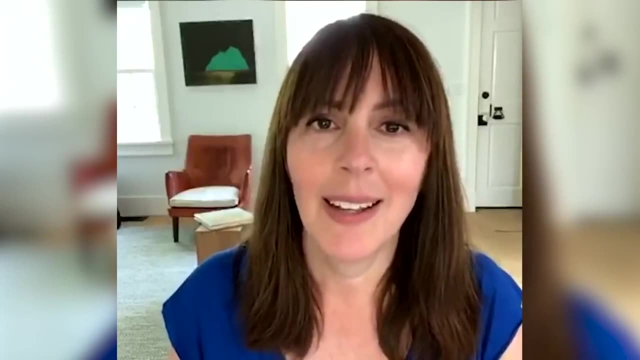 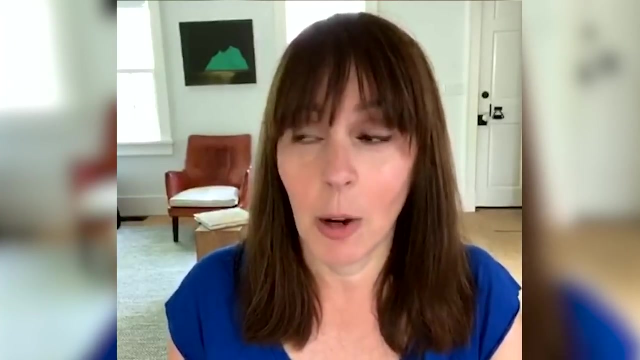 this site 750 wordscom, and so it's seven, five zero wordscom and it's just. it's a journaling website, um, it's free and you just write in it whatever you want to write every day, and or if you can go every day, it doesn't punish you if you. 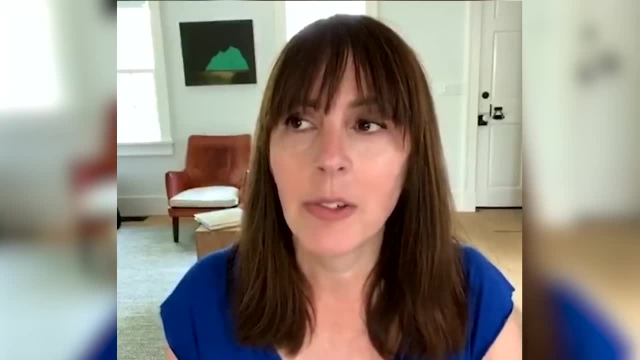 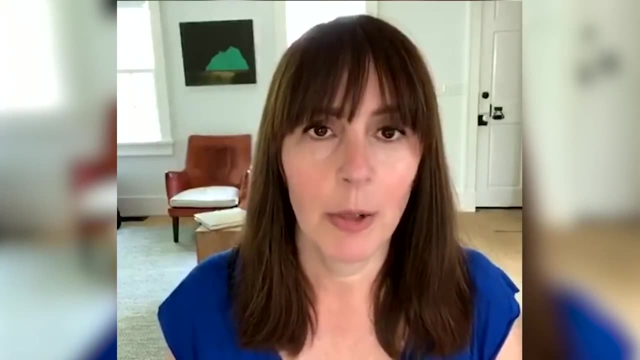 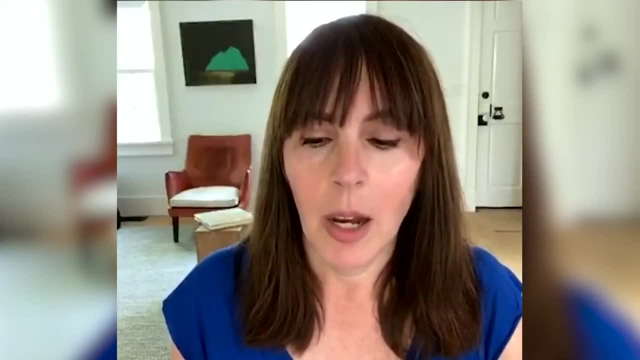 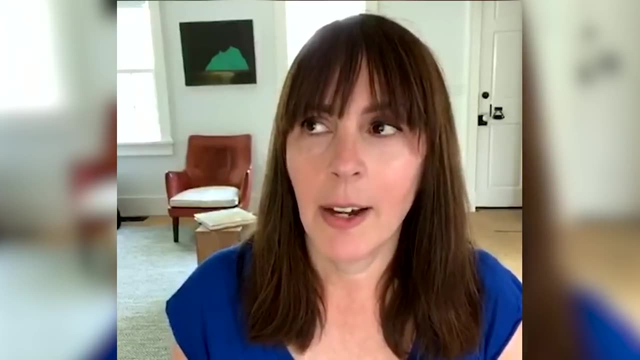 doing it. so this is, this is journaling, this is free writing. um, when i'm doing it, i put no pressure on myself to write anything. good, i might say, i might start out writing. i have nothing to write, i have nothing to write. i have nothing to write. i might write that for a while, and that's fine too. 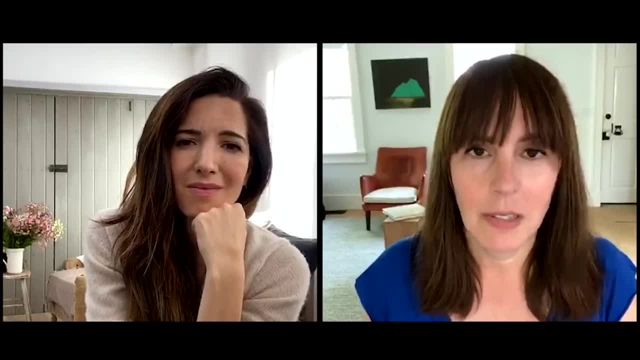 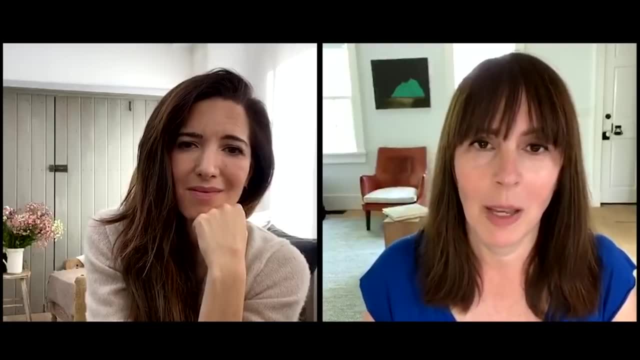 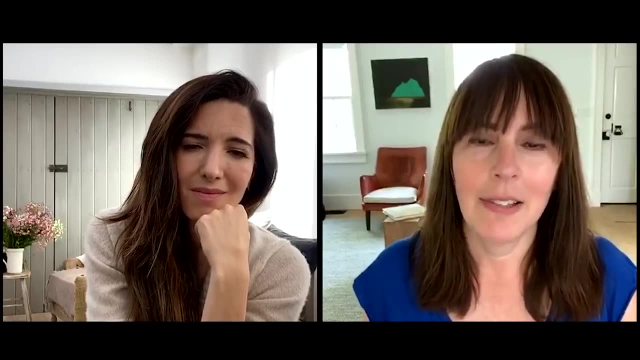 writing. i have nothing to write as writing as well, but it always turns into something. i always get on a roll. sometimes it's arduous to like. okay, here i am still writing my words. i'm almost at 750 words, but often i will get in a writing groove and as i write, um, you know, a couple of things happen when. 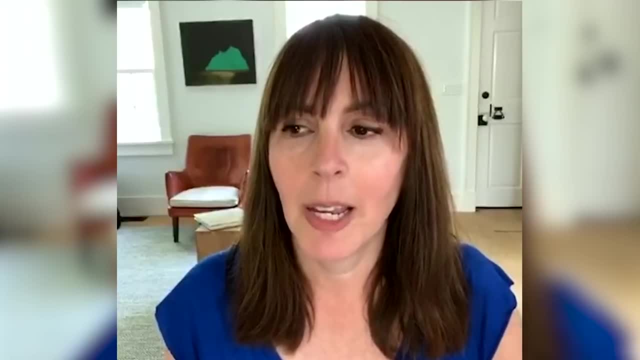 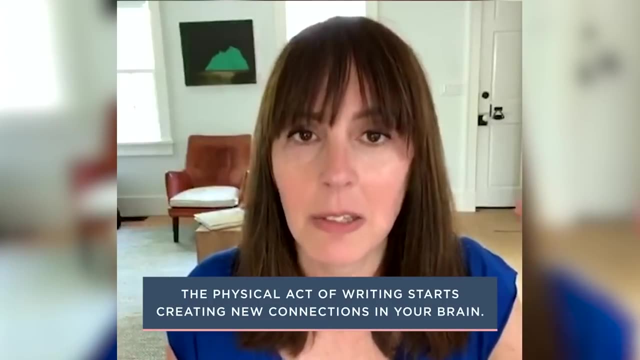 you write one one of them is that you generate new ideas like your brain's. just the act of writing, the physical act of writing, starts creating new connections in your brain. so you start getting ideas as you're writing and when you write them down, those create more and more ideas. it can. 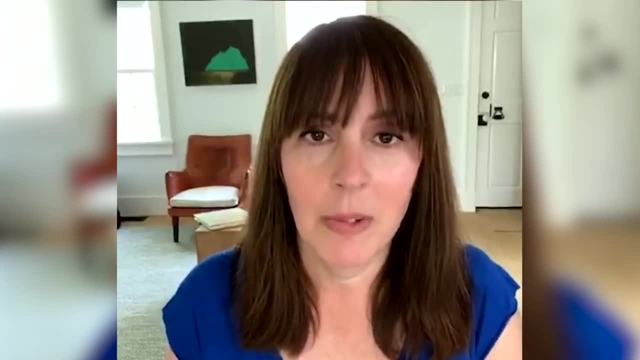 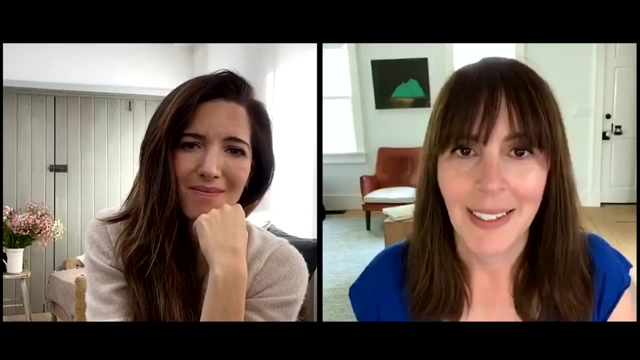 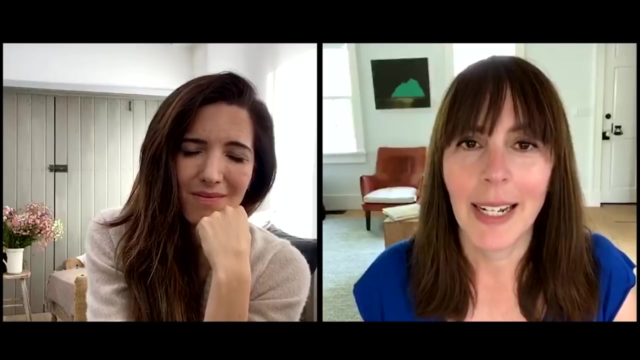 almost get overwhelming. but you just keep going and writing and writing them down and you also get in a mindset: um, i think you train your brain to shut off the critic, the inner critic, that this is no good. because it doesn't have to be good. no one is going to read it. and when you, when you're able to, 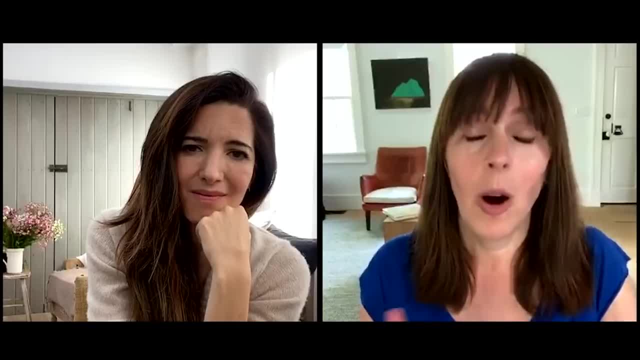 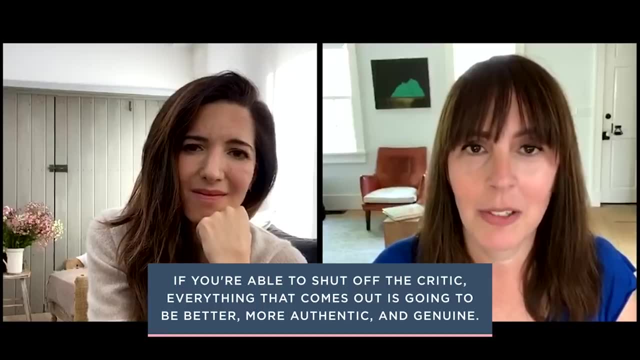 do that you write so much better when, when you are indeed writing for somebody else, for an audience, um, you're, if you're able to shut off the critic, everything that comes out is going to be so much better and so much more authentic and genuine and um. 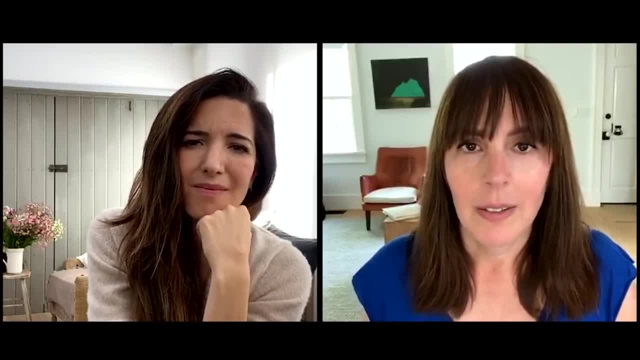 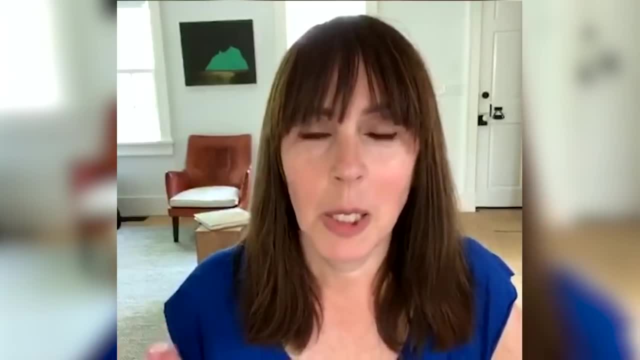 things come out of you that you don't know. we're there like it's, you know it's almost like a dream state, right? you have like your subconscious. there are all kinds of thoughts and pictures and um ideas inside your brain or inside your heart, wherever they are, wherever they're lodged. 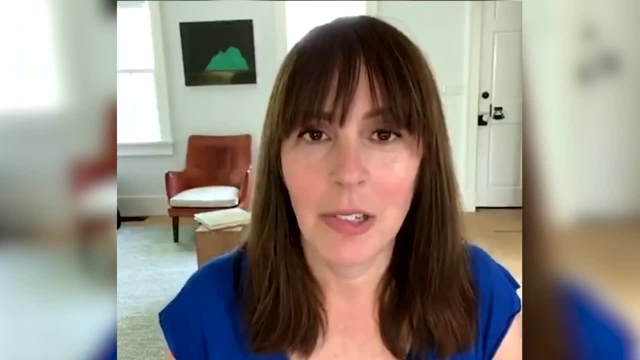 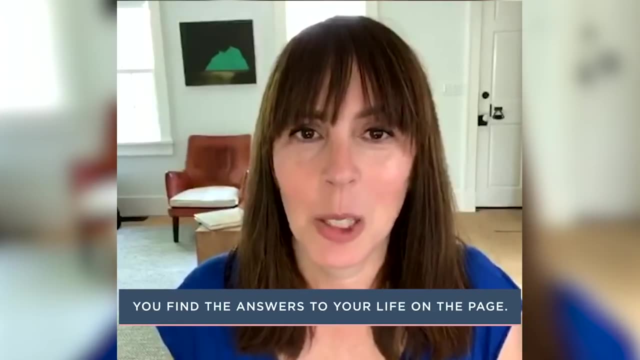 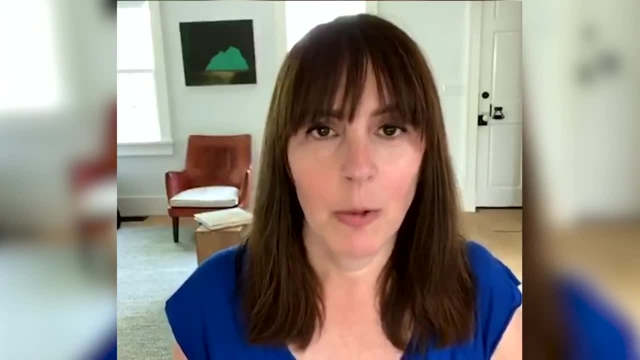 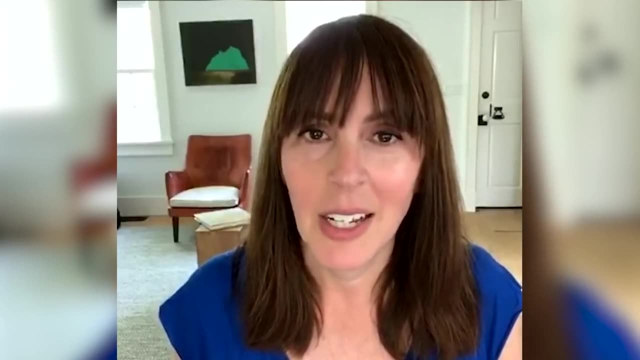 it creates meaning. if you're looking for answers to something, if you're writing about something that you can't figure out or that's bothering you, or that you think that you feel you're stuck in, sometimes you will find an answer to it. here's why i'm that way, like, or here's what this means. 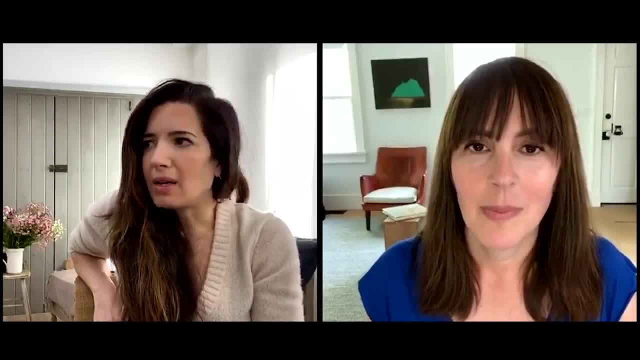 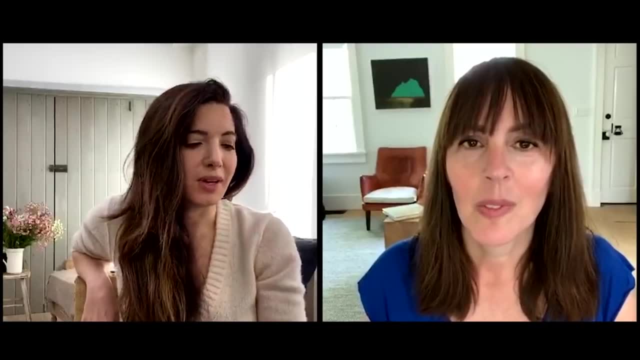 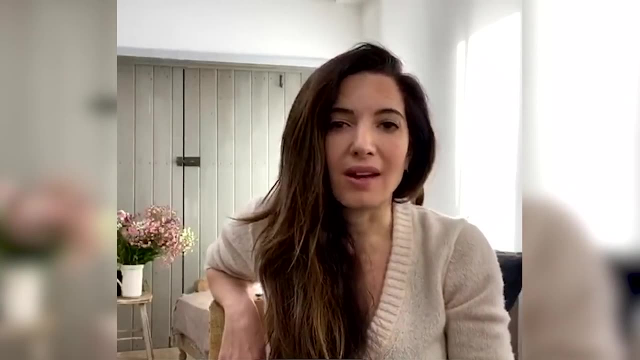 and it's kind of miraculous, you know. i so agree with that because i think that each of us- you know my position, that i've always taken as as a coach- has been: hey, i don't have all the answers, but i'm going to help you find your own, and i think that writing is one of the most brilliant ways to 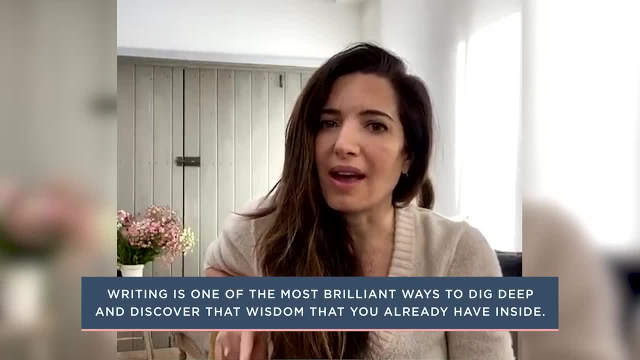 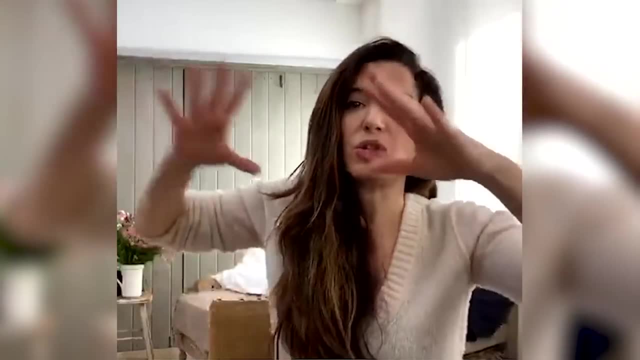 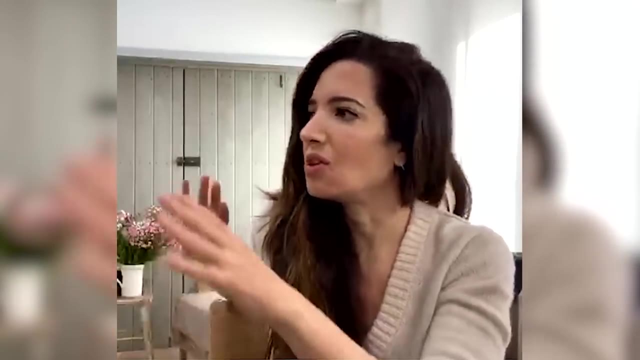 dig deep and discover that wisdom that you already have inside that is sometimes hard to perceive or to hear with so much noise in the world around you. you know and the demands of every life and responding to emails or texts, or you know, taking care of your family and making meals, and you're 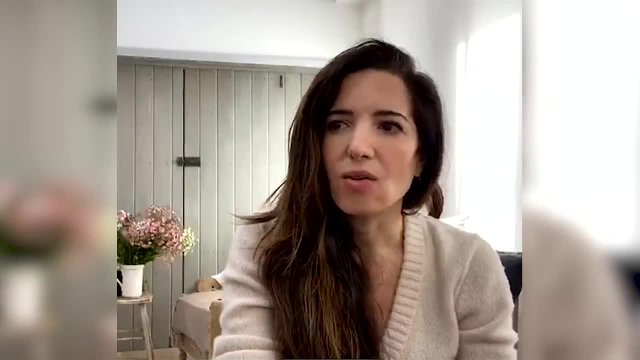 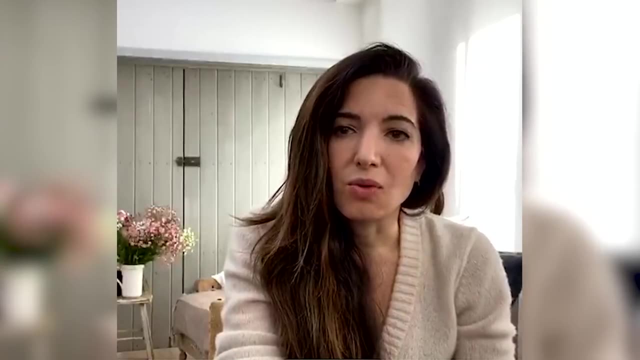 just doing the normal things of everyday life. but there is something incredible that you can do to help you find your own, and to help you find your own and to help you incredibly transportative about writing and being with yourself and your own thoughts that we don't even you know. i mean usually in our culture right now, we don't take time to do that. 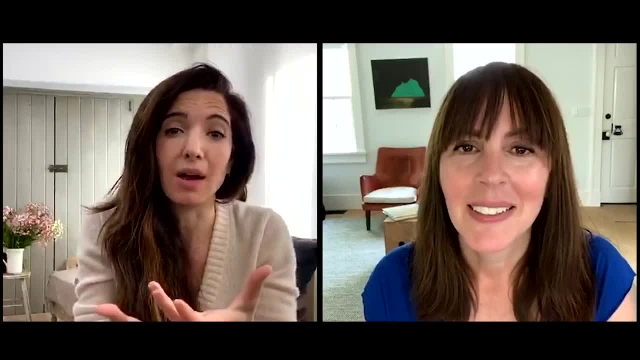 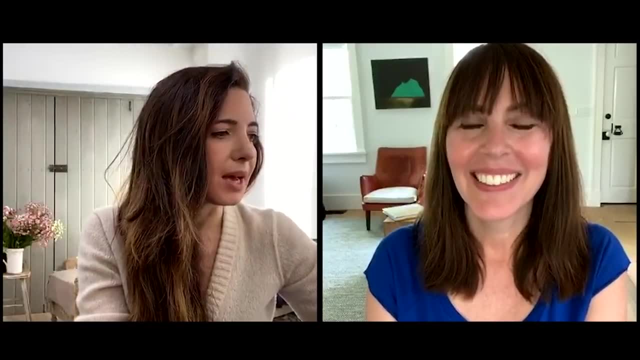 very often it's like the moment there's downtime, it's like we pick up a device and consume rather than create. anyway, you know, what i'm gonna do is is add some, um, add some prompts into here. so these are actually some prompts, you guys, that we have from the copy cure, which is amazing, and this is. 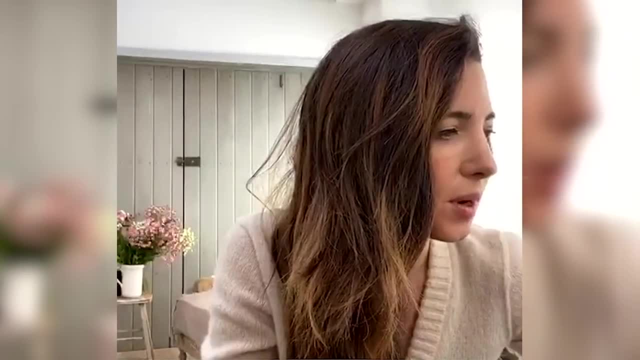 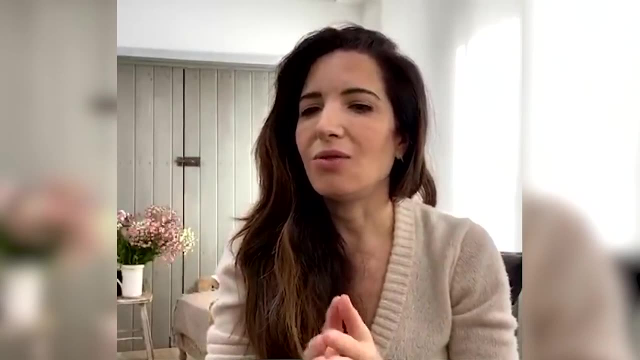 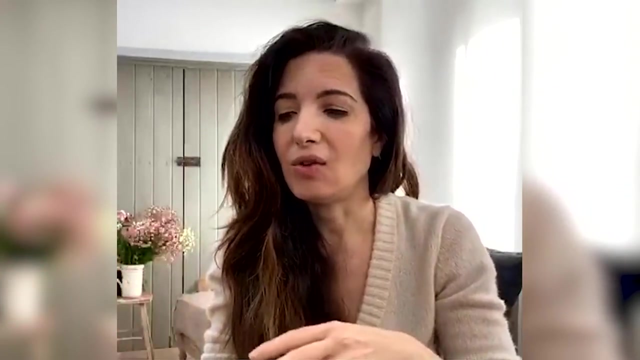 from a list that we share: 121 writing prompts and 24 selling segues. what that does is help your brain start to think more creatively, so that you never show up at the blank page and go, oh goodness, i don't know what to write about today, or if you have a great story to tell and then you need to. 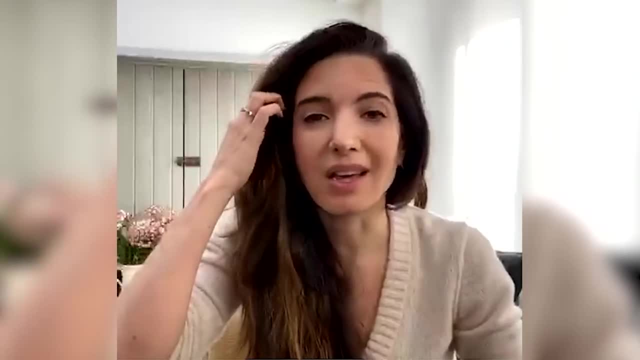 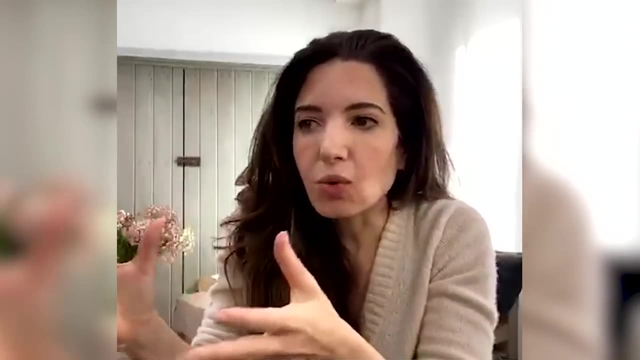 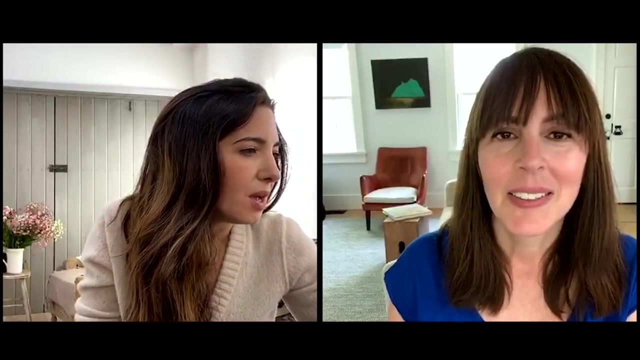 transition into an offer or something that you want to share. it can be a campaign, it can be a people to take action. how do you actually bridge the one story you're telling or the narrative into something else? um, so i'm gonna choose a couple. let's see what was your favorite. 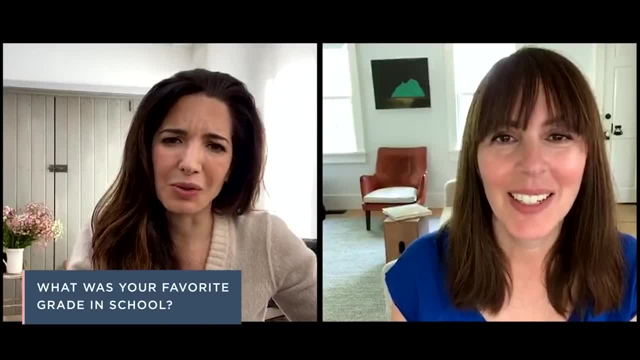 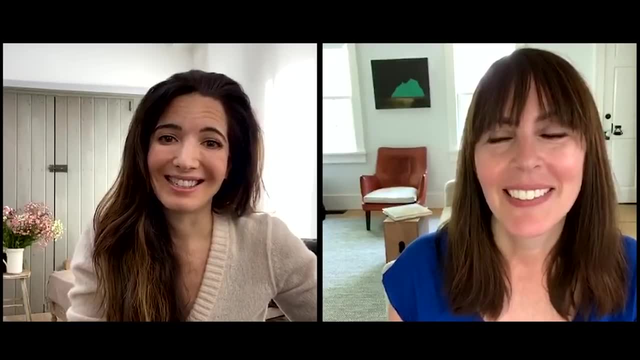 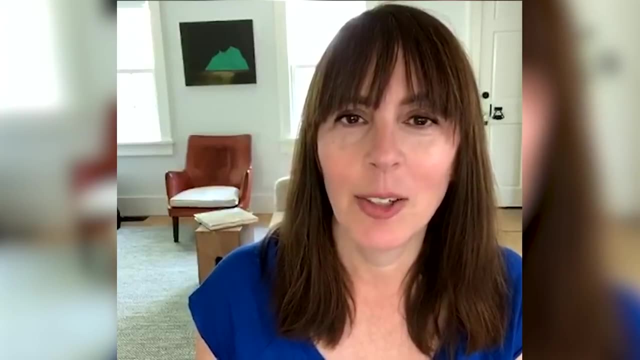 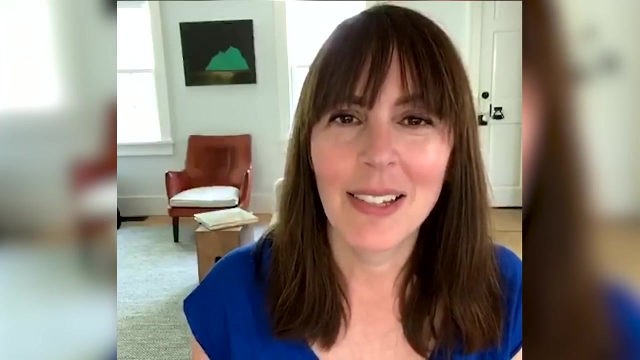 grade in school. what was your favorite? oh, that's good. my favorite grade, i think, was senior year, 12th grade. why? i think that's when i felt the most confident about who i was and i knew who my friends were and, um, i think also we had electives that year and i did some creative writing. actually, i think that was. 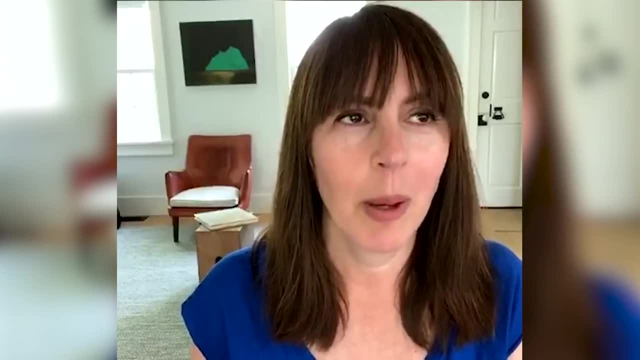 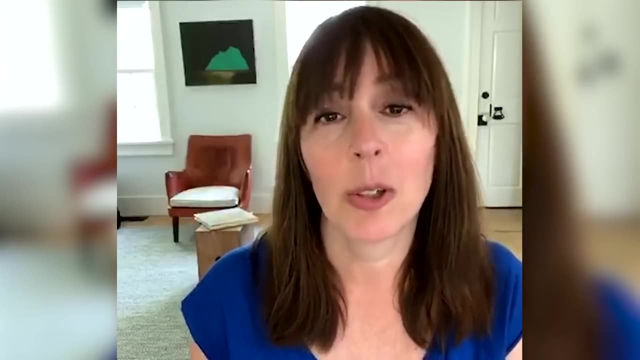 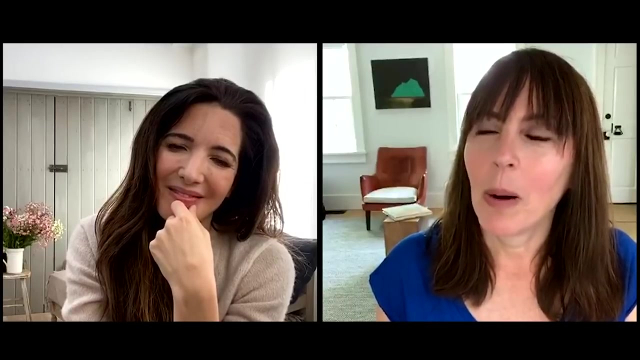 yeah, but i also just i just enjoyed senior year and i remember also driving around with my friend anna in her car because she could drive and we would just drive barefoot. well, she was barefoot um through the city and i just remember like we'd park in whatever. her dad owned garages and we 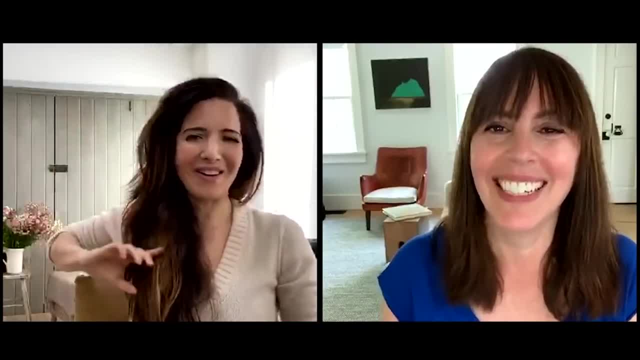 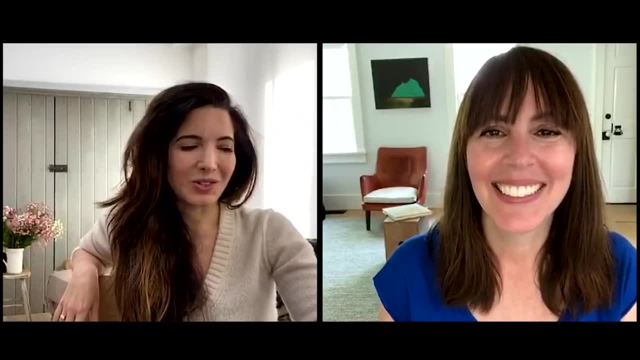 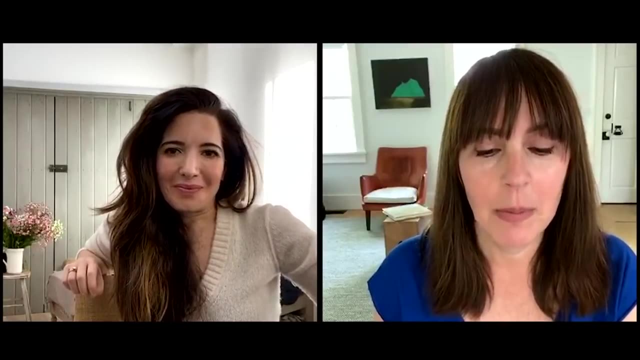 would park in the city and get frozen fruits and go shopping and that's oh, imagine you in the city as a, as a senior, like i just can't even. you're just such a fun troublemaker. i love you. i was pretty innocent as a baby. i have some- yeah, i have some- prompts that are good for right now. 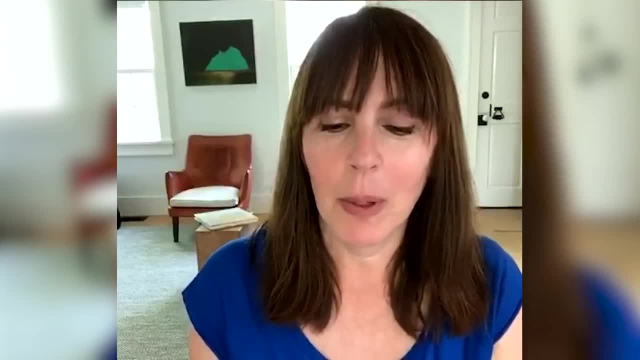 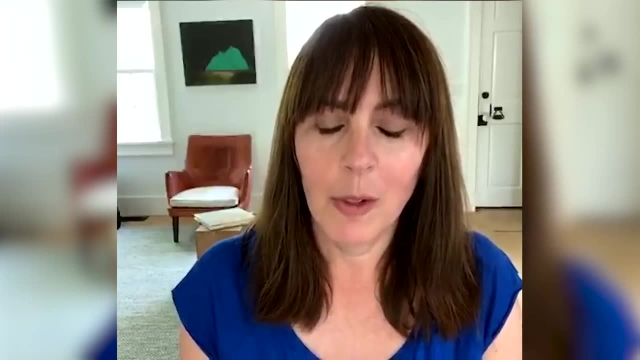 if you want me to read them, because i i think people like what what's on our minds right now is what's you know, quarantine pandemic and all that. so one thing if you want me to read them like in a positive mindset, is um three things that made life better this week. 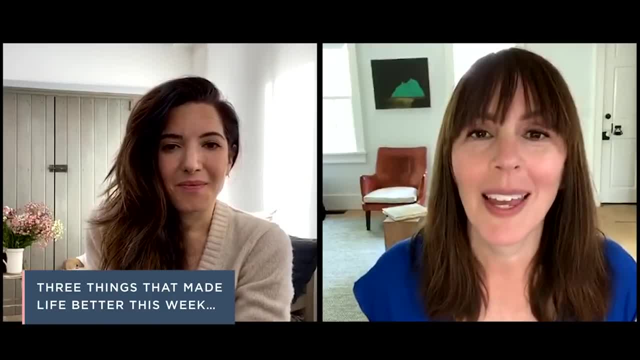 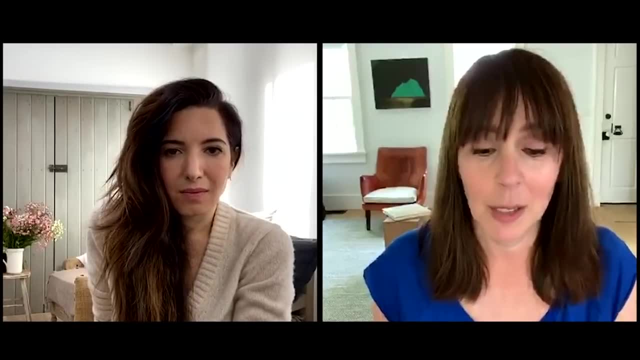 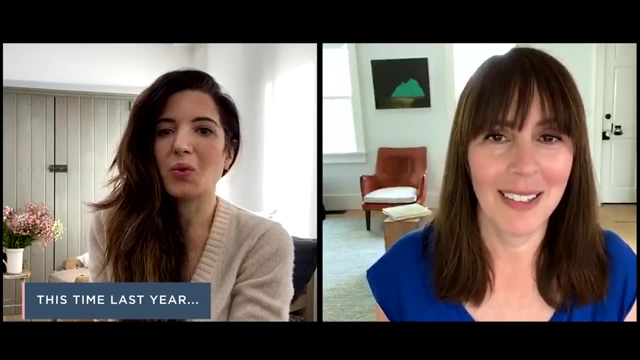 and you know it can be just one thing, but just writing, like even even creating a list, is a great writing exercise. um, so it can be three things. that could be as many things as you want. um. another prompt is: this time last year, finish this time last year. what is this? this is like may something. 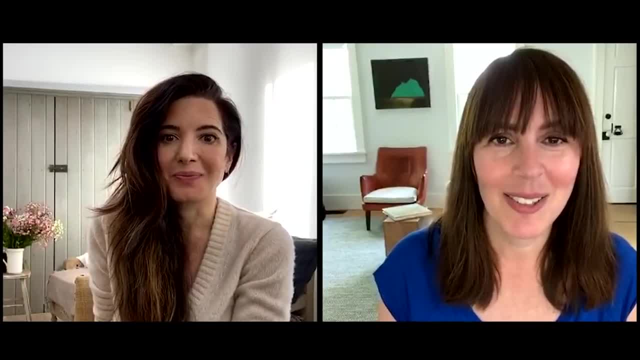 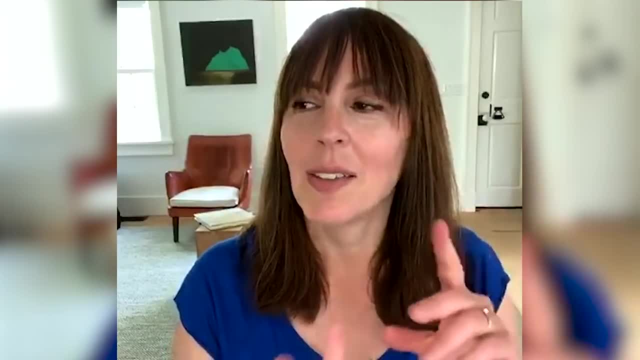 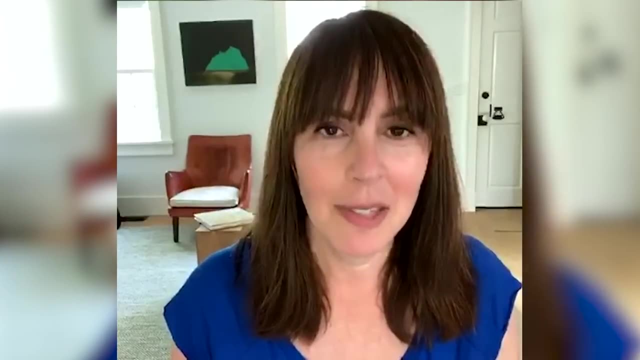 we're in the middle of may, wow, middle of may, starkly different world, right and like. by the way, i will say that i i think that we it is. there is incredible value for all of us right now in writing down what's happening in our lives. yes, because you think every day is the same and you think your life is the same as. 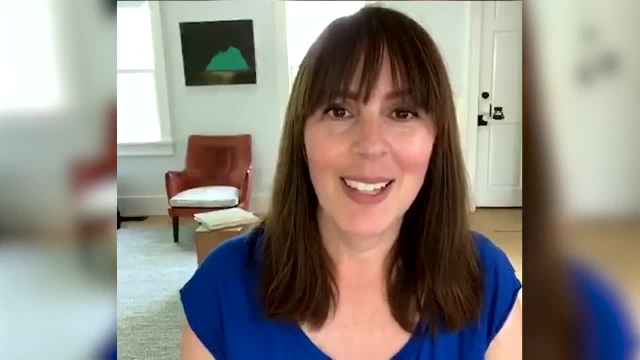 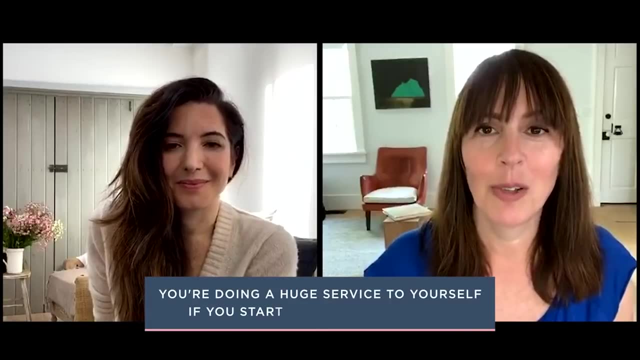 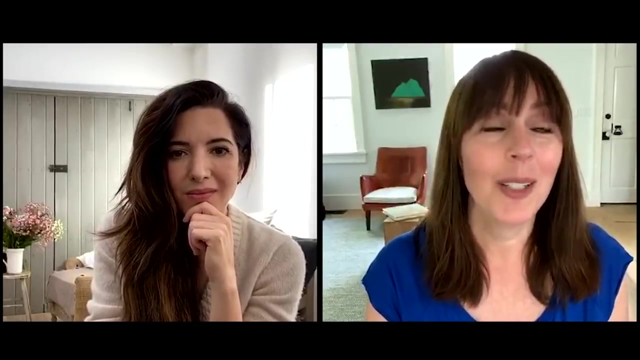 everyone else's, but it is starkly not, and so writing down the details also, you think you will remember and you will not. so you're doing a huge service to yourself if you start recording your life. it'll be incredible to look back on um and and a gift to other people. you know when, when you tell. 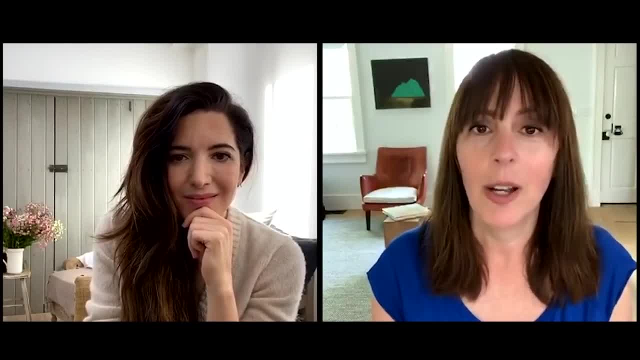 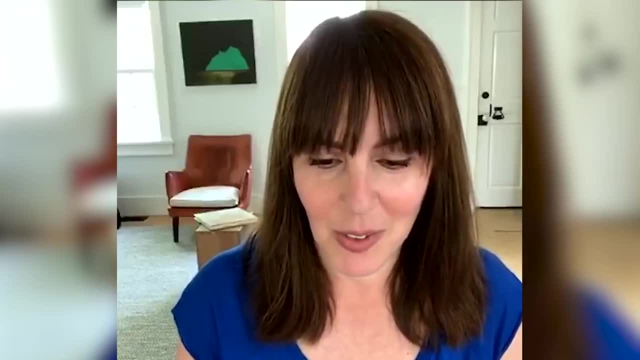 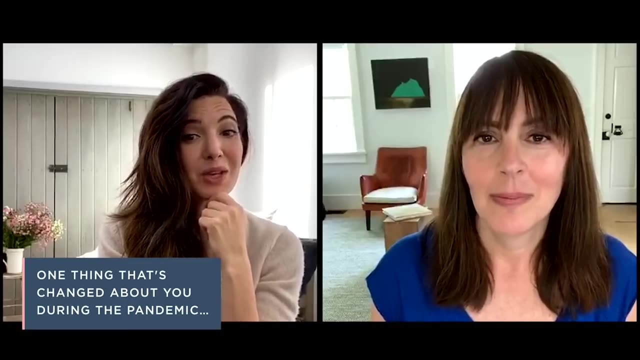 stories of this time to your kids, your grandkids. you know people who weren't here for it. um, you will have this record of things that you never would have remembered. so there's, that's another one this time last year. um, one thing that's changed about you during the pandemic, oh so. 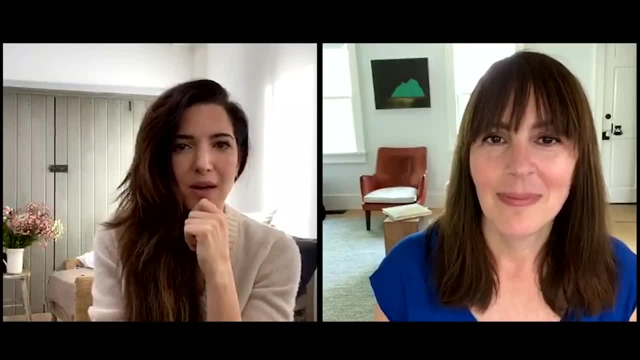 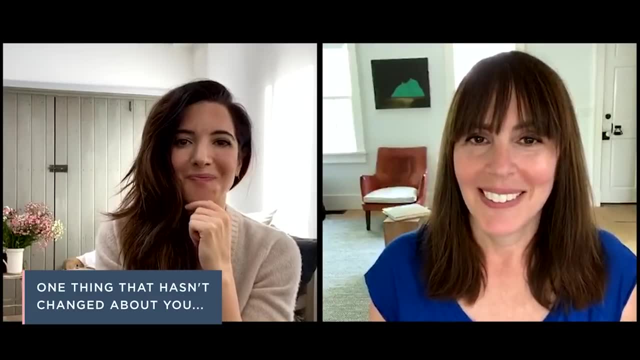 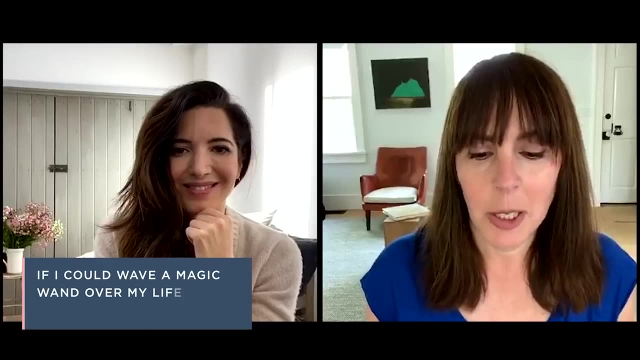 what's one thing that's changed about you during this, these past couple of months? yeah, yeah, um, one thing that's changed about you during the pandemic? um, let's say, and one thing that hasn't. here's one that can is for any time. if i could wave a magic wand over my life, here's what would. 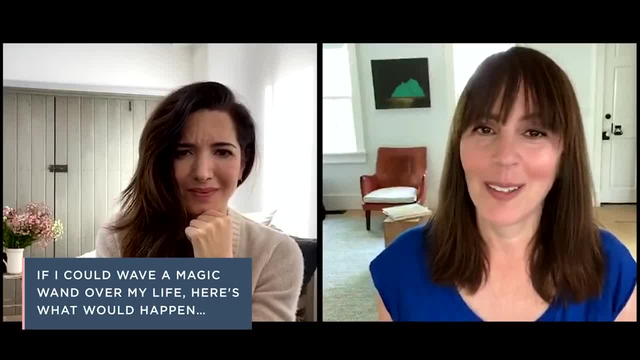 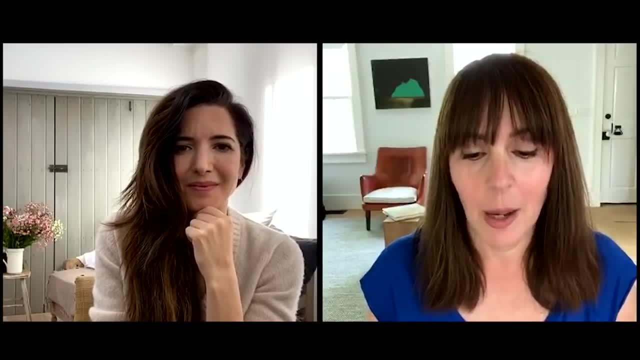 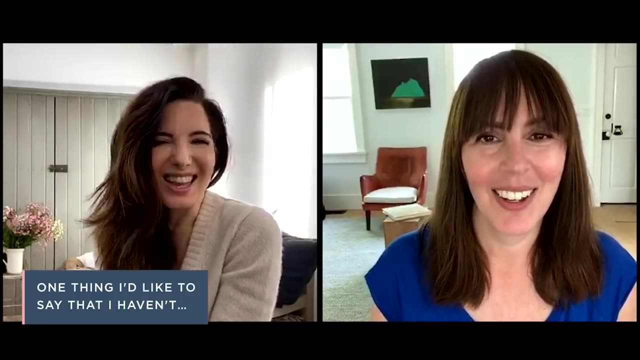 happen and that that might have nothing to do with how things are right now during the world. you know, but- and like you can use that anytime, um, another thing for any time. one thing i'd like to say that i haven't, oh So yeah, I'd like to say, but I haven't. Yeah, so that might be to somebody you know, it might be. 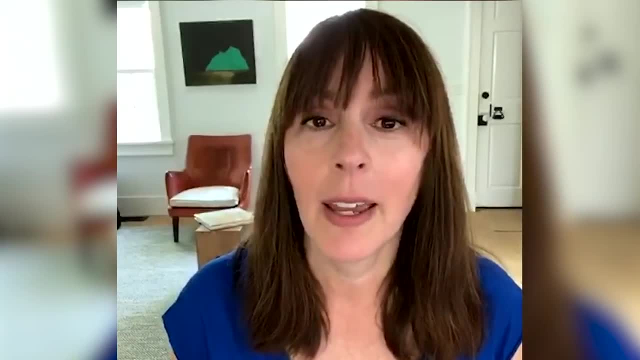 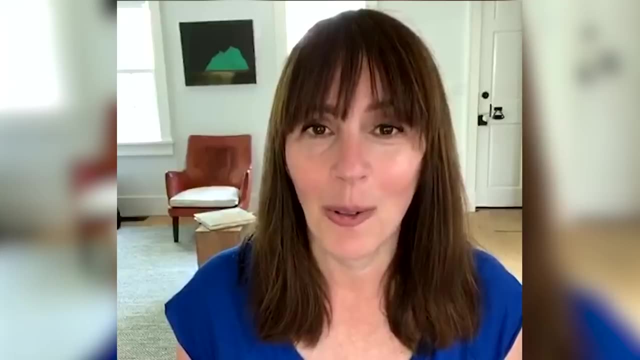 to somebody who, like, came too close to you yesterday not wearing a mask. or it might be something you want to say to the world, or it might be something that you didn't say to your friend on the phone that you wanted to say, but that's always good And probably most of us. 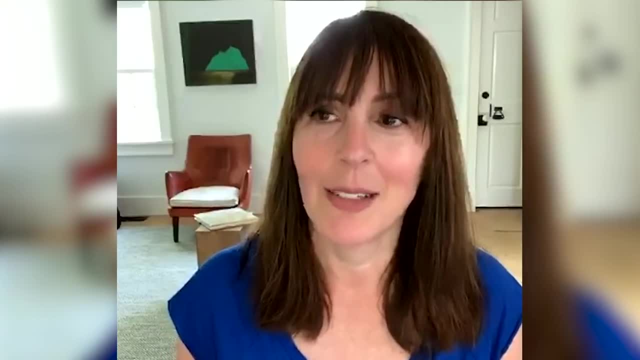 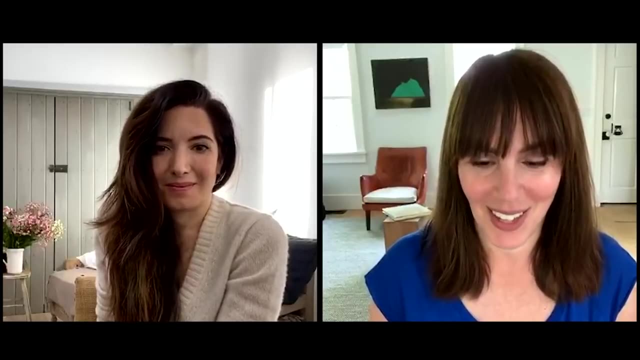 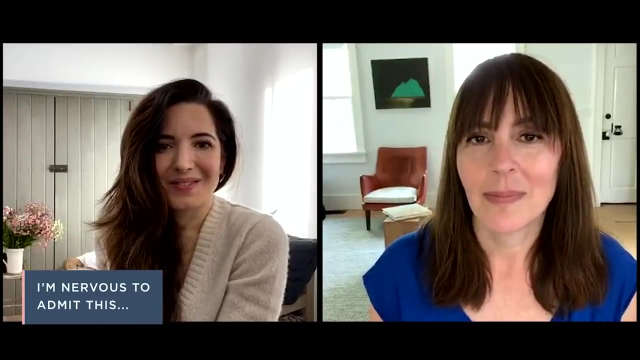 especially as women have something to say that we didn't say. pretty much every day There's always something that we wanted to say and we didn't. So that's a good, that's really good one. Here's another one, good for anytime. I'm nervous to admit this. Oh, I love that. I even feel like 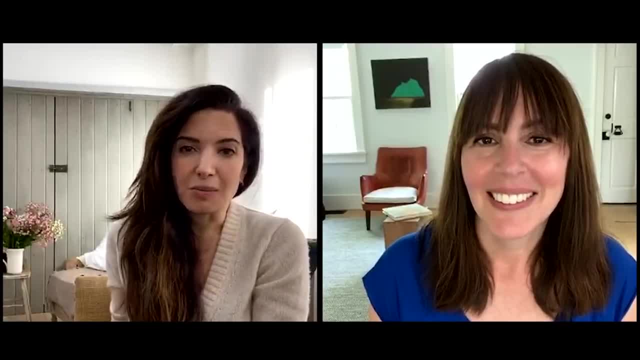 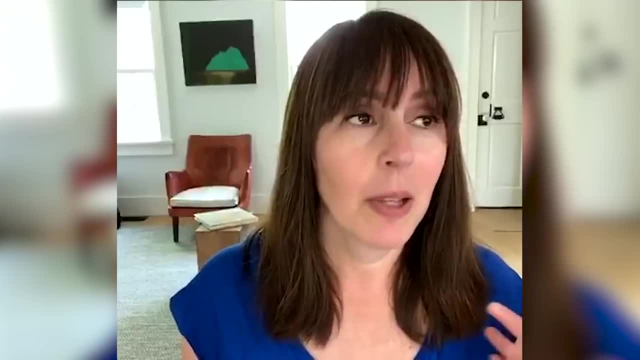 I'm nervous to admit this. It's actually also a great subject line. Yes, that is a great subject line. I would open that all day long And that's yeah, that. that might be about something you're shamed of or embarrassed about, But it might also be about something that you want, Because 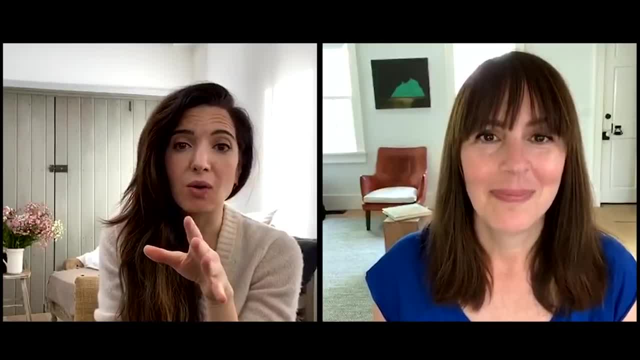 aren't we? It's something that you have because our culture is so adept at shaming people if they're even feeling good, right, You're not. you're like: damned if you do, damned if you don't- Yep. 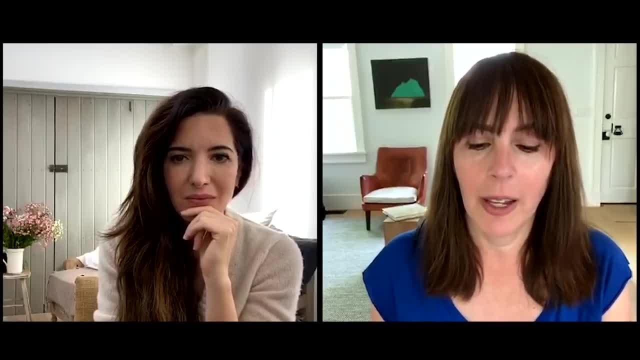 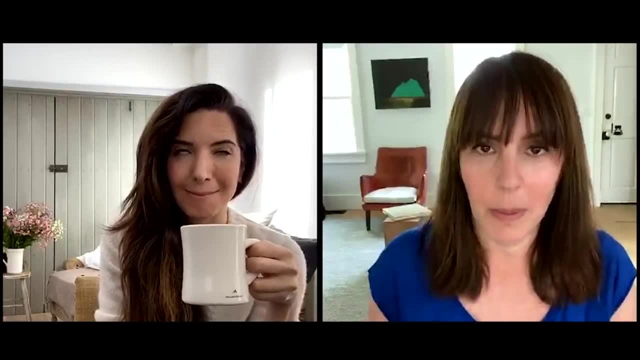 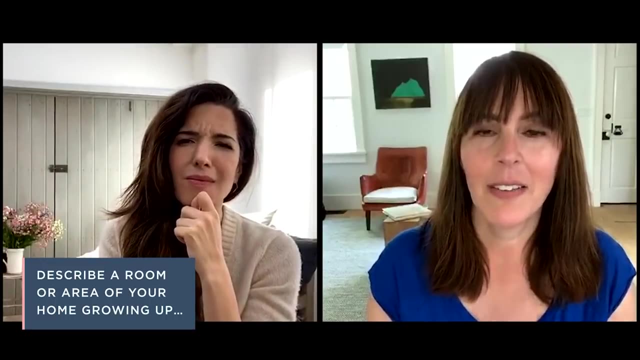 Yeah, And here's one like a great creative writing prompt for to get you in the mindset of using details, concrete details, painting a picture with your words. Describe a room or area of your home, growing up in detail that you can see any area. it could be a closet. 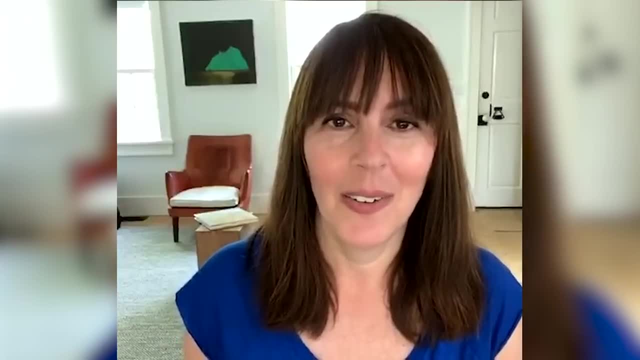 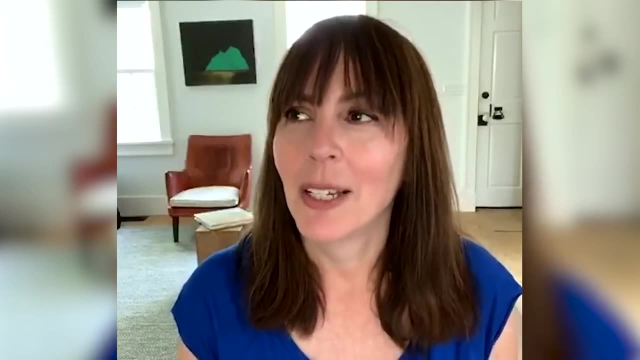 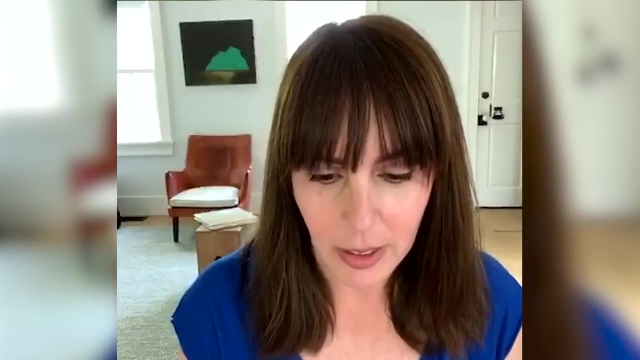 it could be your bedroom, it might be, you know, the clutter on your mom's desk, any area of your house, And you will find so much. you'll discover so much about yourself and your family and how you grew up in. just in just writing that And then, when you're at a loss for prompts, I mean you can. 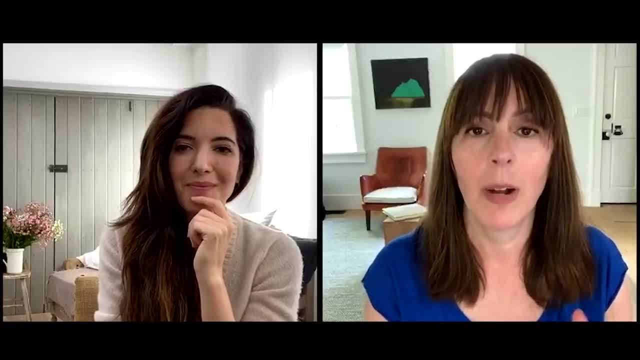 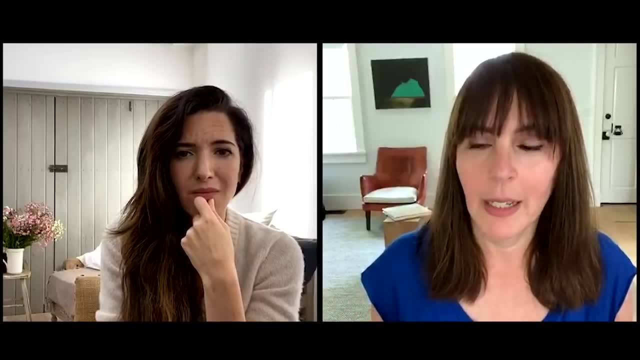 like our prompts are amazing in the copy cure. these are going to also help you write for an audience. But anytime you just want to write for an audience, you can do that. And then when you're at a loss for prompts and you want to write with one, an easy go to prompt for your creative, your. 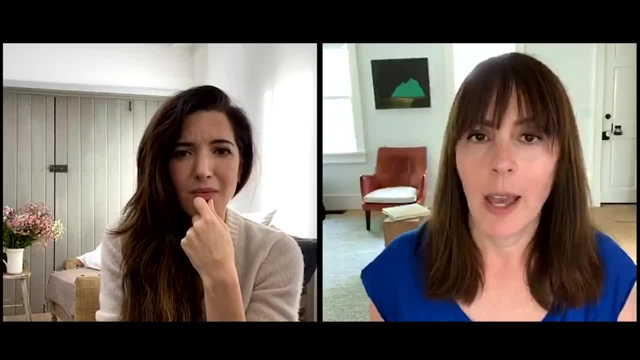 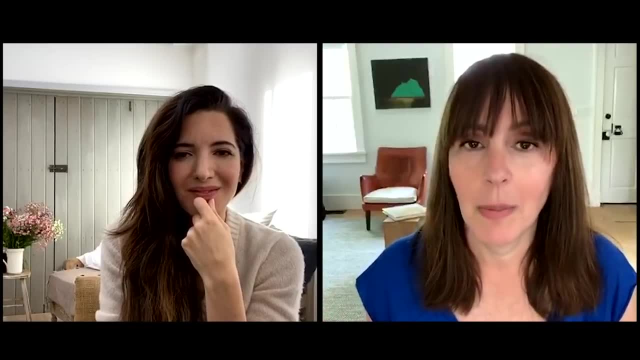 own writing, like open a book or a magazine or whatever you see in front of you and pick the first word that jumps out and let that and let that spray. you have just write anything that comes to mind. it doesn't have to stay to remain about that thing. So like it might be the word, 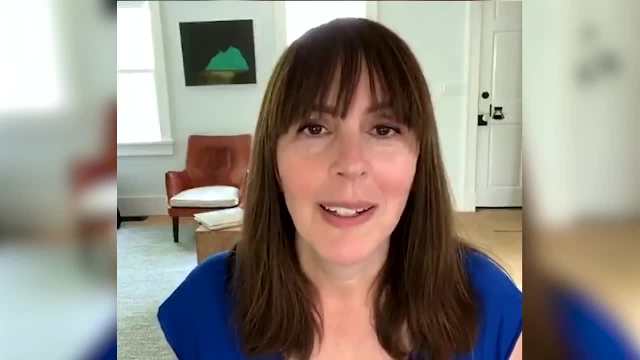 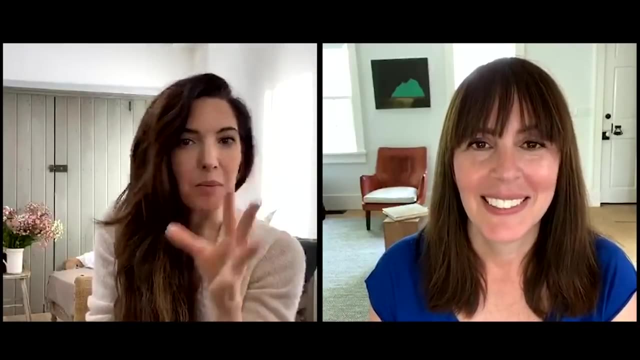 urgent. or it might be the word secret, or it might be the word soap. We all have stories. Yes, It is. It's like writing improv. Yeah, it is like someone throws out something, or you just latch onto one word and you're. 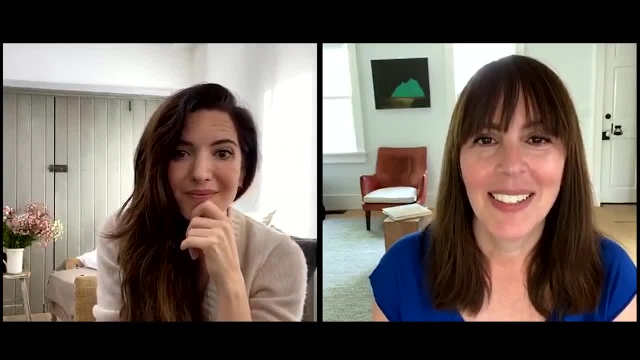 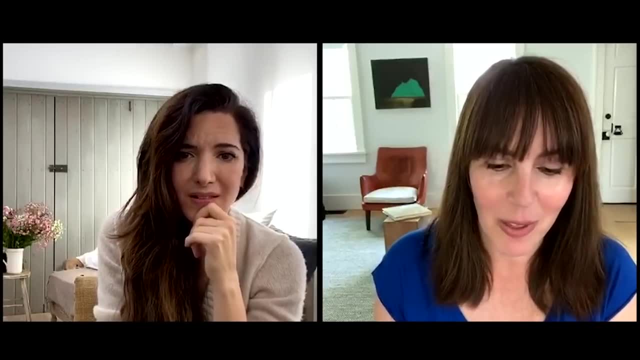 like, okay, we're going to go with this Boom, Yes, Yes, exactly. I mean I think soap and I think of so many different things and different stories, So it's just that I could go with, So you can attach any meaning to it that you want, And then okay. 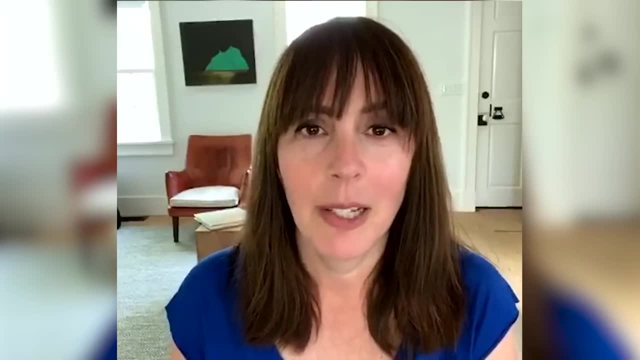 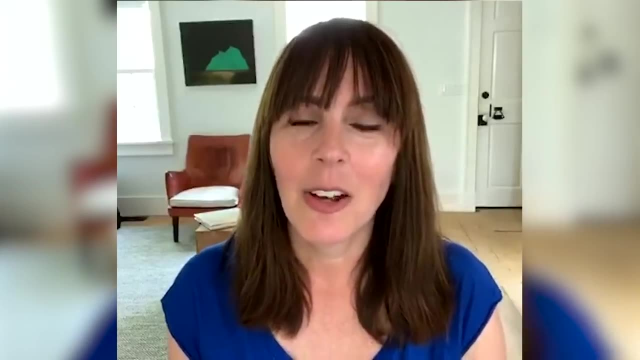 there's this really cool thing that I want to share that I got from our friend, Danny Shapiro, whose workshop I went to. So she's a bestselling author and she's amazing. She also teaches writing and she taught us this sort of- it's sort of a meditation. 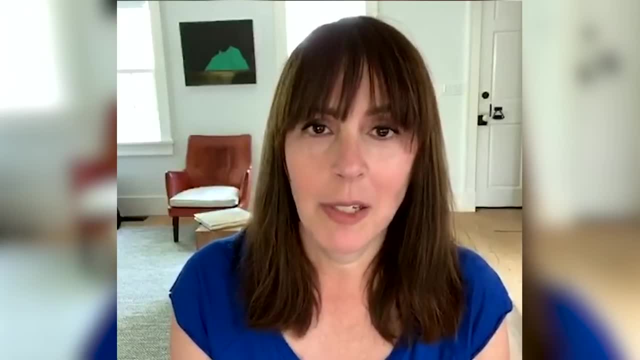 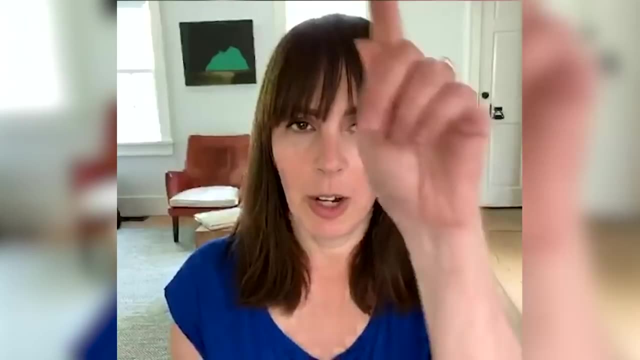 sort of a journaling technique that she likes to start with every day, And I love it so much. So you draw, you take a piece of paper and you draw a quadrant. you draw, you know, a cross, and in the top left, 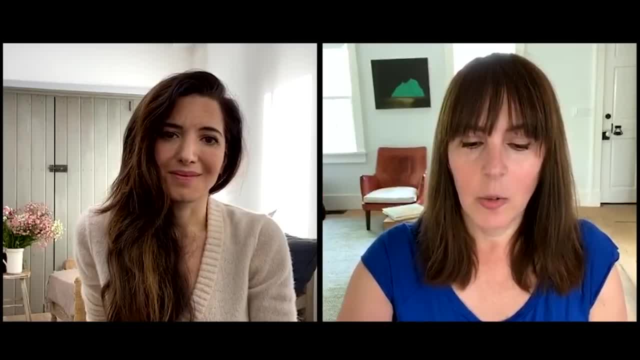 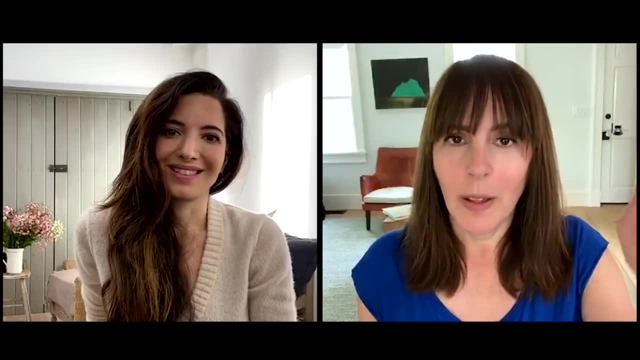 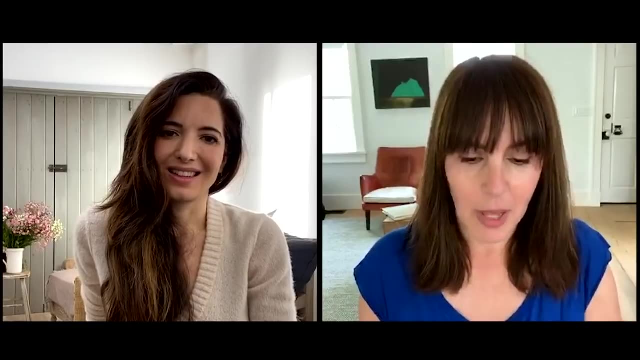 you're going to write did and one and a list, one through seven. Then you will fill these in later. Top right, I saw, and one through seven. bottom left, heard and just one, And then. and then you're going to write doodle on the right. 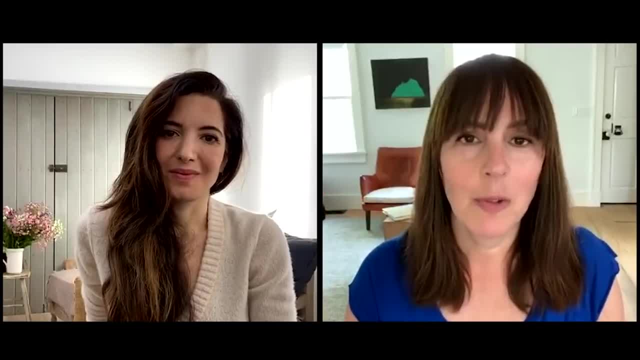 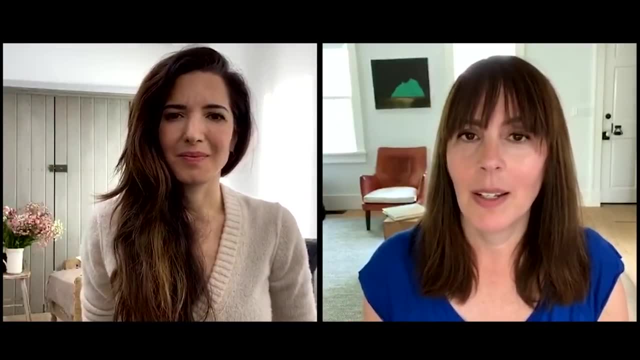 So in the this is going to apply to, like the past 24 hours. on the top left, you're going to write down, just jot down, seven things you did. It might be, you know, dried dishes. It might be eight cashews. 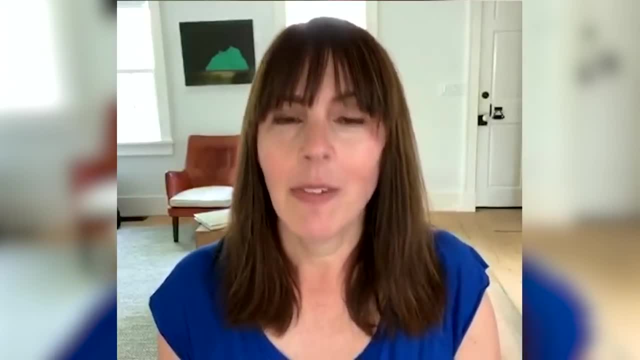 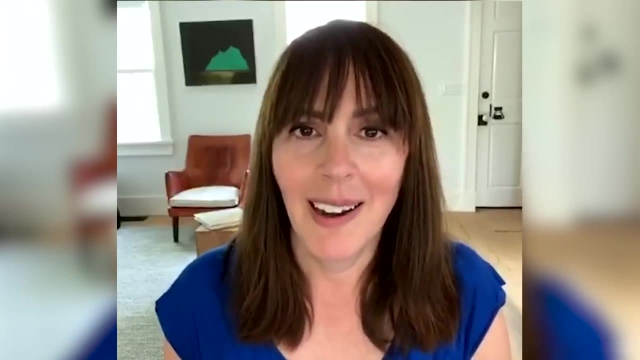 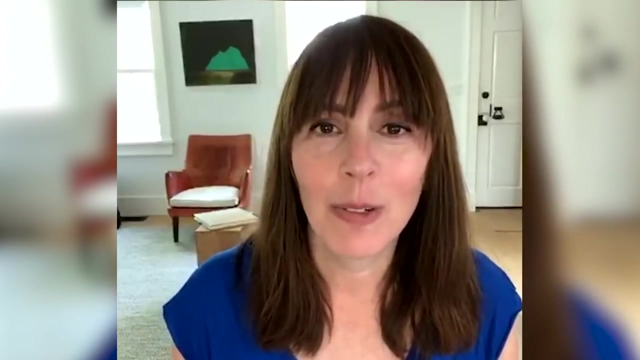 Any little things that you did on the top right, Seven things that you saw, So it might be a bird, It might be my unpainted toenails. I saw those, plenty of things there. And then one thing that you heard, So it might be a line of dialogue you overheard. 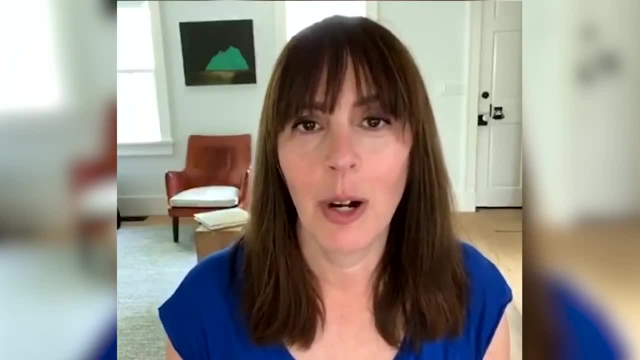 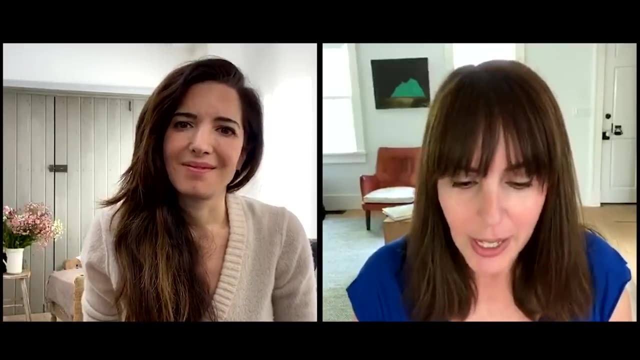 It might be something you heard on the radio. It might be the sound of a frog outside your door. It might be a, you know, the FUD of a package on your doorstep, which I just heard, And then on the bottom right. 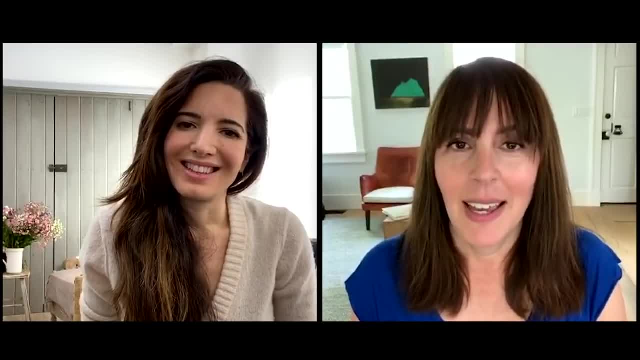 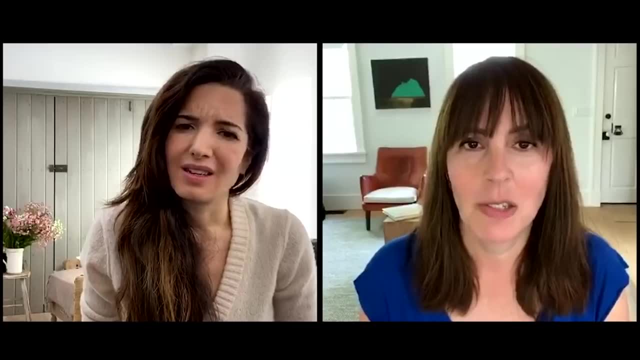 you're going to make a doodle of anything And you can give yourself, say, 10 minutes to do all of these And it's a great exercise. It just it. it lets you go. There's no stress about writing paragraphs or sentences or anything like that. 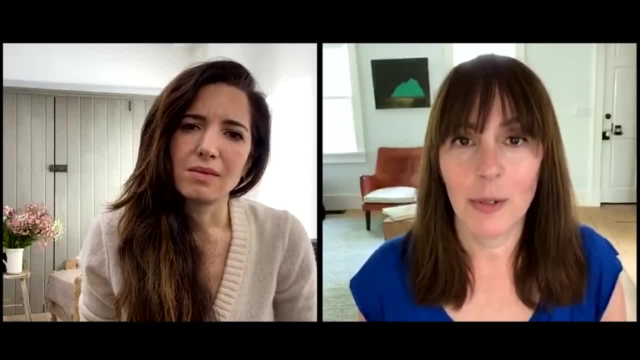 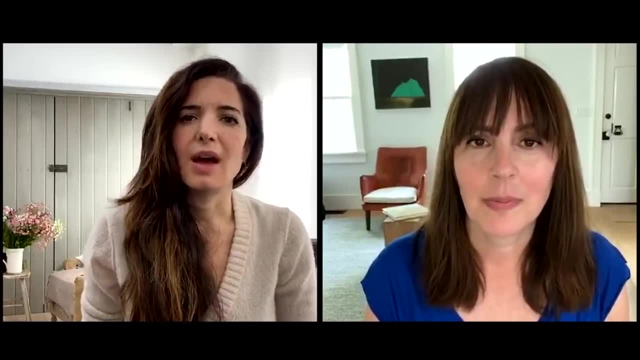 It's just list-making, but it trains you to be observant, to keep track of things that you, to just pick up on little details that you might not notice. Yeah, So I think what I love about that, too is: I think there's so much to be said for just momentum. 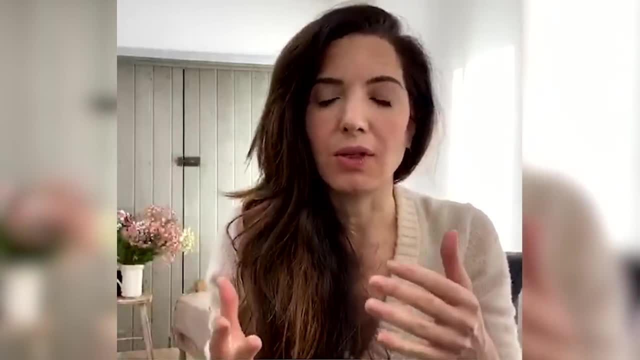 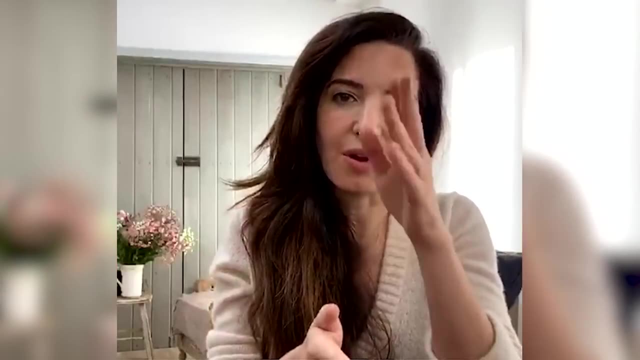 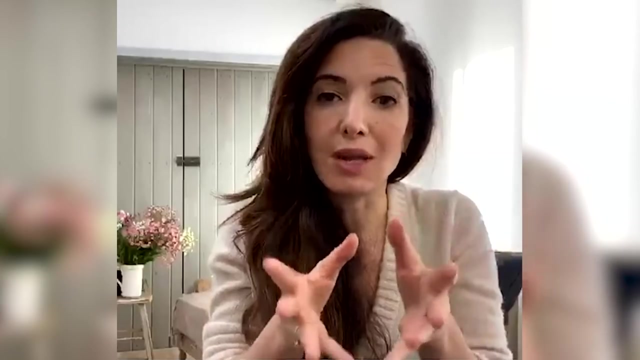 And in our society that's so obsessed with being productive and always producing an outcome, I think that what these prompts and even that incredible matrix describes and helps us do is kind of overcome that constant push to create a final product and just to get ideas flowing. 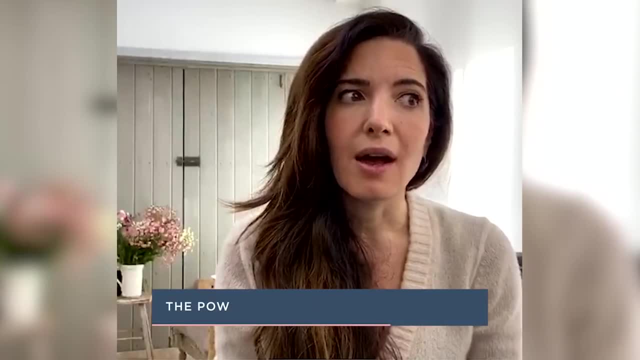 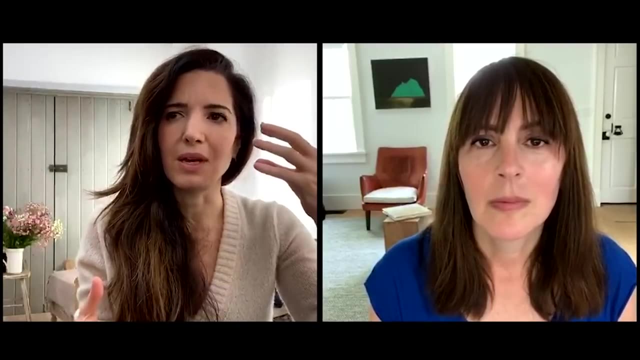 Like the power of momentum is absolutely it's miraculous And if you can give yourself the space to just start making connections and, like you said, develop the skillset of being even more observant, of paying attention to details right And having those kinds of memory captures and putting them down on paper, 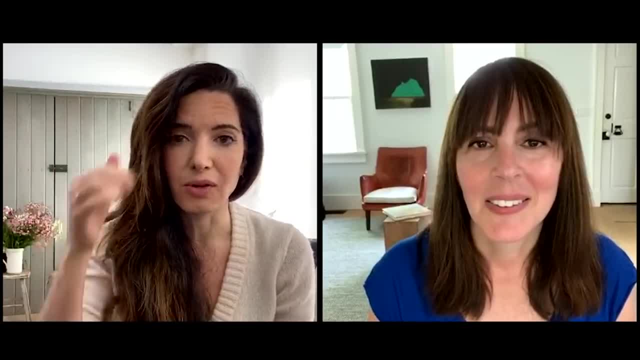 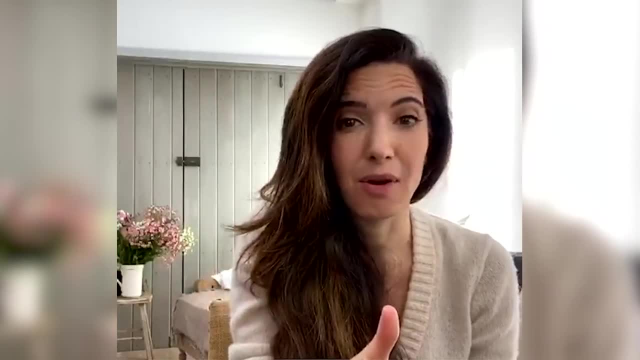 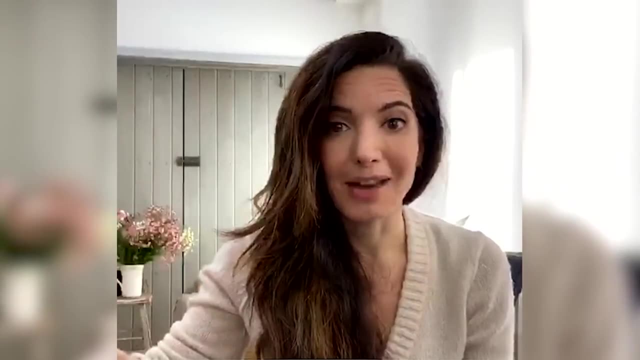 I was looking back at journals that I have just from earlier this year and the emotion that I was talking about like in the end of January, kind of before all of this hit, And I was describing, you know how Josh had this particular bad cough, and now I'm like looking back at all. 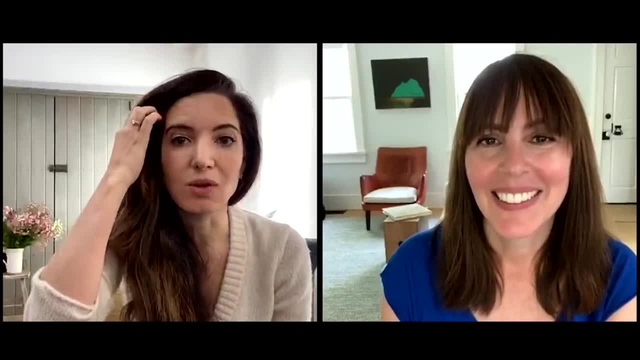 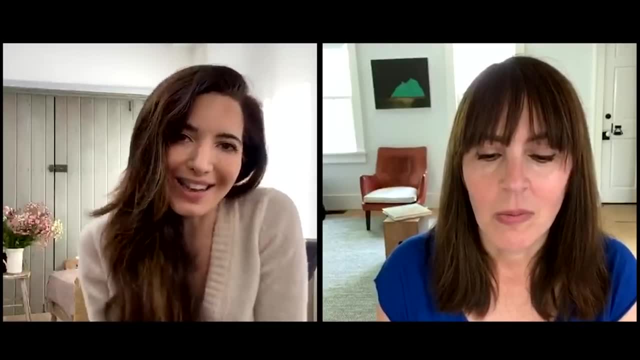 those details, Yeah, And I'm so happy that I was Keeping those journals for this time. So I love these prompts. These are amazing. Anything else that you want to share with people around writing before we wrap up this self-care Saturday: 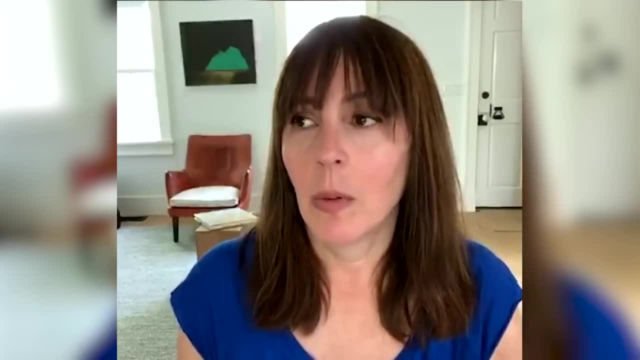 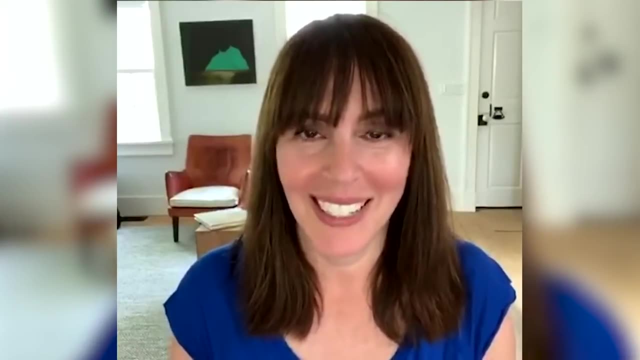 Yeah, I mean, I think that writing is one of the top forms of self-expression. It's definitely the most accessible, portable, affordable, like anyone can do it. It's the thing that we are so excited to learn when we're kids. 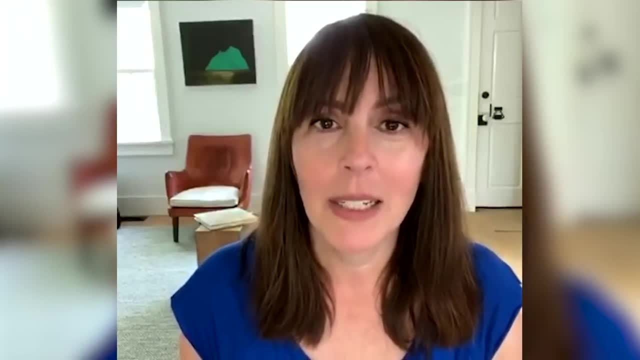 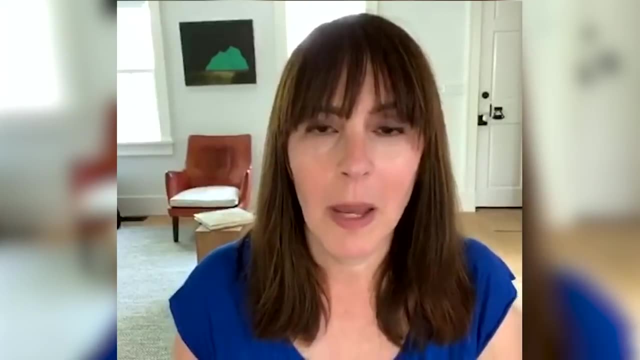 like first grade, like I'm learning to write. I mean it's, I think it's a miracle that it is built into our muscle memory to like create words on the page, whether we're writing longhand or on a keyboard, like that is crazy that we can do that. 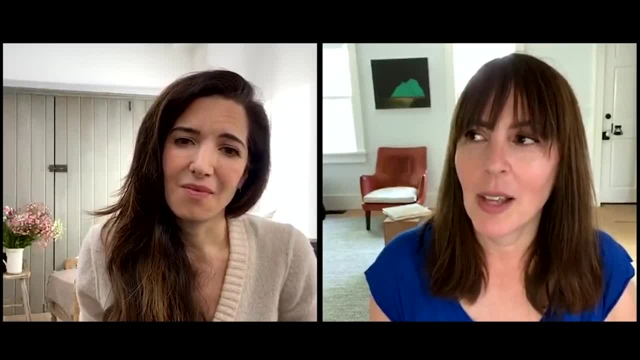 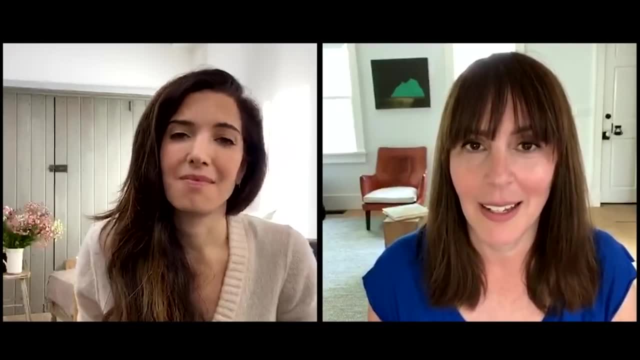 So it's, it's such a gift. And when it comes to self-expression, self-expression is the greatest form to me of self-care, right up there with physical exercise. I'd say they're neck and neck. And when you think about the word expression or express, 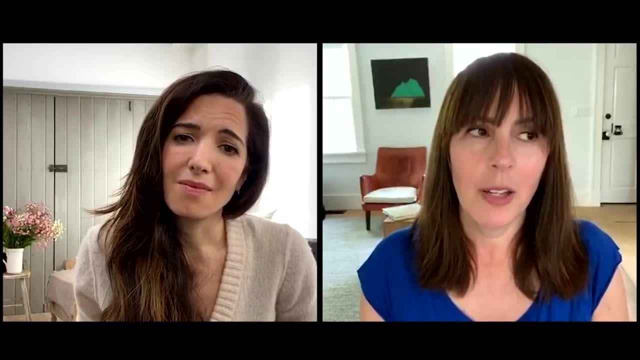 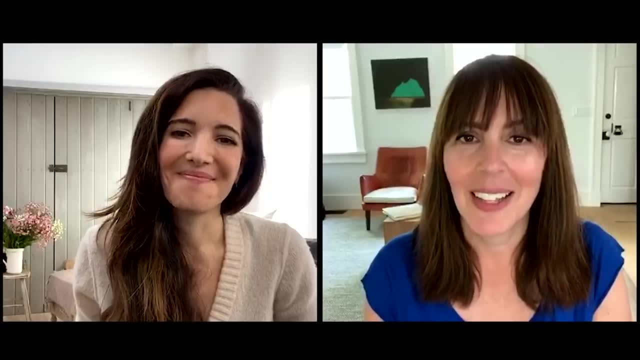 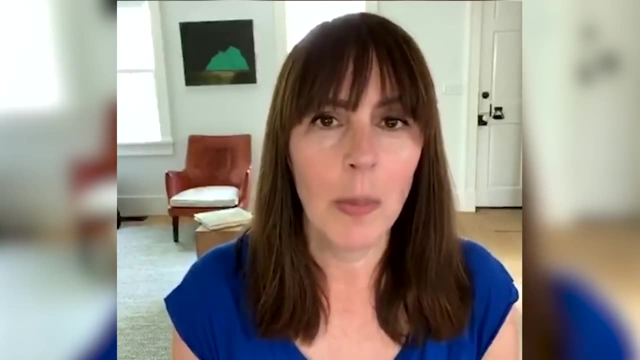 it's not just about communicating, but also about, like another form of that word or another meaning of it. is like squeezing something out, like juice or, you know, breast milk. Neither of us would know, but it is about letting something out, And I think that's so important. 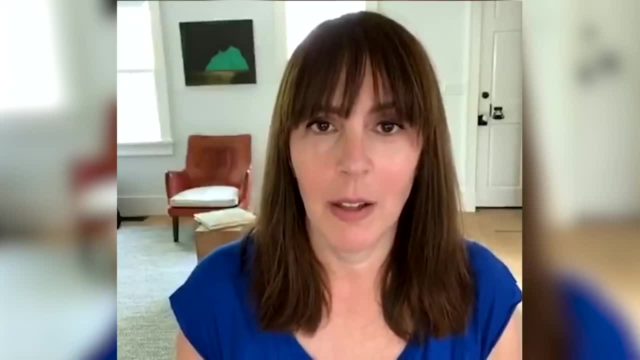 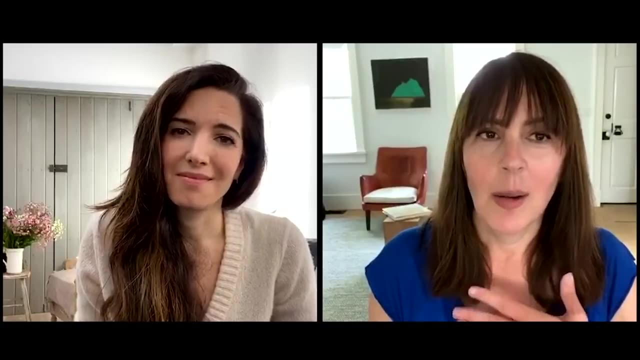 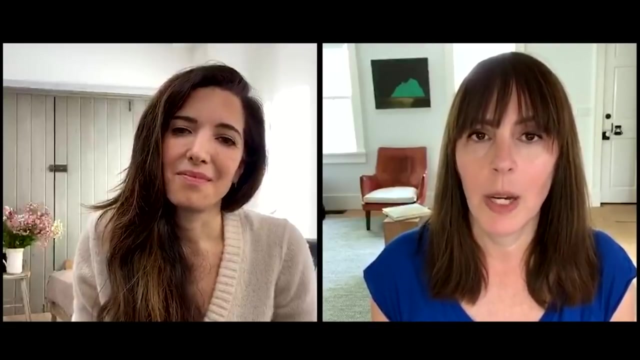 We all have, like those of us who are not in the habit of expressing ourselves in any form, I think, have feel, have a feeling of something trapped inside, And so the best thing that you can do for yourself is is express yourself, And I think that you should use writing to do it. 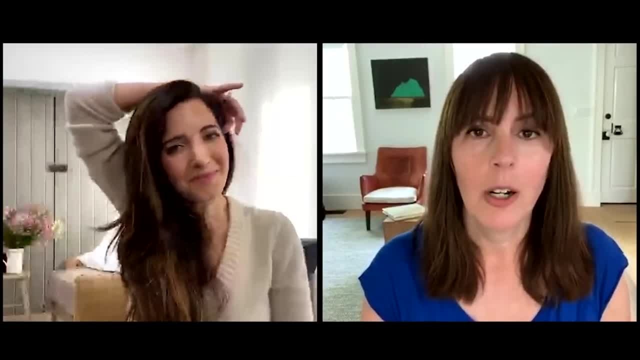 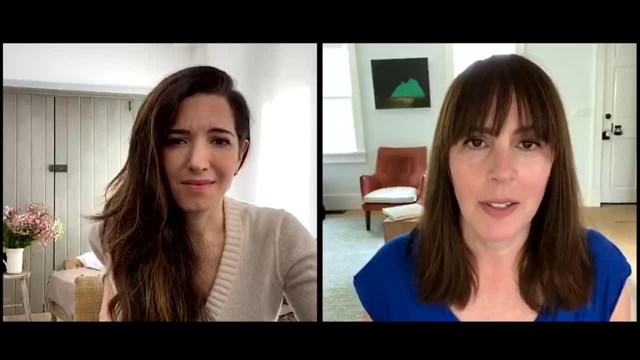 And you don't have to be a professional writer. You don't have to be an author. writing, like to say that writing is only for those people, is like saying that exercise is only for pro athletes. So I think that's something that we should all be doing, and you will be so. 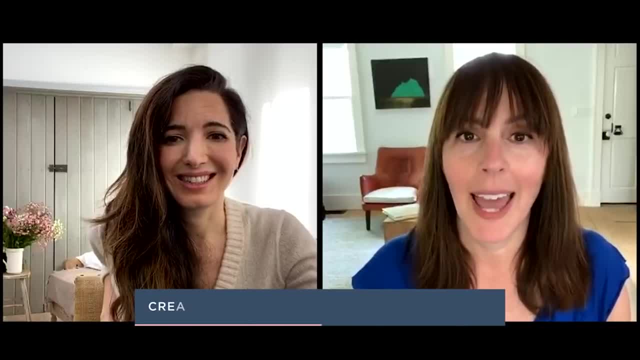 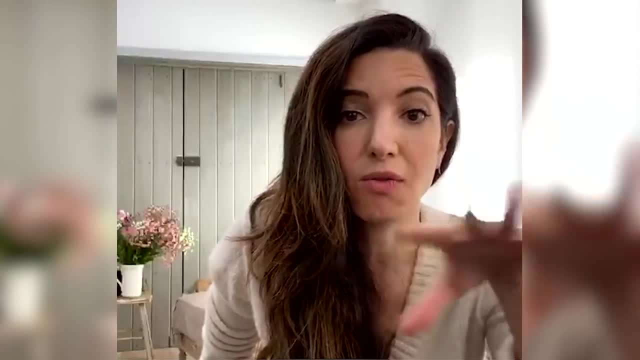 happy with yourself, I think if you create a writing habit and just do it every day. Yeah, Yes, Yeah. I'll tell you it's been transformative for me, even when you know COVID hit and kind of everything started shifting. 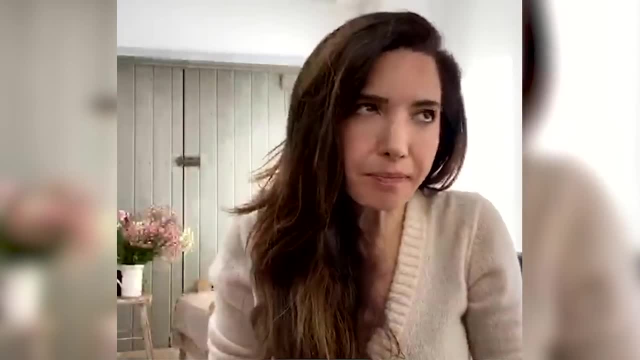 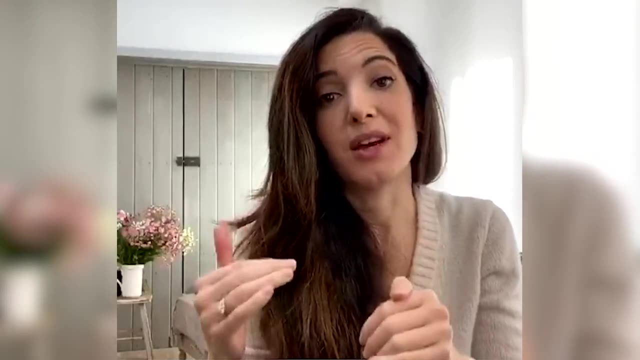 Our lives started shifting and everything had to kind of be rejiggered. I fell out, probably for maybe three to four weeks, of my habit of getting up early in the morning and writing, And that was appropriate, That was fine. It was like. 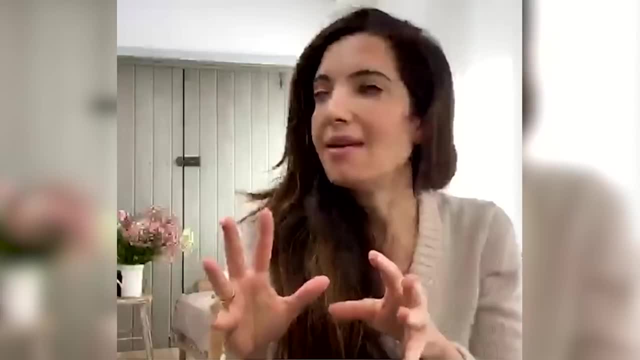 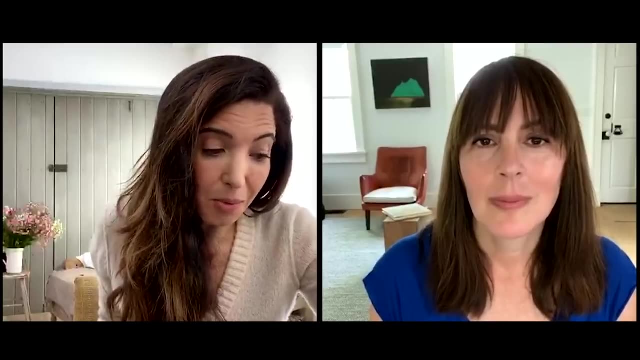 there was so much happening, There was so much that needed to shift that for me. I had to say, okay, I'm going to prioritize a little bit more sleep right now. I wanted to really take care of my health And then, a couple of weeks ago, 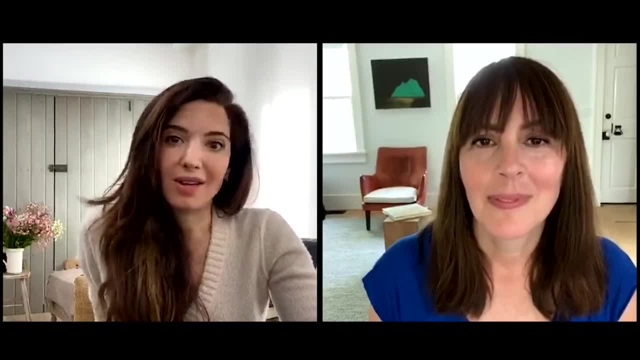 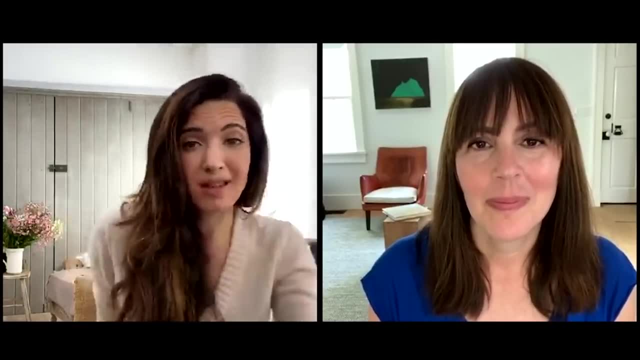 I restarted that habit again of waking up super early and just going and writing on the page. You know, sometimes it'll be two hours, Sometimes it'll be 30 minutes. You know it depends on, again, what's happening in the flow. 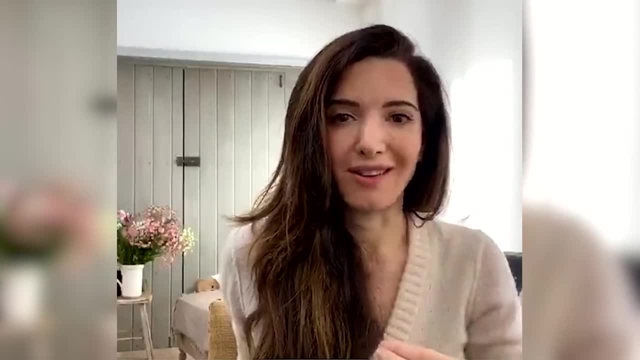 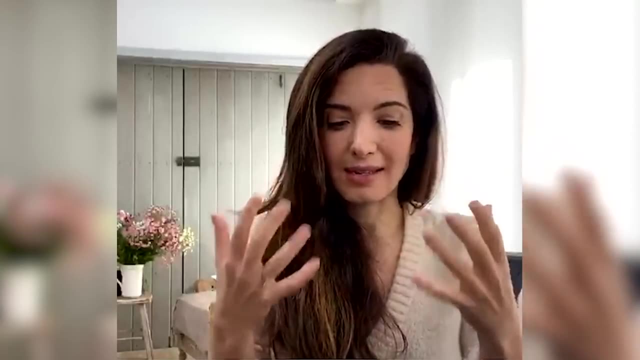 but I could not agree with you more. I feel so good when I have spent time on the page, when, even if it is just 20 minutes of sharing and getting down more thoughts and more ideas and putting them on paper and moving that ball a little bit ahead. 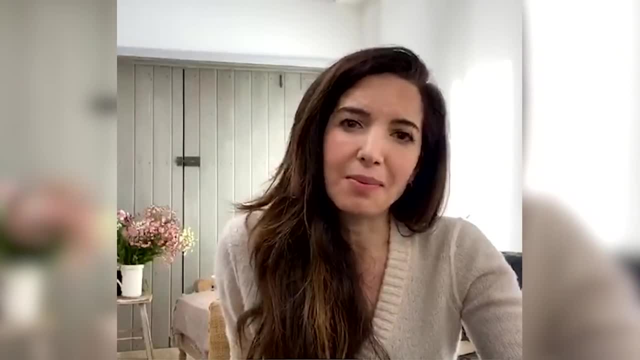 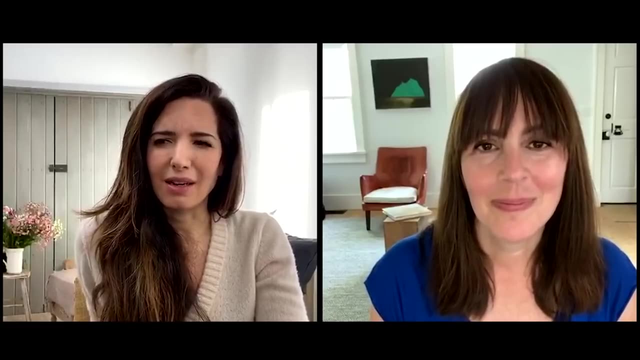 I just feel this sense of groundedness And the sense of fulfillment and satisfaction, that I can notice a difference if I miss a day, and I can notice a difference of feeling like, ah, like I didn't have that little pocket of time to. 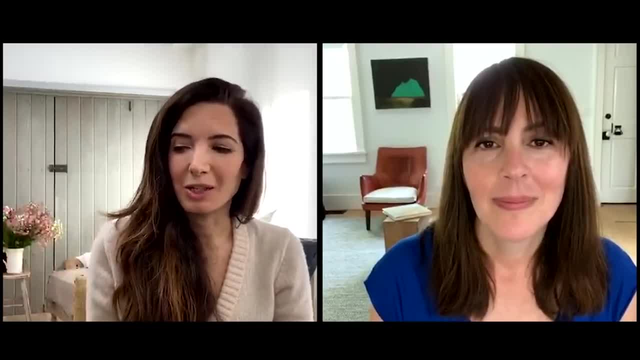 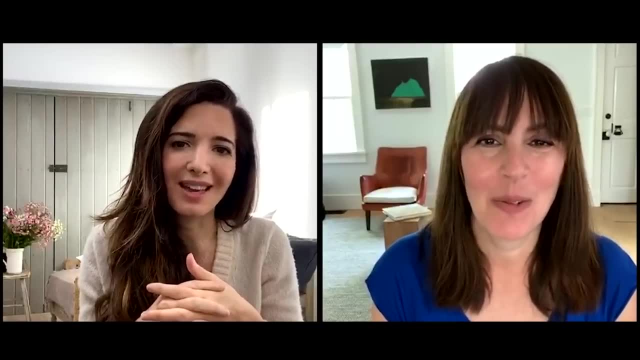 to really spend time between me and me, and I'm expressing myself. So, Laura, you are so brilliant. I'm so grateful for our friendship. My goodness, Me too, Thank you. Thank you so much for hanging out with me today, Oh. 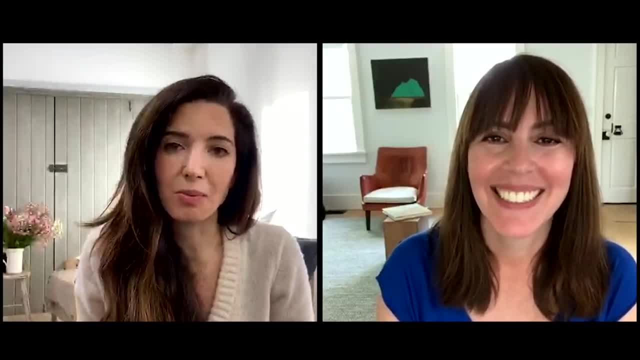 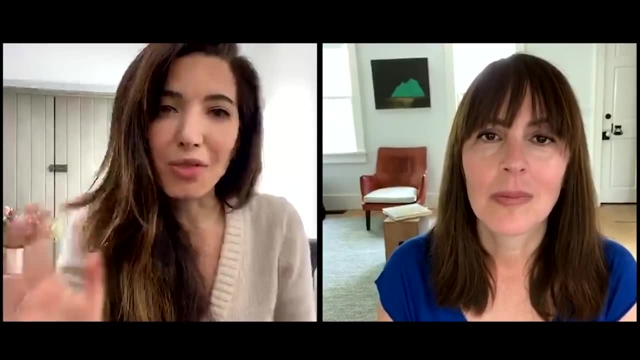 thank you for hanging out with us, Yeah, And thanks for taking the time to put all of those prompts together and for all You guys that have been with us for this self-care Saturday writer's edition. Thank you, Thank you, Thank you. 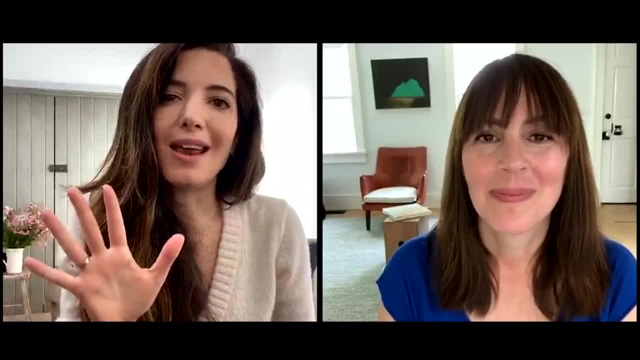 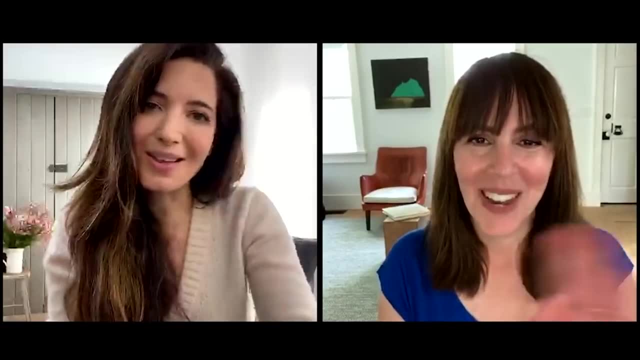 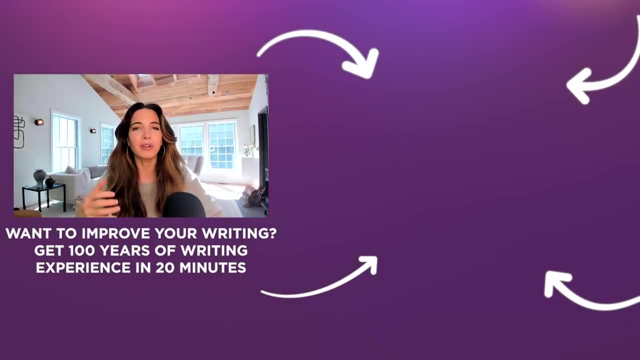 Again, you can rewatch to get all of the prompts and, in the meantime, take really good care of yourselves and each other, And we will see you soon. Bye Laura, Bye everyone, Bye everyone. Are you someone who aspires to become a better or more prolific writer? 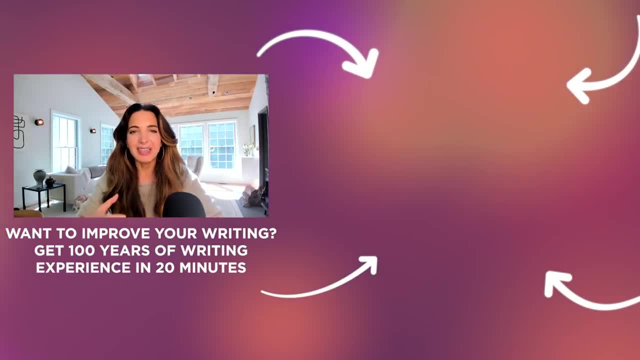 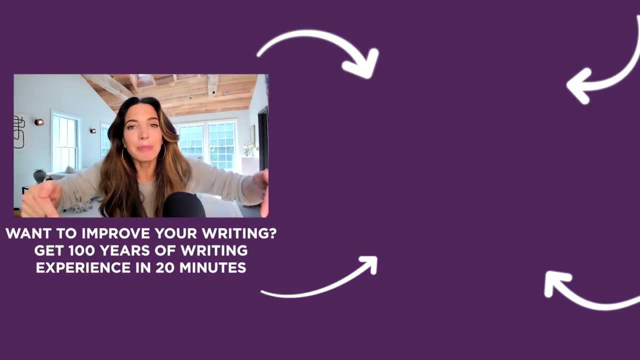 Maybe you want to get your book done. Maybe it's a program, Maybe it's a screenplay, something like that. If writing Is a part of your practice, you'd like it to be, or you want to get better. This is the episode for you.